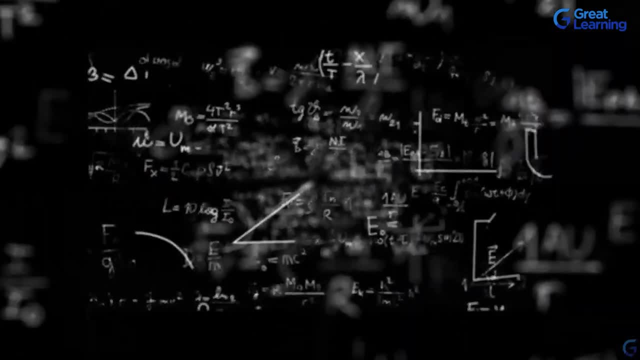 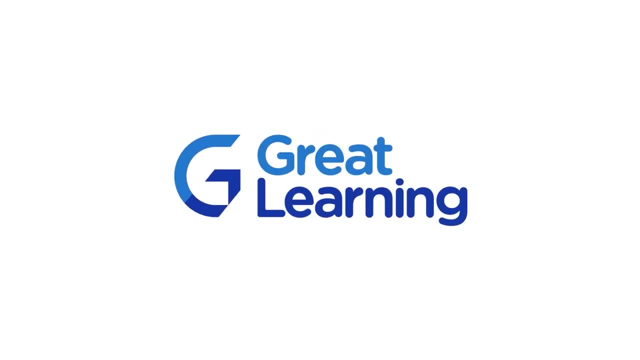 structure algorithms like Varsha's and Truksha's algorithm. So if you are interested in knowing more about graph theory, then welcome to this course. If you haven't subscribed to our channel yet, I want to request you to hit the subscribe button. 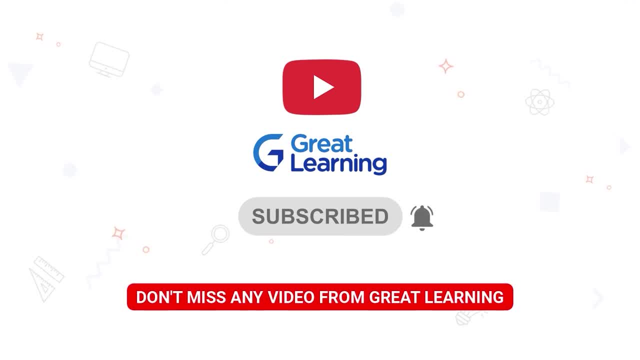 and turn on the notification bell so that you don't miss out on any new update or video releases from Great Learning. If you enjoyed this video, show us some love and like this video. Knowledge increases by sharing, so make sure you share this video. 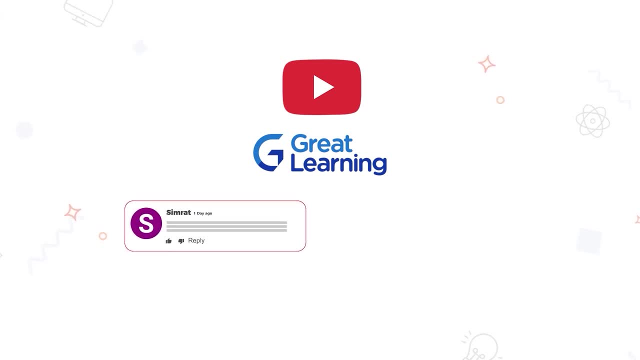 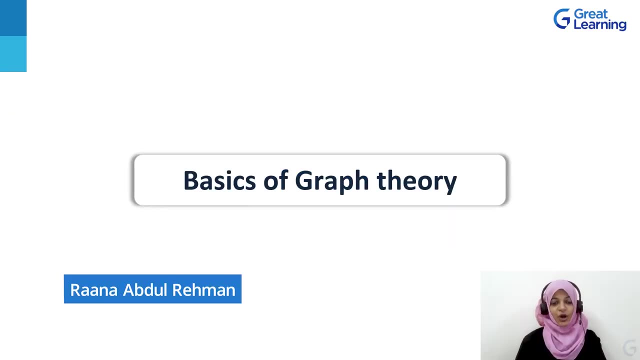 with your friends and colleagues. Make sure to comment on the video for any questions you may have. If you have any questions, feel free to ask them in the comments below and I will respond to your comments. Hello everyone, and welcome to this new course on graph theory. 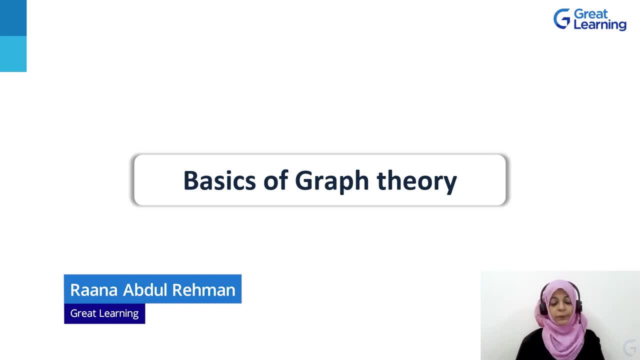 Now, in this particular course, we are going to understand what are the basic concepts of graph theory and we are going to understand how they can be implemented in various ways. So let's quickly get started. So, in this particular course, we are going to understand: 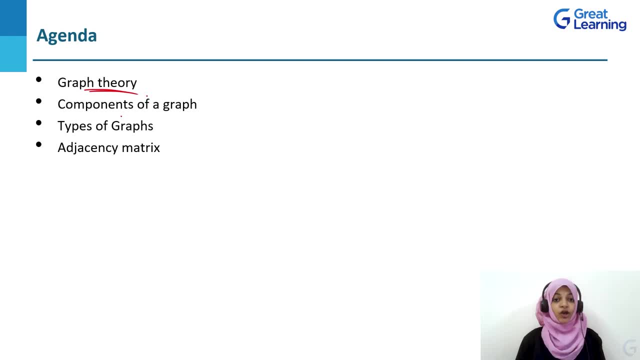 what are the basic elements in graph theory, what are the components of a graph, what are the various types of graphs? So there will be various graphs that we will normally be seeing in graph theory, and we are going to discuss them all in detail here. We'll also be looking at why these graphs 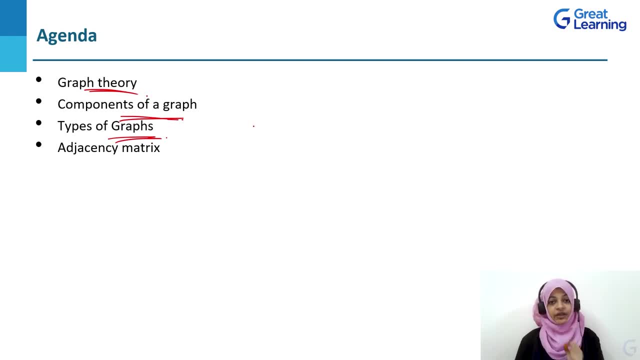 are different from each other, So the minute characteristics of the various graphs will also be identified and discussed here. Lastly, we're going to look at a concept of adjacency matrix and understand exactly how and why adjacency matrix is utilized. So let's quickly dive into the course. 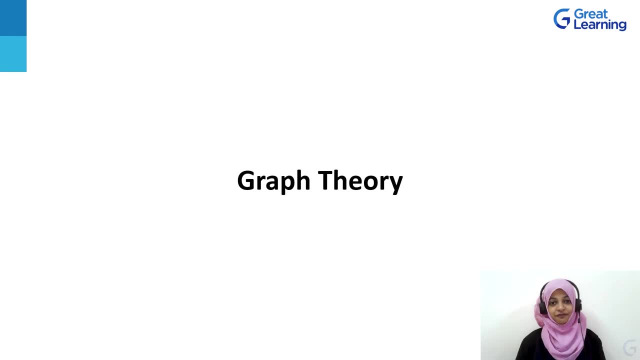 So first we're going to look at the concept of graph theory. Now, in graph theory, we first need to understand what it is, and we also need to look at what are the applications that we actually have in real life, as well as in computer science. Why do we need to do these things? Because it 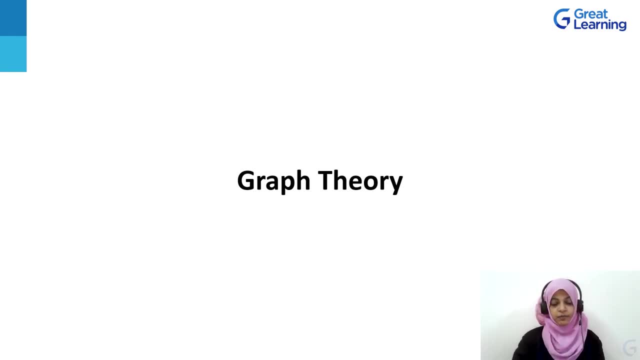 will help us understand exactly why we are studying this particular subject, right? So let's quickly get started. So the first thing that we need to understand is that, in graph theory, the basic concept that we have is of graphs, right? So what are graphs? Graphs are actually. 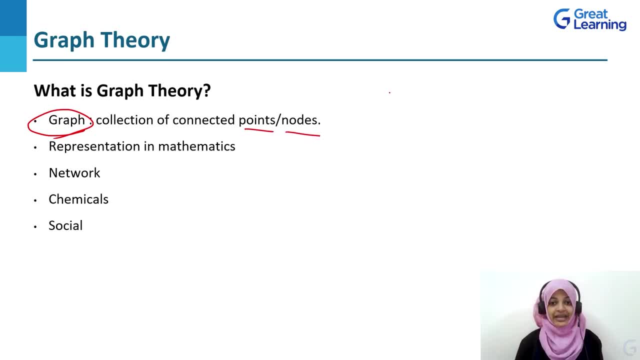 a collection of points or nodes. So, as I've already stated, there are some elements in a graph. right Now, these elements are known as points, or more commonly called nodes in a graph. So node or point is a technical term and elements is just a colloquial term. right Now, these elements or these 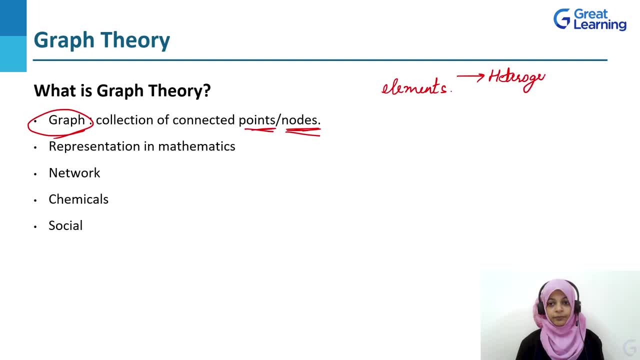 elements can either be heterogeneous in nature, or they could be homogeneous in nature. Now, what does this mean? This means that the two elements, or more than two elements, which are connected with each other and forming the graph, may either be of the same type or of different. 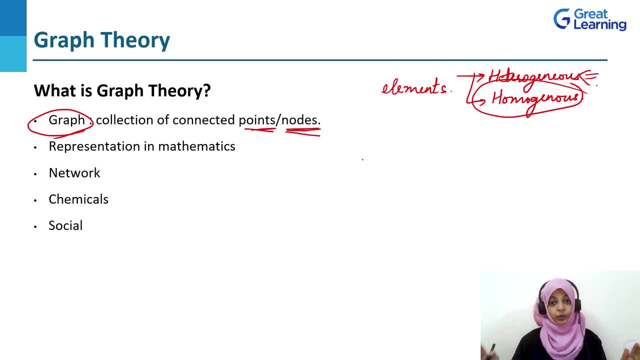 types. So we can have, say, for example, two humans communicating with each other. This would make the two nodes homogeneous in nature. On the other hand, if the communication is between a human and a digital device, say for example a mobile phone, then this particular communication or 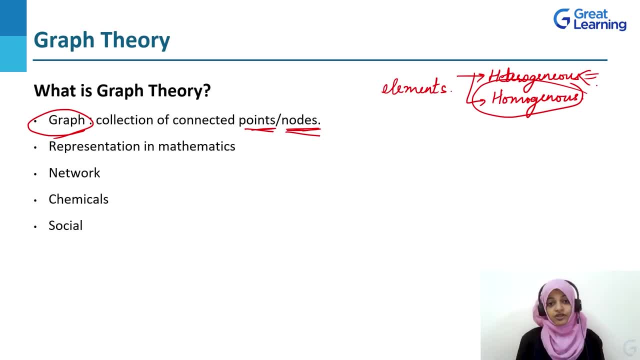 the nodes in this particular graph will actually be heterogeneous in nature because both the elements or both the nodes in the graph are actually not of the same type, right? Next, we need to understand that graphs are actually a mathematical representation. Now, any kind of communication or any kind of connection that is actually seen between any 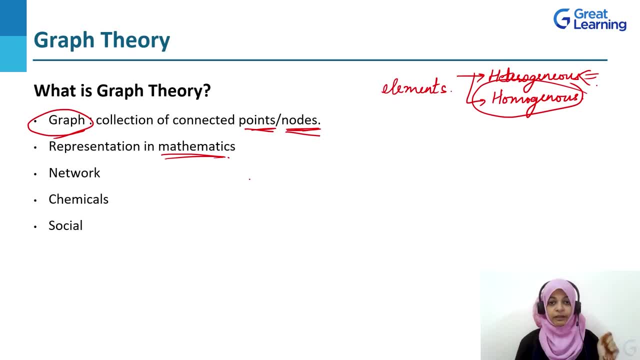 node can be represented in mathematics with the help of graph. Now, graphs can be of various types. You could have graphs that you can normally see. You can have graphs that are like trees. You can have those trees divided into binary and non-binary trees, and so on and so forth. But one thing we need: 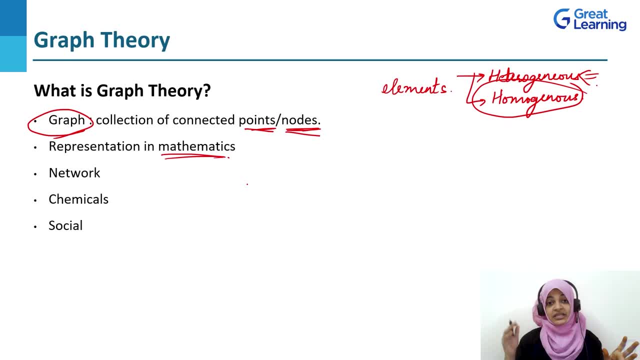 to understand very clearly is that if you have nodes and there is a connection between those nodes, it is amply obvious that it can be mathematically represented as a graph. Now, some of the most commonly seen graphs are in the form of networks, chemicals and even social interactions. So 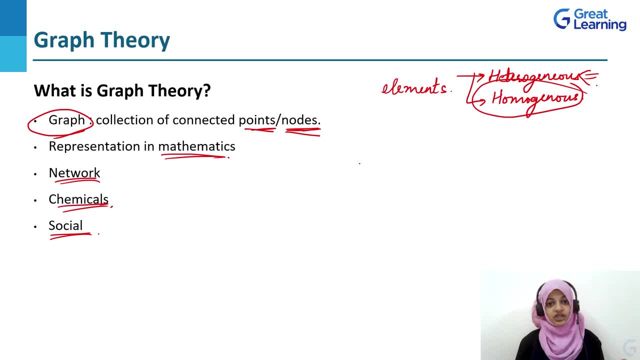 networks, as we already know, are actually the connections between various nodes, wherein the nodes would be either humans or other kinds of communication devices. right So if we have humans connected to some mobile devices? right So if we have humans connected to some mobile. 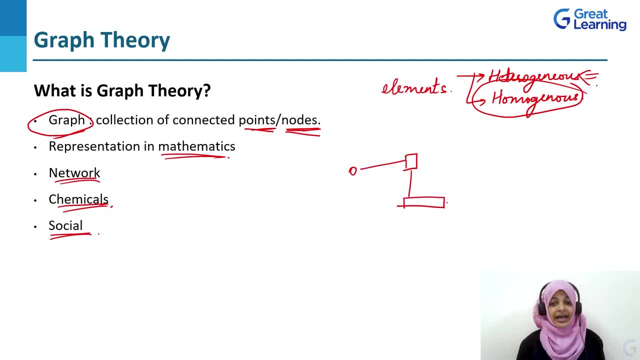 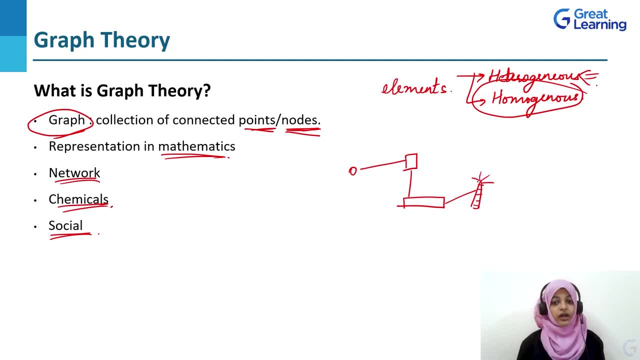 to a tower, say, for example, then this particular depiction would also be a graph right Now, why is this a graph? Because here we've got various nodes or elements which are connected to each other, So this kind of a network can also be represented as a graph. Next, let us 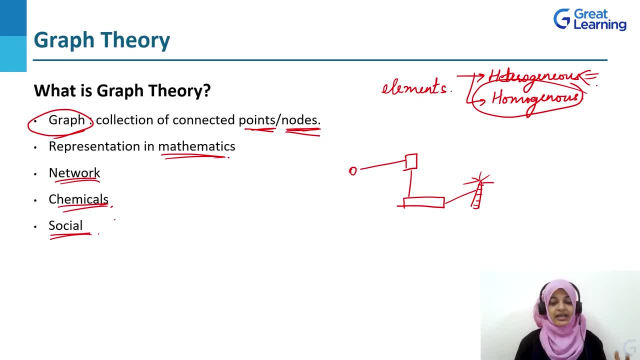 look at an example of chemicals. We've seen various chemicals as we have studied in lower classes right. All of these chemicals are actually depicted using some diagrammatic representation. So, for example, if we look at H2O, H2O is often represented as H O H. So 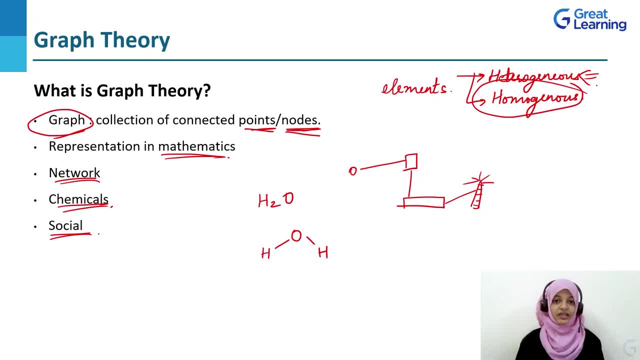 here we can see that we've got three atoms which are actually connected to each other in such a manner that it is forming one molecule. So there is some interaction between these various nodes. So thus we can say the diagrammatic representation of any 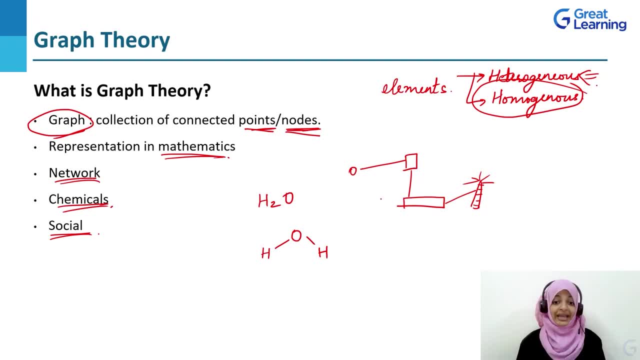 kind of chemical is actually a depiction of a graph. Another example that I can give you here is CCl4, right Carbon with four chlorines. This is depicted in this particular manner: We have a carbon in between with four chlorine atoms around it. Again, as you can see, 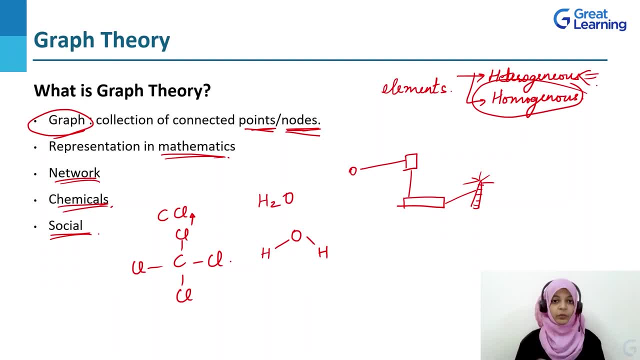 we have five nodes and all of these nodes are interacting with each other in such a manner that you are able to form a graph of this particular interaction. Lastly, we've got social interactions represented as graphs, Any kind of social interaction, whether they are entertainment-based interactions or they are communication-based interactions. 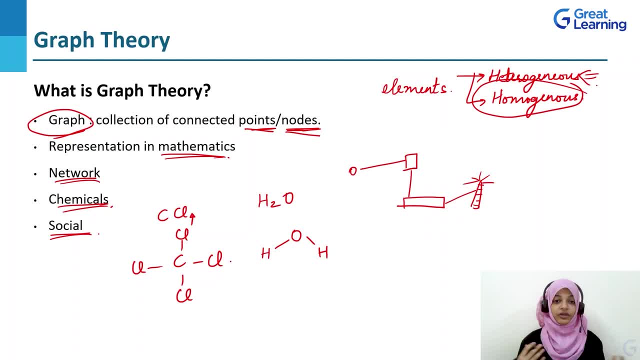 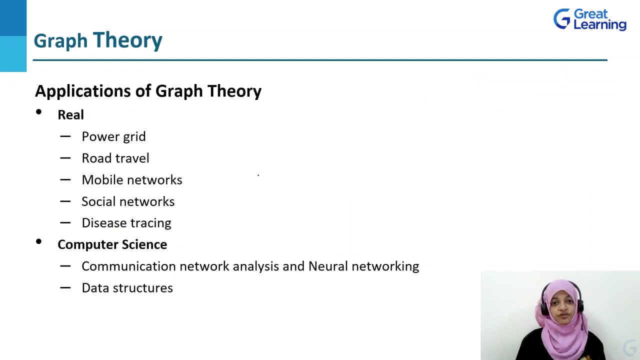 can actually be referred to in the form of graphs, right? So any diagrammatic representation that you want to create, such that it shows the interaction between various nodes and this is represented in a mathematical manner, then that particular diagrammatic representation can be known as a graph. Next, let us look at some applications of graph theory. 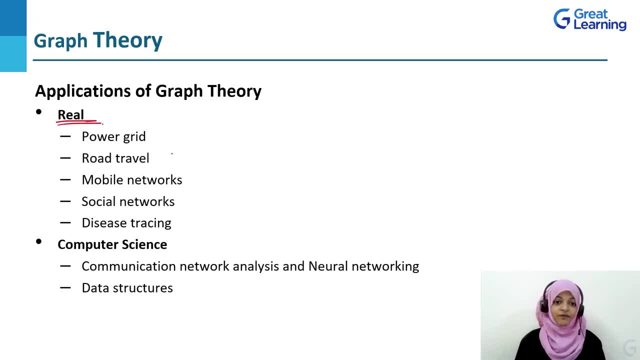 So first we look at some real-life applications. Now, as we've already seen, any kind of interaction would become a part of a graph or would be diagrammatically represented as a graph. So this means that if we've got the interaction between these nodes, we can say that the diagrammatic 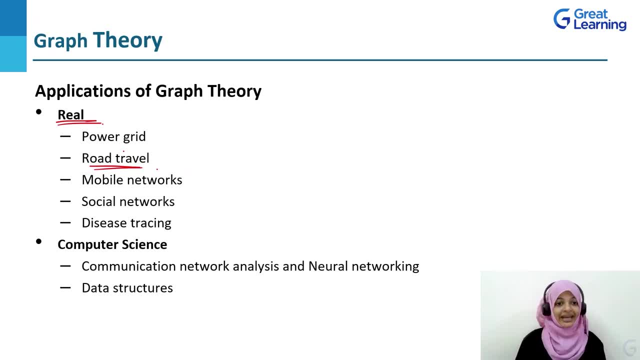 representation is represented as an interaction between a start and an endpoint, or an interaction between one tower to the next, or an interaction between two or more mobile phones, or an interaction between humans, either via their social networking sites or via contact disease. In each of these cases, you can see that there are some interactions that are going on, and all of these interactions- 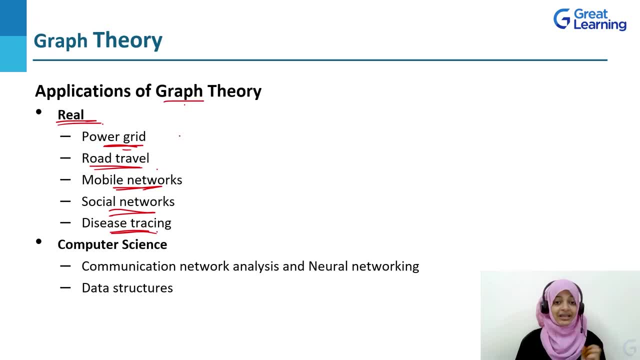 can be depicted using graphs In Power Grids. graph actually helps us determine where a step up or step down transformer has to be attached in order to maintain the voltage of any current that is moving from one point to the next. Power grid analysis using graph theory also. 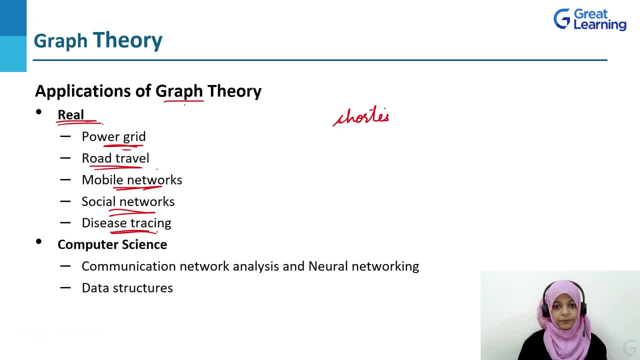 helps us determine the shortest and most efficient route that needs to be taken in order to transport electricity from point A to point B. In a similar manner, if someone is undertaking road travel, an analysis of the whole graph of roads- or, in this case, we could also call it a map of roads- 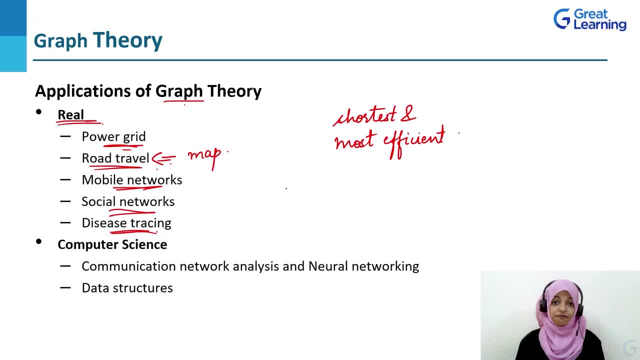 would actually help us determine the shortest, most efficient and fastest way to reach from point A to point B In mobile networking sites. again, as in power grids, we can use graph theory concepts in order to determine and analyze exactly where the power grid is located, Where a cell tower has to be placed in order to ensure maximum area coverage for that particular. 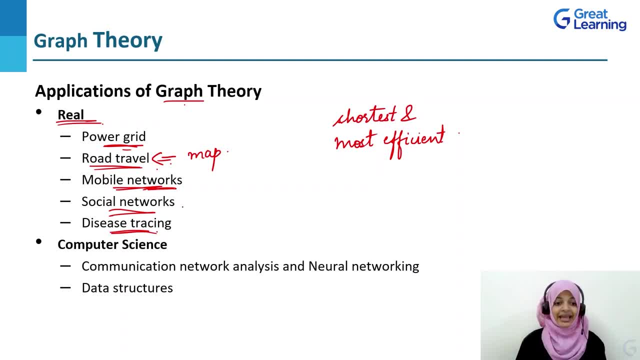 network provider. Next, social networking analysis will actually help us determine how humans are interacting with each other. how far are they interacting with each other, how much and how frequently do they interact with each other? Apart from that, social networking analysis also helps us determine what is the most. 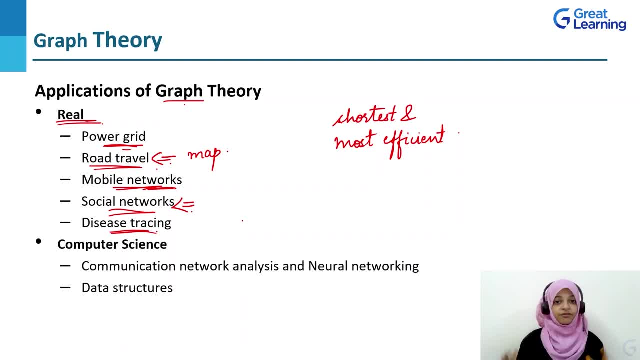 common and most efficient route to reach from point A to point B. In a similar manner, if someone is undertaking road trips and a map of the roads from point A to point B where they haveography at the start of the crop, towards the end of the crop stores, how far is there going to be? 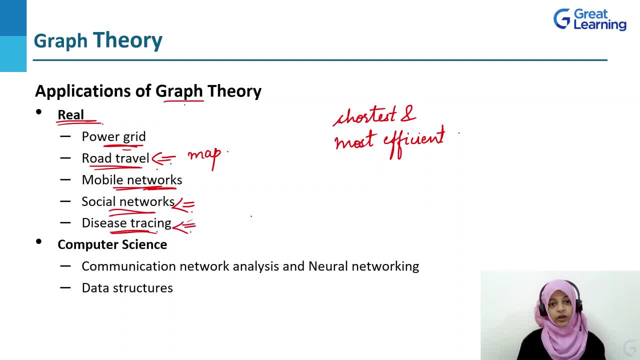 average tidak hit price of sleep and what is the bridge ratio for camps location? Since these are common laughing terms, you can also slightly DIAL DIALпIN times as you draw. tried and Seven Times App are the best methods to know where your rolling, though, and where are you talking to, and try to find the way you want. 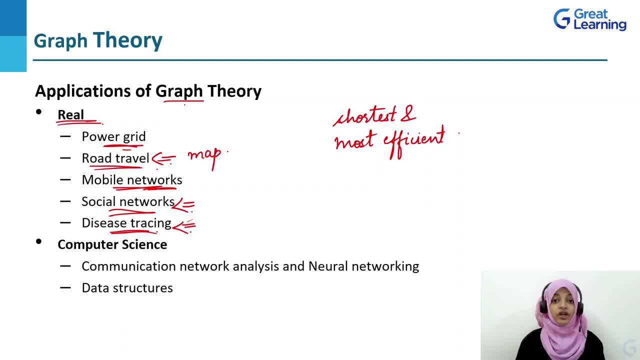 with each other. this helps us actually analyze and contract trace the disease and help us estimate the actual dangerousness of any kind of disease. right, so these were the real life applications of graph theory. let us look at the computer science applications of graph theory. computer science applications are most commonly seen in network analysis, where we are actually talking. 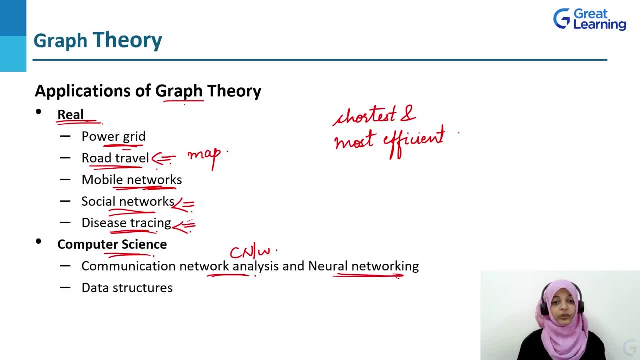 about computer networks and also in neural networks. so while we are actually trying to build a neural network, the first point of instance that we actually take care of is analyzing whether a particular neural network is feasible or not by applying graph theory concepts. next, we also see various graph theory concepts in data structures. so in data structures, whenever you have any. 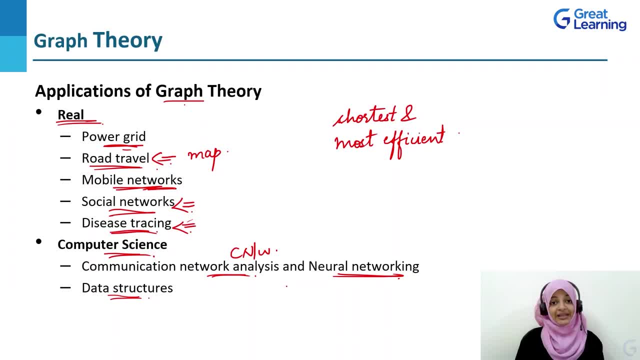 concepts related to cruscals, warshels spanning trees, etc. these are actually basic graph theory concepts that have been extrapolated and implemented onto data structures such that these graph theory concepts can actually fit into a computer programmable manner. so these are how graph theory concepts can actually be applicable in the real world, as well as in. 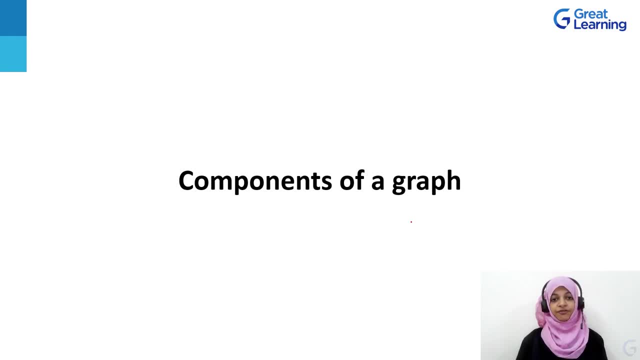 computer science. next, let us look at the components that are part of any graph. now please remember that these components are important to understand because they form the basis of any and all Git-like systems graphs that we might come into contact with. so the first thing we need to 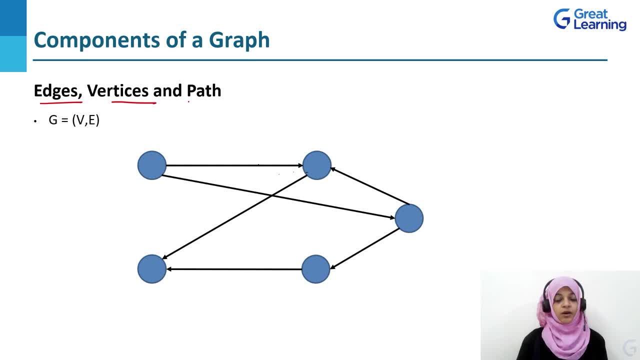 understand here is: what are edges, what are vertices and what is a path? assume we have this kind of a graph, as given here. in this graph we've got various blue circles. these blue circles are actually our nodes. these nodes are known as vertices, right, so these vertices are actually named vertices. they can be. 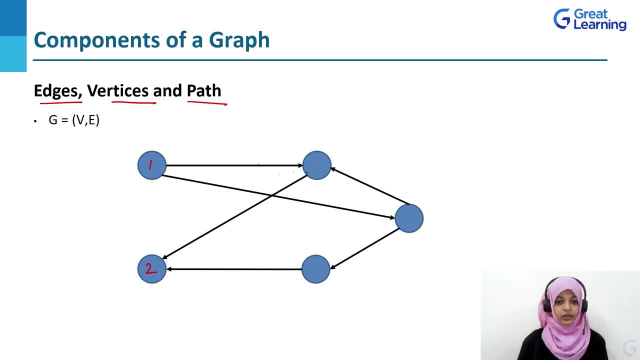 named as numerics, as 1, 2, 3, 4, 5, or they can also be named alphabetically, like a, b, c, d and e. the naming conventions for the nodes are up to you. we can also have a combination of alphabets and numerals, such as a1, a2, a3, a4, a5,. 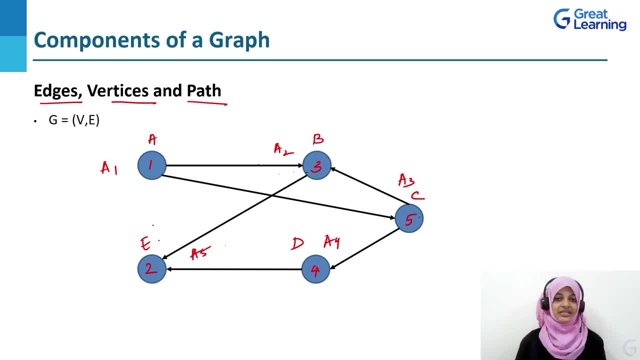 and so on and so forth. So, as you can see, we can name our nodes as and how we require, and these nodes are known as vertices. So, if we look at this particular diagram, I have named all of the vertices here as numerals, because that was easiest for me, right? Let us next understand what edges 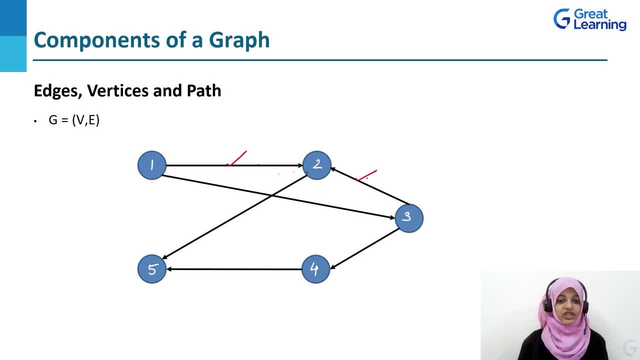 are. Edges are actually the connecting lines which exist between any two nodes of a graph. As you can see, these lines are such that they always connect two nodes or two vertices within the graph. Please note that any one edge will always only exist between two vertices. You can't. 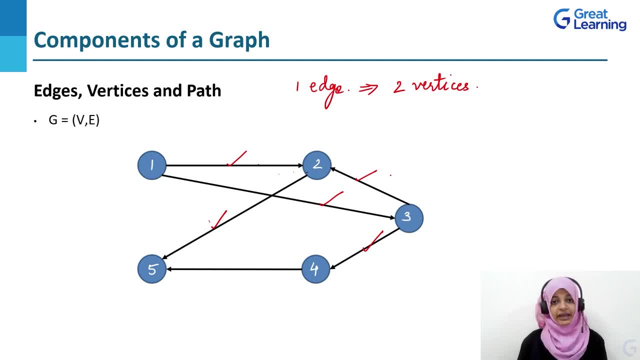 have one edge, going through three vertices at the same time. This is some very important concept, as we'll see further on. Now. here we can see that there is an interaction between node 1 or vertex 1 and vertex 2.. This particular interaction has an arrow given here. Now what? 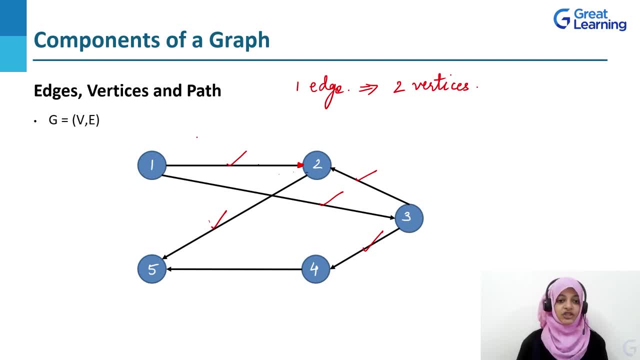 does this arrow mean? This means that this particular interaction is going from vertex 1 to vertex 2.. So in edges we actually have two types of edges. We've got directed edges and we've got non-directed edges. Directed edges are those that actually have arrows. 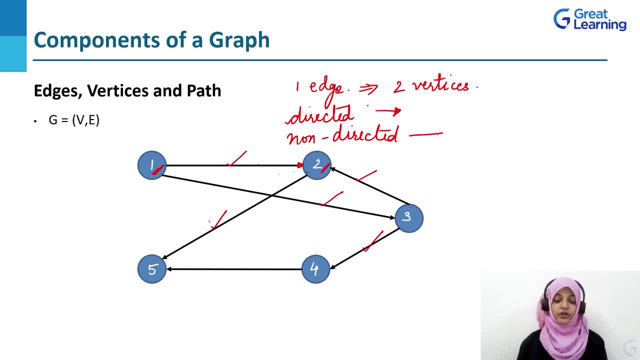 And non-directed edges are those which have no arrows between them, right. So because of this, we will see that there are two types of graphs too. Let us now concentrate on what a path is. A path is very simple. A path is actually the set of vertices that have to be jumped through in order. 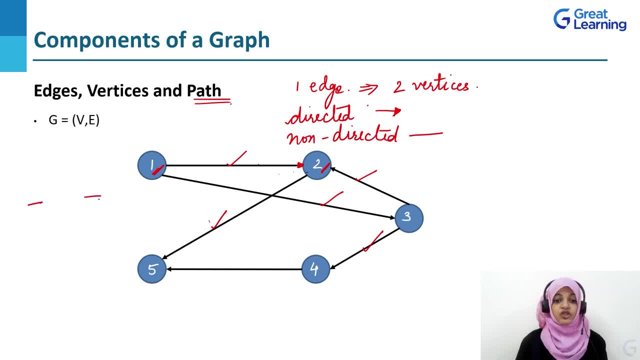 to reach from one vertex to another. So if we want to move from vertex 1 to vertex 5, we can see that there is no direct path from vertex 1 to vertex 5.. So we need to take a path through the other vertices which are there in between in order to reach vertex 5, right? So let us? 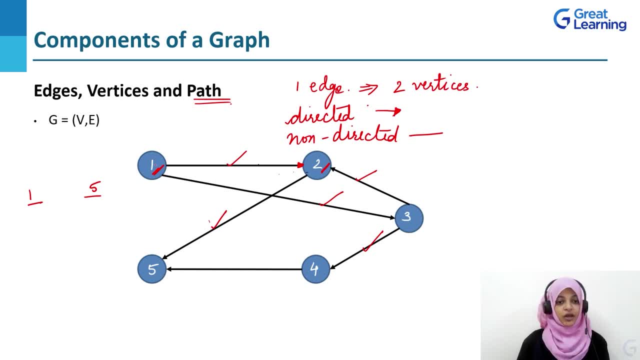 see what path can be taken. We can see that vertex 1 goes to vertex 2 and vertex 2 can go to vertex 5. So we have one path here: vertex 1 to 2 and then from 2 to 5.. Similarly, we 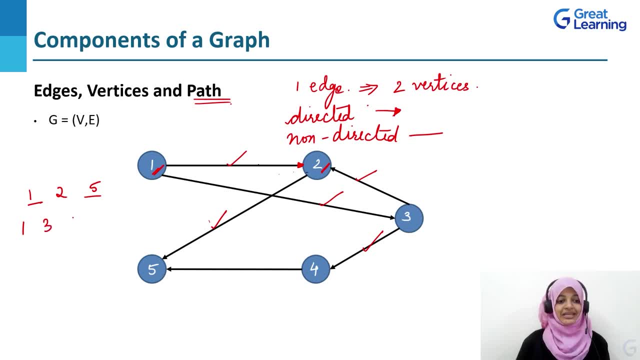 can go from vertex 1 to vertex 3.. From vertex 3 to vertex 4 and from vertex 4 to vertex 5.. This is another path, So in order to go from one particular vertex to another, a graph may have multiple possible paths. Each. 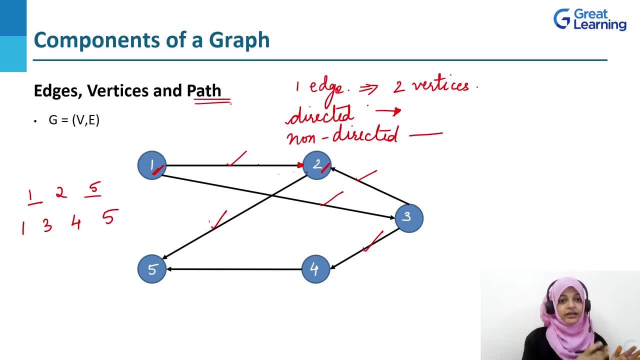 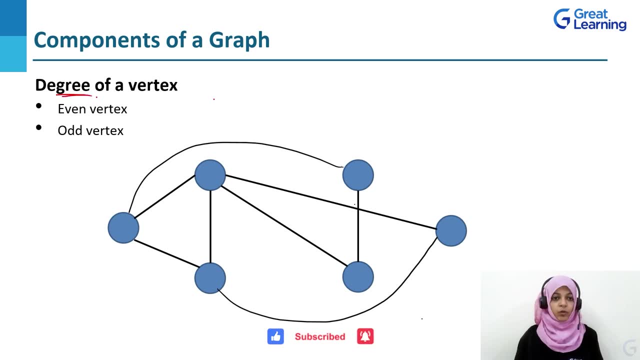 and every path is such that it will take you from the intended vertex to the destination vertex. Next, let's look at the concept of degree of a vertex. Now, what is the degree of a vertex? It is actually the number of edges Which are incident on a particular vertex, Right? so for each and every vertex, we would 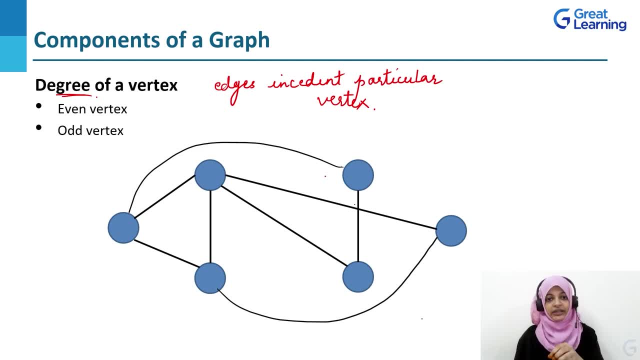 have a different number of edges that would be incident on it, and that particular value becomes the degree of a vertex. Now the number of edges that are incident on a vertex may either be even in number or odd in number. So, based upon the number of, 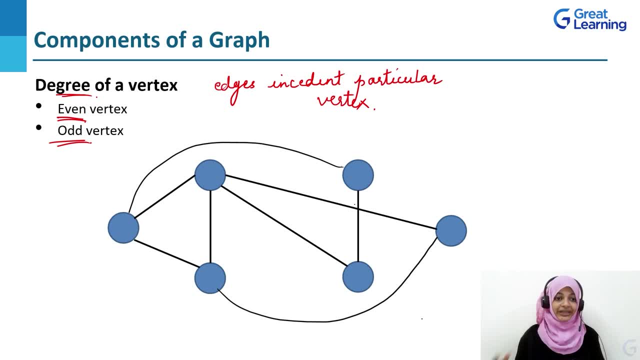 edges on a particular vertex. we can say that the vertex is either even or an odd vertex, So this is not a defining factor of a vertex. it is just a manner of denoting how many edges are actually incident on that particular vertex, right? So if this is my particular graph, this means that I've got 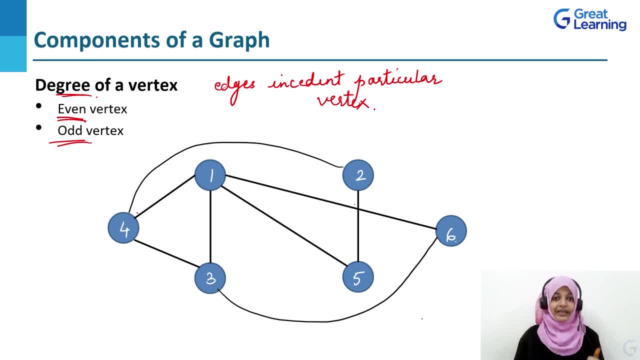 six vertices in total. Let us count the degree of each and every vertex. Let us start with vertex 1.. Vertex 1 has four edges, which is incident on it. Please note that here this particular graph does not have directed edges. This means that the edges will be counted twice, Once for the. 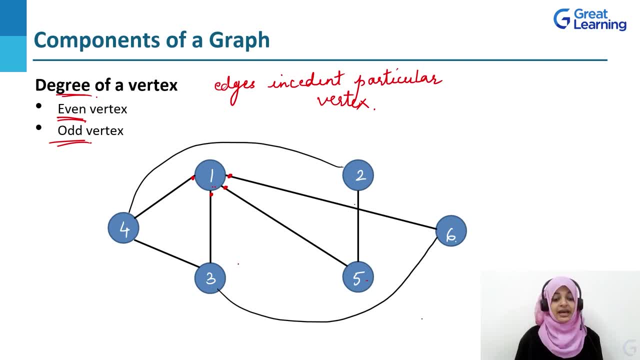 initial vertex and once for the final vertex. This is because this is an undirected graph, or a graph having a set of undirected edges. So here, vertex 1 has a degree of four, Vertex 2 has a degree of 2. coincidentally, Vertex 3 has a degree of 3. coincidentally, Vertex 4 again has a degree of 3.. Vertex 5 has a degree of 2 and, lastly, vertex 6 also has a degree of 2.. From this we can say that we have some even and some odd vertices, based just upon their degrees. As we can see, vertex 1 is an even vertex. 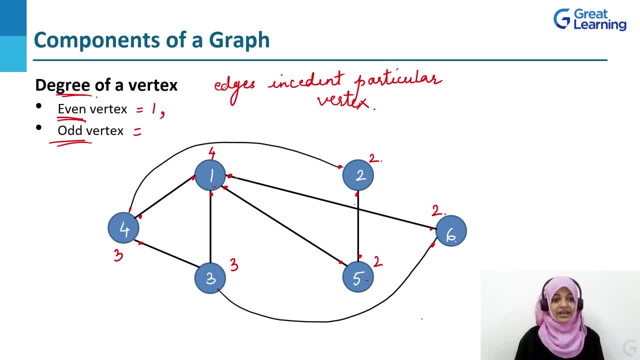 because the degree of that particular vertex is 4.. Similarly, vertex 2 is also an even vertex. Vertex 3 is an odd vertex because the degree of that particular vertex is odd. Next, vertex 4 is also an odd vertex. Lastly, vertex 5 and 6 are both even vertices because both of their degrees. 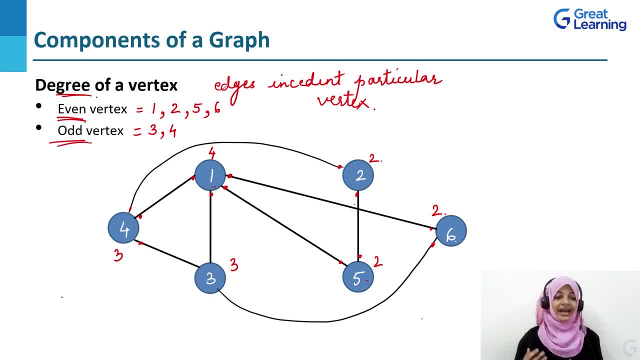 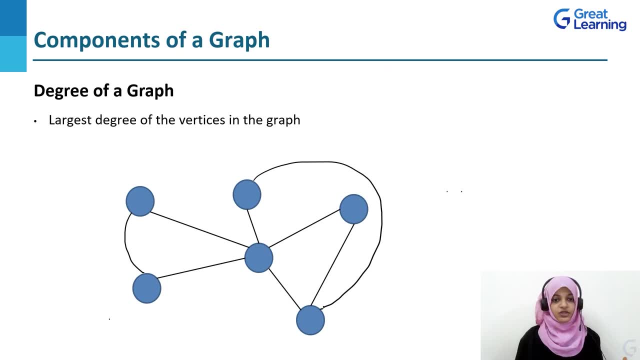 are 2, which is an even number. This is how we are actually able to identify the degree of a vertex. Next, let us understand what the degree of a whole graph is. So it's pretty simple. the degree of the graph is actually the largest degree of all of the vertices that are a part. 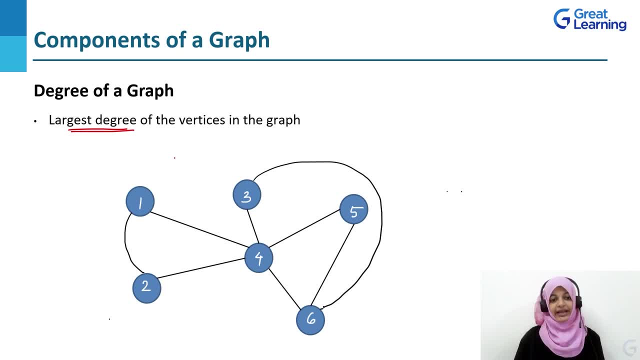 of that graph. So let us consider this particular diagram here. If we consider this diagram and we quickly just calculate the degree of each and every vertex, So the values written in red around all of the vertices are actually the degrees of all of those vertices. 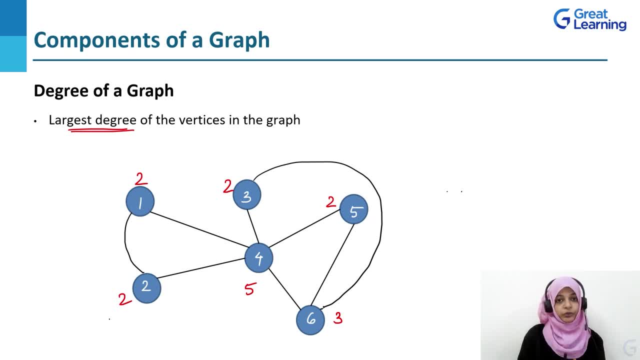 Now, from this you can see that we've got a lowest degree of 2 and a highest degree of 5.. The degree 5 is actually of vertex 4.. So, as we can understand, the degree of this graph will actually be the largest degree of the vertices in the graph. 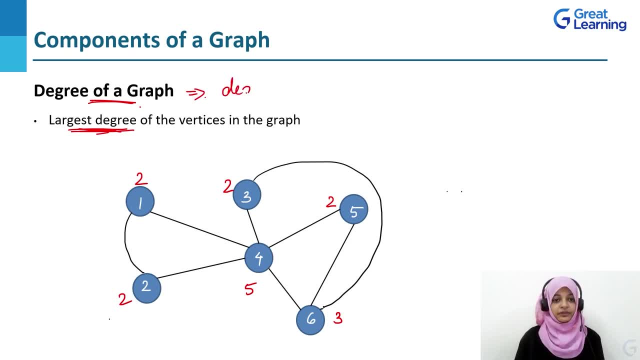 This implies that the degree of the graph will actually be the degree of vertex 4, which is actually equal to 5.. So the degree of this particular graph given here is 5.. Next, let's look at a very important concept, which is the handshaking lemma. 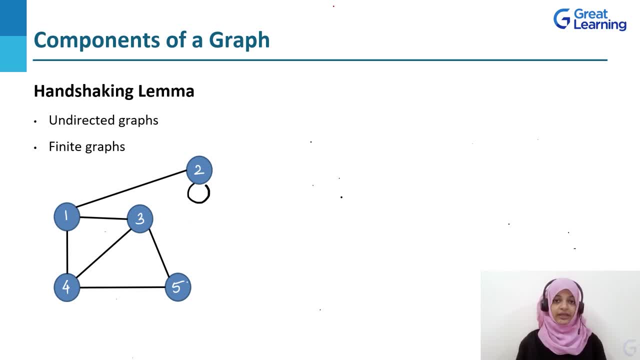 There are two important interpretations of the handshaking lemma. We will be looking at both of them here. The two prerequisites that we need to keep in mind while actually understanding the handshaking lemma is that these particular graphs are supposed to be finite in nature and they're supposed to be undirected graphs. This means 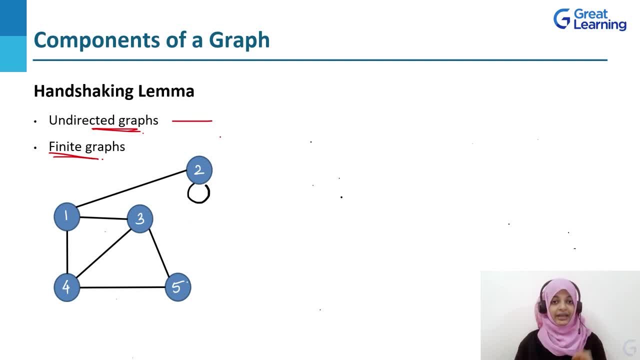 that each and every edge in the graph will be an undirected edge. That means no arrows. So here we need to have these two prerequisites in mind. Let us now look at the two interpretations of the handshaking lemma. The first interpretation says that the number of vertices touching odd edges 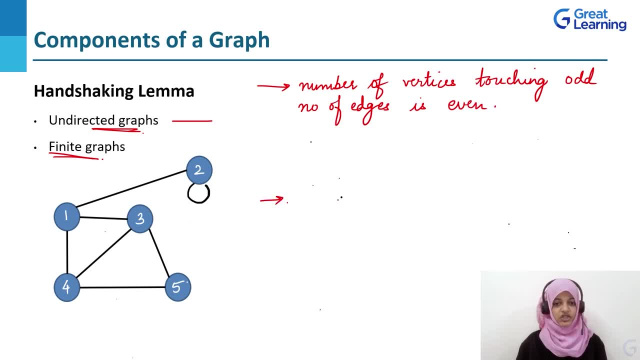 is equal to 1, and the second interpretation says that the sum of all degrees is twice the sum of edges. We will be looking at both of these interpretations with the help of the diagram given here. us look at the first interpretation. what does it mean? it means that if we've got vertices such that 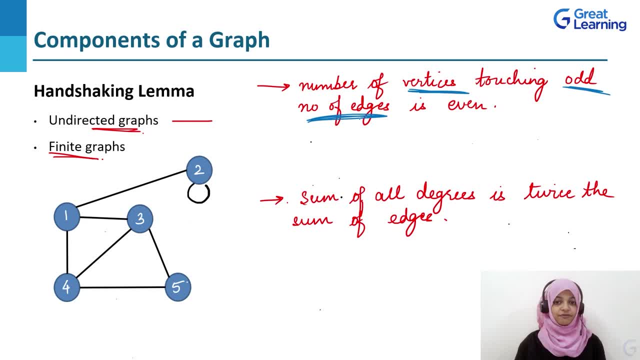 they're touching an odd number of edges. it implies that if the degree of the vertices is odd, then the number of such vertices odd degree is actually even. let us identify that in this particular diagram. so if we see here, then vertex 2 actually has an odd degree, vertex 1: 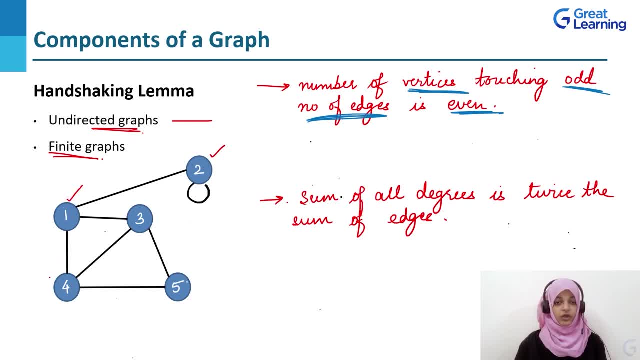 also has an odd degree. vertex 4 also has an odd degree. vertex 3 also has an odd degree. vertex 5, on the other hand, does not have an odd degree if you make any other edge from 5 to any other vertex given in this particular graph. 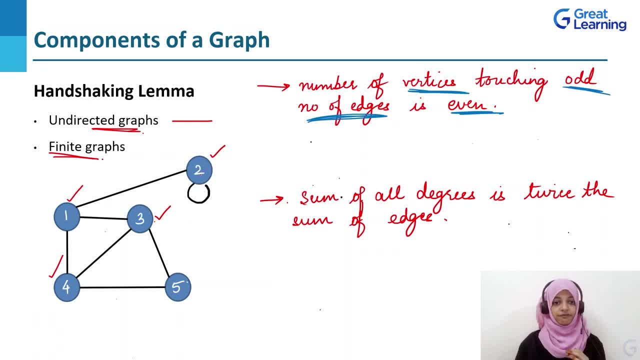 you will find that the balance of the whole graph will shift. This means that if you try to make 5 to have an odd degree, then you'll end up with an other vertex that will actually get converted from even to odd degree. So there is a balance maintained always. 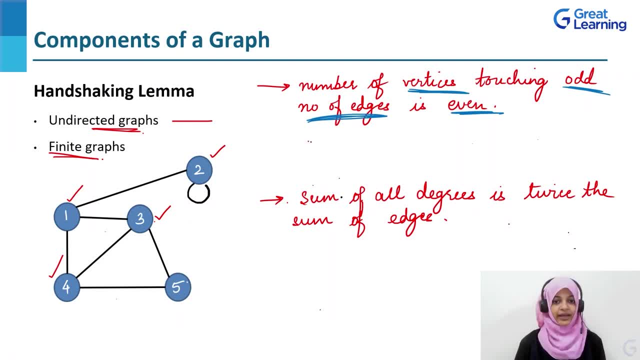 So, as you can see here, we're actually able to identify that all of the vertices which have odd degrees are actually 4.. And 4 is an even number. This means that the number of vertices having an odd degree is actually even. This is what the first interpretation of the handshaking lemma is. 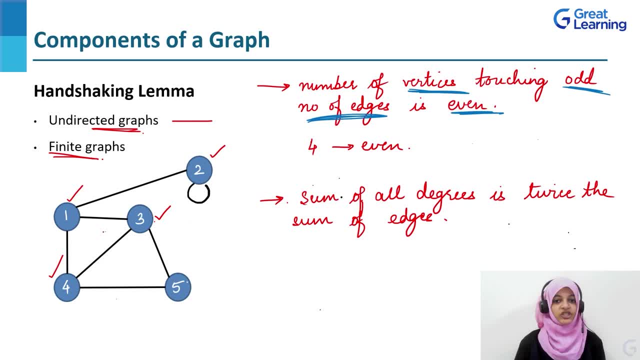 Next, let us understand the second interpretation of the handshaking lemma. So the second interpretation says that if we take the sum of all of the degrees, of all of the vertices that are a part of the graph, then that particular sum will be equal to 2 times the sum of degrees. 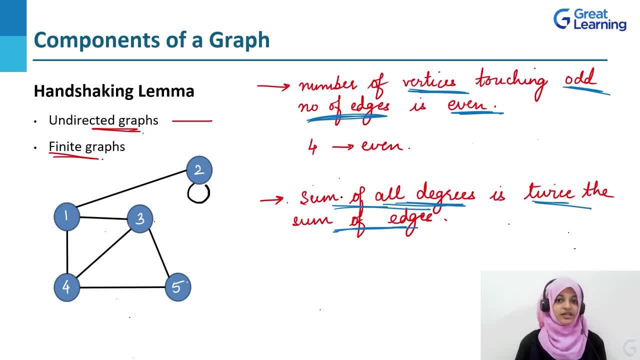 This is equal to the edges that are a part of the graph. So let us first identify the number of edges that we have in this particular graph. We've got 1,, 2,, 3,, 4,, 5,, 6, and 7 edges in this graph. 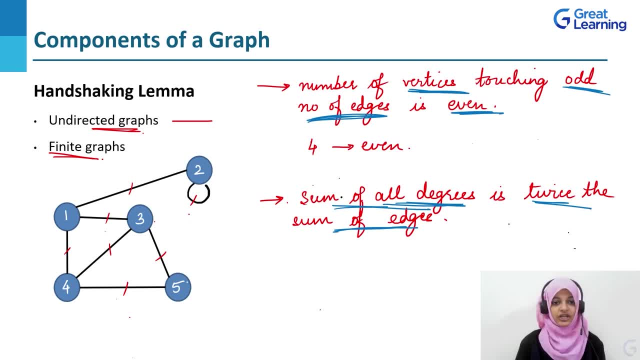 This last particular edge that looks circular in nature is actually a special edge, called a loop. It starts and ends at the exact same vertex, But this is also considered as an individual edge. Therefore, the number of edges in this particular graph is 7.. 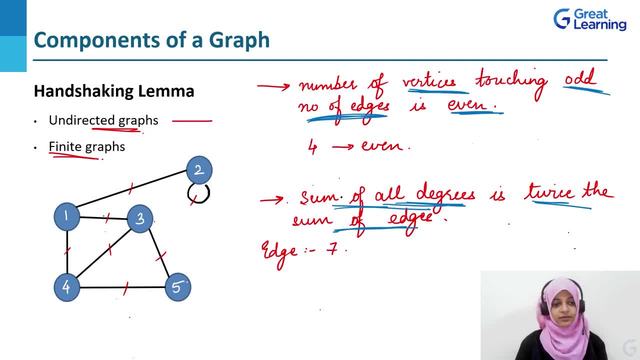 Next let us calculate the degrees of each and every vertex. So the degree of vertex 1 is 3.. Degree of vertex 4 is 3.. Degree of vertex 3 is also 3.. Degree of vertex 2 is also 3.. 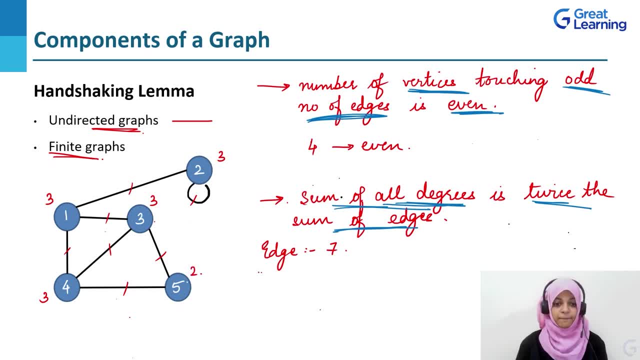 And degree of vertex 5 is 2.. Taking the sum of all the degrees, we get the sum as 3 plus 3 plus 3.. 3 plus 3 plus 2, which is actually equal to 14.. Now how do we actually equate these two? 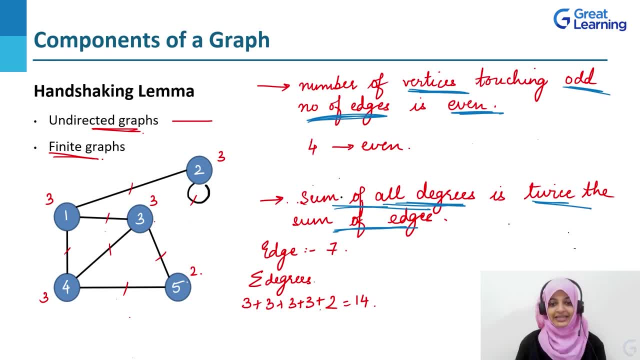 So if you read the statement very carefully here, this says that the sum of the degrees is actually equal to 2 times the number of edges. Now, 2 times the number of edges, which is 7, will actually give us 14, which is exactly equal to the sum of the degrees as we've obtained in this particular graph. Now 2 times the number of edges, which is 7, will actually give us 14, which is exactly equal to the sum of the degrees as we've obtained in this particular graph. Now, 2 times the number of edges, which is 7, will actually give us 14, which is exactly equal to the sum of the degrees as we've obtained in this particular graph. Now 2 times the number of edges, which is 7, will actually give us 14, which is exactly equal to the sum of the degrees as we've obtained in this particular graph. Now, 2 times the number of edges, which is 7, will actually give us 14, which is exactly equal to the sum of the degrees as we've obtained in this particular graph. 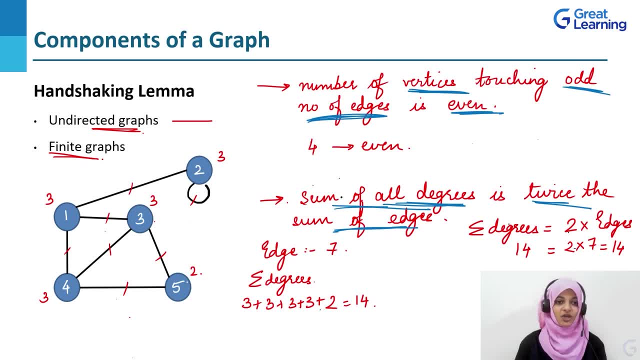 Now 2 times the number of edges, which is 7, will actually give us 14, which is exactly equal to the sum of the degrees as we've obtained in this particular graph. Now, 2 times the number of edges, which is 7, will actually give us 14, which is exactly equal to the sum of the degrees as we've obtained in this particular graph. 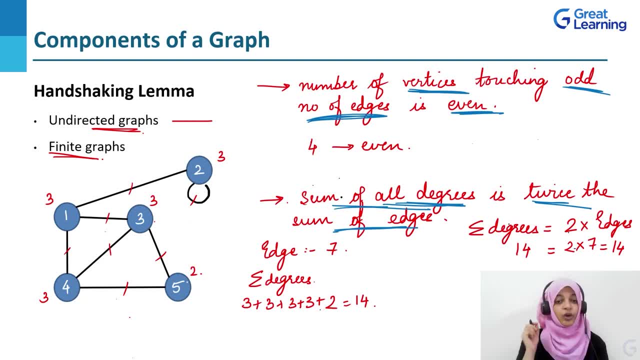 Now 2 times the number of edges, which is 7, will actually give us 14, which is exactly equal to the sum of the degrees as we've obtained in this particular graph. Now, 2 times the number of edges, which is 7, will actually give us 14, which is exactly equal to the sum of the degrees as we've obtained in this particular graph. 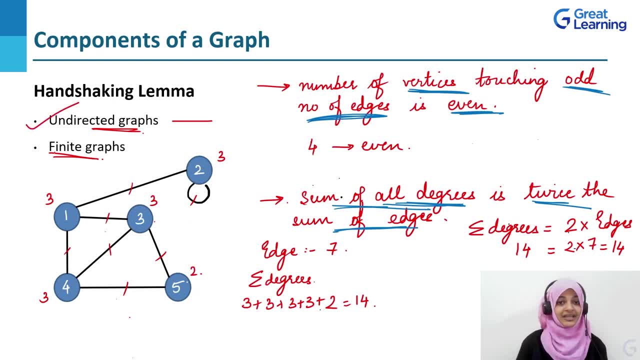 Now 2 times the number of edges, which is 7, will actually give us 14, which is exactly equal to the sum of the degrees as we've obtained in this particular graph. Now, 2 times the number of edges, which is 7, will actually give us 14, which is exactly equal to the sum of the degrees as we've obtained in this particular graph. 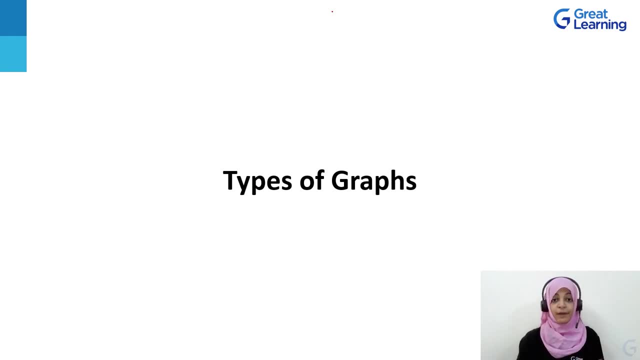 Now 2 times the number of edges, which is 7, will actually give us 14, which is exactly equal to the sum of the degrees as we've obtained in this particular graph. Now, 2 times the number of edges, which is 7, will actually give us 14, which is exactly equal to the sum of the degrees as we've obtained in this particular graph. 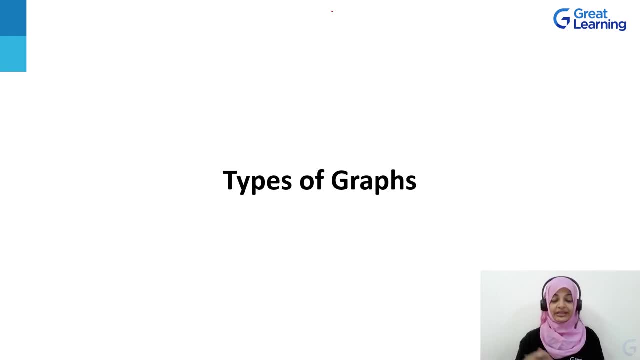 Now 2 times the number of edges, which is 7, will actually give us 14, which is exactly equal to the sum of the degrees as we've obtained in this particular graph. Now, 2 times the number of edges, which is 7, will actually give us 14, which is exactly equal to the sum of the degrees as we've obtained in this particular graph. 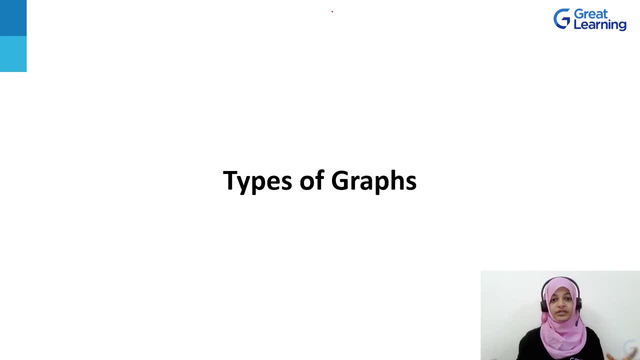 Now 2 times the number of edges, which is 7, will actually give us 14, which is exactly equal to the sum of the degrees as we've obtained in this particular graph. Now, 2 times the number of edges, which is 7, will actually give us 14, which is exactly equal to the sum of the degrees as we've obtained in this particular graph. 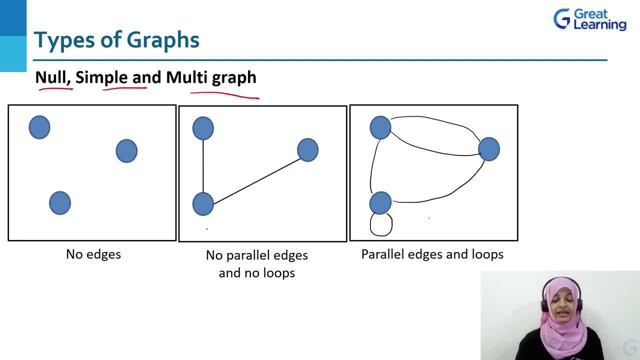 Now 2 times the number of edges, which is 7, will actually give us 14, which is exactly equal to the sum of the degrees as we've obtained in this particular graph. Now, 2 times the number of edges, which is 7, will actually give us 14, which is exactly equal to the sum of the degrees as we've obtained in this particular graph. 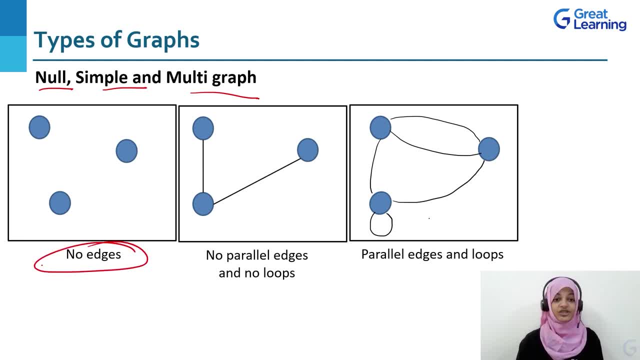 Now 2 times the number of edges, which is 7, will actually give us 14, which is exactly equal to the sum of the degrees as we've obtained in this particular graph. Now, 2 times the number of edges, which is 7, will actually give us 14, which is exactly equal to the sum of the degrees as we've obtained in this particular graph. 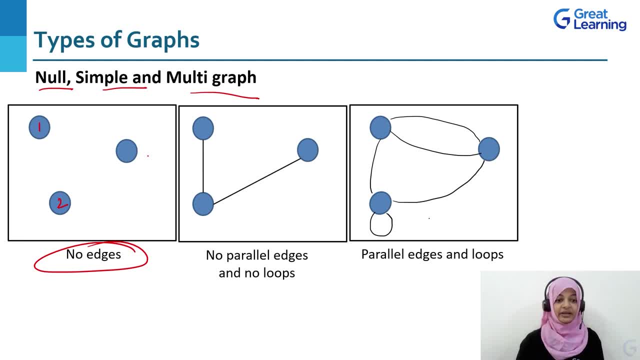 Now 2 times the number of edges, which is 7, will actually give us 14, which is exactly equal to the sum of the degrees as we've obtained in this particular graph. Now, 2 times the number of edges, which is 7, will actually give us 14, which is exactly equal to the sum of the degrees as we've obtained in this particular graph. 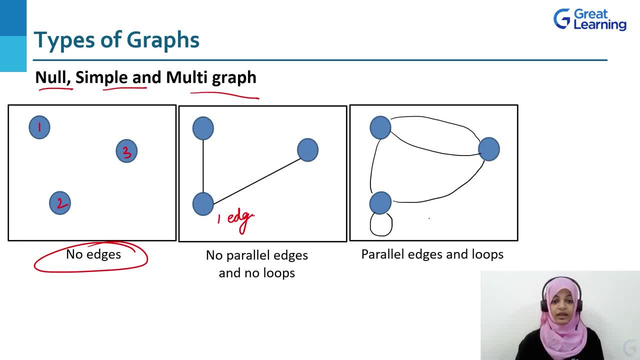 Now 2 times the number of edges, which is 7, will actually give us 14, which is exactly equal to the sum of the degrees as we've obtained in this particular graph. Now, 2 times the number of edges, which is 7, will actually give us 14, which is exactly equal to the sum of the degrees as we've obtained in this particular graph. 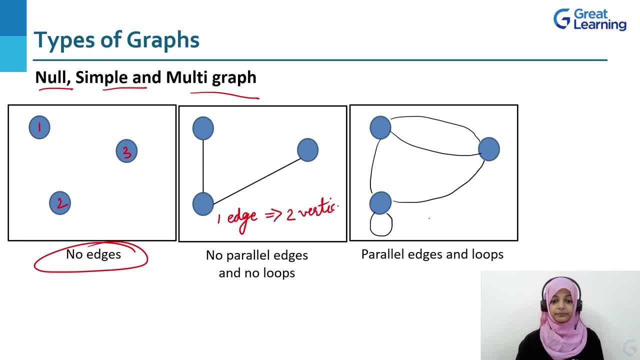 Now 2 times the number of edges, which is 7, will actually give us 14, which is exactly equal to the sum of the degrees as we've obtained in this particular graph. Now, 2 times the number of edges, which is 7, will actually give us 14, which is exactly equal to the sum of the degrees as we've obtained in this particular graph. 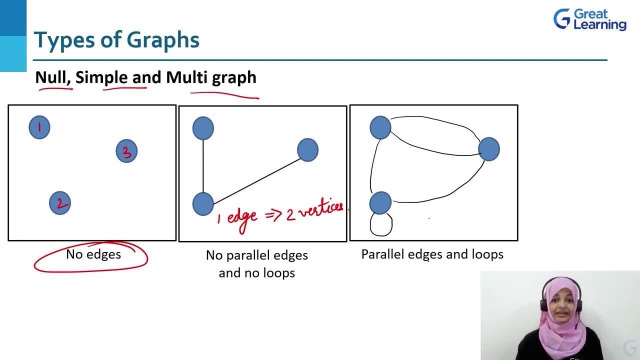 Now 2 times the number of edges, which is 7, will actually give us 14, which is exactly equal to the sum of the degrees as we've obtained in this particular graph. Now, 2 times the number of edges, which is 7, will actually give us 14, which is exactly equal to the sum of the degrees as we've obtained in this particular graph. 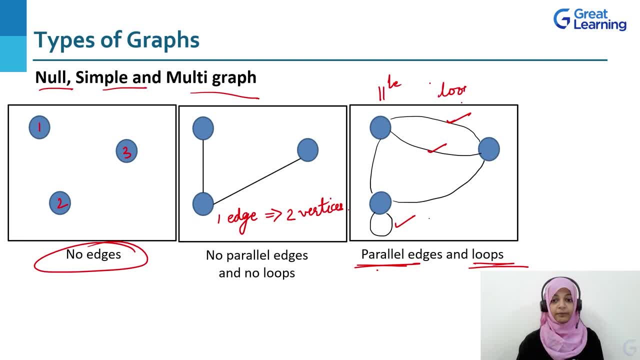 Now 2 times the number of edges, which is 7, will actually give us 14, which is exactly equal to the sum of the degrees as we've obtained in this particular graph. Now, 2 times the number of edges, which is 7, will actually give us 14, which is exactly equal to the sum of the degrees as we've obtained in this particular graph. 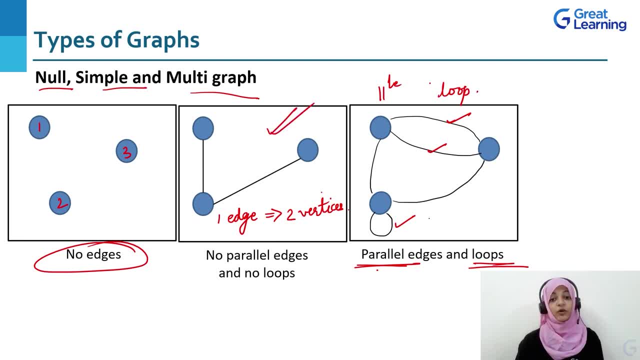 Now 2 times the number of edges, which is 7, will actually give us 14, which is exactly equal to the sum of the degrees as we've obtained in this particular graph. Now, 2 times the number of edges, which is 7, will actually give us 14, which is exactly equal to the sum of the degrees as we've obtained in this particular graph. 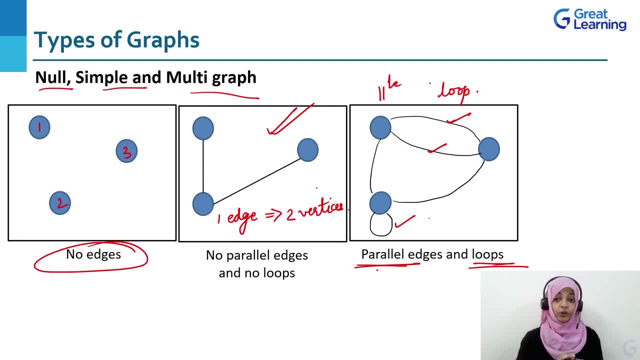 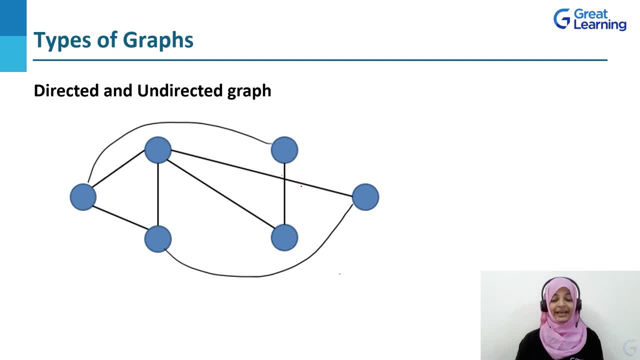 Now 2 times the number of edges, which is 7, will actually give us 14, which is exactly equal to the sum of the degrees as we've obtained in this particular graph. Now, 2 times the number of edges, which is 7, will actually give us 14, which is exactly equal to the sum of the degrees as we've obtained in this particular graph. 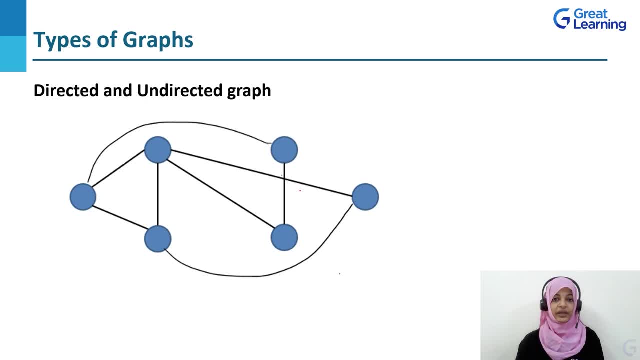 Now 2 times the number of edges, which is 7, will actually give us 14, which is exactly equal to the sum of the degrees as we've obtained in this particular graph. Now, 2 times the number of edges, which is 7, will actually give us 14, which is exactly equal to the sum of the degrees as we've obtained in this particular graph. 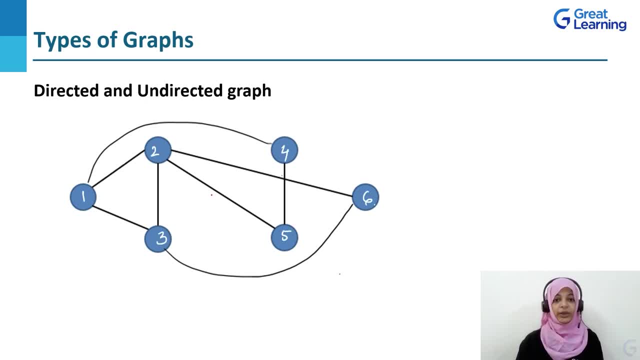 Now 2 times the number of edges, which is 7, will actually give us 14, which is exactly equal to the sum of the degrees as we've obtained in this particular graph. Now, 2 times the number of edges, which is 7, will actually give us 14, which is exactly equal to the sum of the degrees as we've obtained in this particular graph. 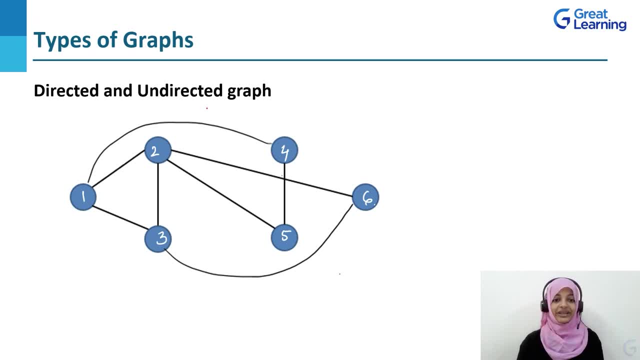 Now 2 times the number of edges, which is 7, will actually give us 14, which is exactly equal to the sum of the degrees as we've obtained in this particular graph. Now, 2 times the number of edges, which is 7, will actually give us 14, which is exactly equal to the sum of the degrees as we've obtained in this particular graph. 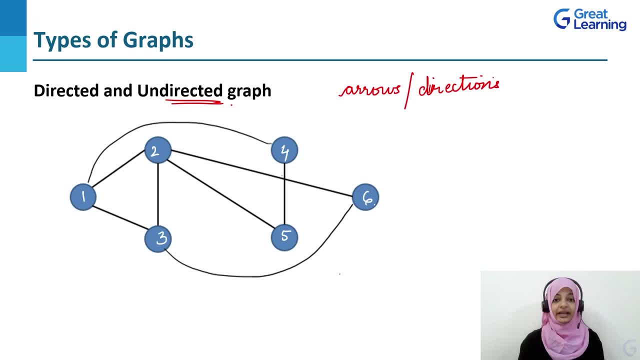 Now 2 times the number of edges, which is 7, will actually give us 14, which is exactly equal to the sum of the degrees as we've obtained in this particular graph. Now, 2 times the number of edges, which is 7, will actually give us 14, which is exactly equal to the sum of the degrees as we've obtained in this particular graph. 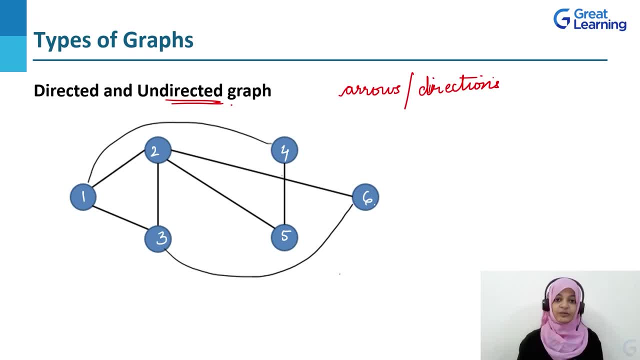 Now 2 times the number of edges, which is 7, will actually give us 14, which is exactly equal to the sum of the degrees as we've obtained in this particular graph. Now, 2 times the number of edges, which is 7, will actually give us 14, which is exactly equal to the sum of the degrees as we've obtained in this particular graph. 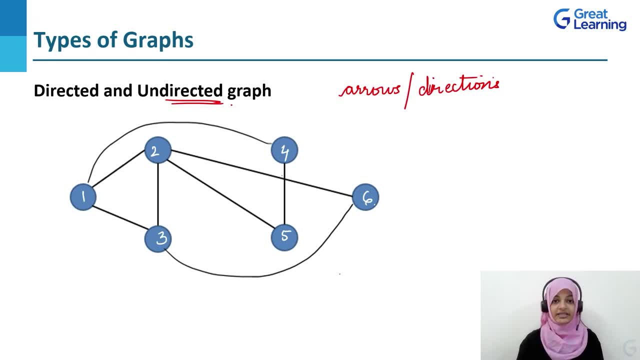 Now 2 times the number of edges, which is 7, will actually give us 14, which is exactly equal to the sum of the degrees as we've obtained in this particular graph. Now, 2 times the number of edges, which is 7, will actually give us 14, which is exactly equal to the sum of the degrees as we've obtained in this particular graph. 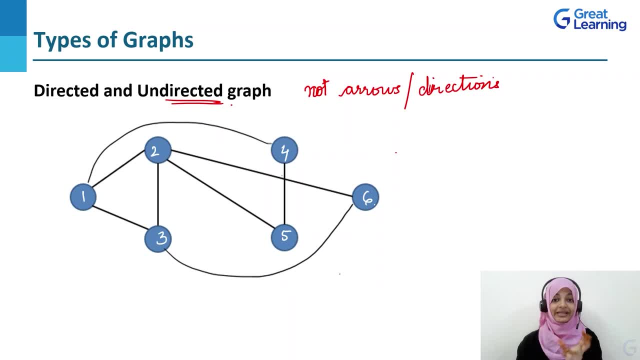 Now 2 times the number of edges, which is 7, will actually give us 14, which is exactly equal to the sum of the degrees as we've obtained in this particular graph. Now, 2 times the number of edges, which is 7, will actually give us 14, which is exactly equal to the sum of the degrees as we've obtained in this particular graph. 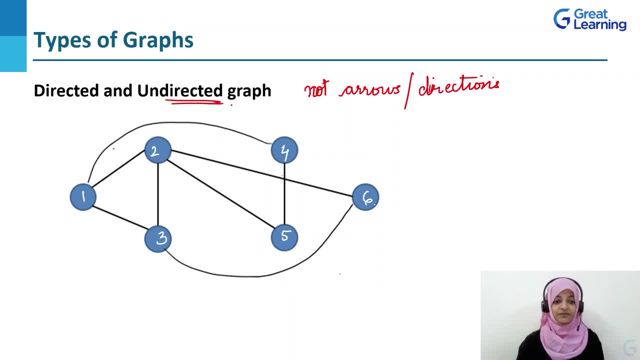 Now 2 times the number of edges, which is 7, will actually give us 14, which is exactly equal to the sum of the degrees as we've obtained in this particular graph. Now, 2 times the number of edges, which is 7, will actually give us 14, which is exactly equal to the sum of the degrees as we've obtained in this particular graph. 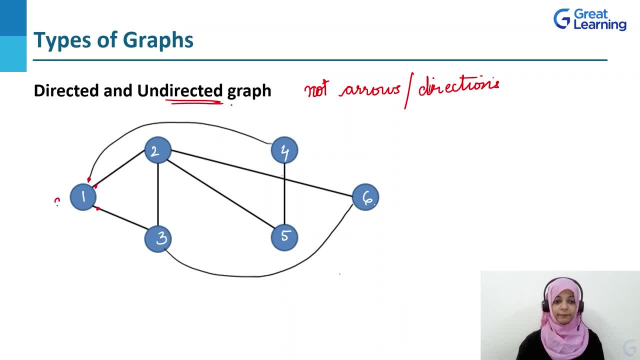 Now 2 times the number of edges, which is 7, will actually give us 14, which is exactly equal to the sum of the degrees as we've obtained in this particular graph. Now, 2 times the number of edges, which is 7, will actually give us 14, which is exactly equal to the sum of the degrees as we've obtained in this particular graph. 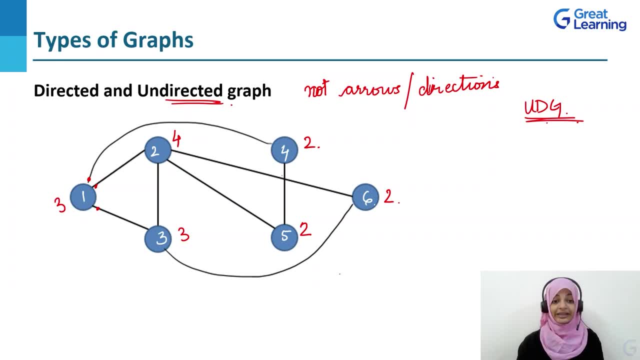 Now 2 times the number of edges, which is 7, will actually give us 14, which is exactly equal to the sum of the degrees as we've obtained in this particular graph. Now, 2 times the number of edges, which is 7, will actually give us 14, which is exactly equal to the sum of the degrees as we've obtained in this particular graph. 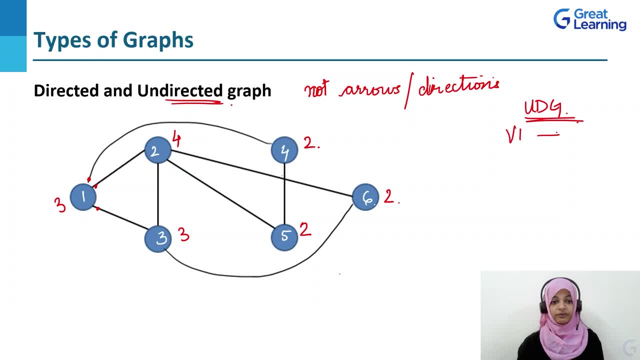 Now 2 times the number of edges, which is 7, will actually give us 14, which is exactly equal to the sum of the degrees as we've obtained in this particular graph. Now, 2 times the number of edges, which is 7, will actually give us 14, which is exactly equal to the sum of the degrees as we've obtained in this particular graph. 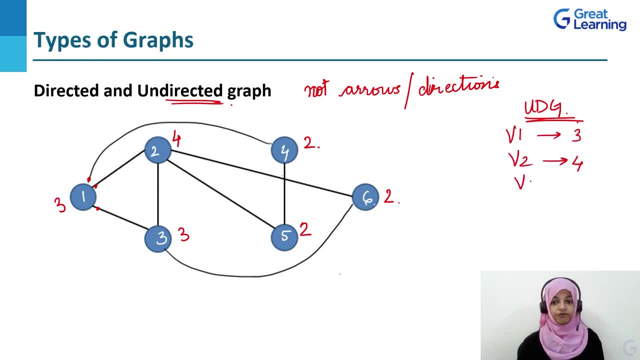 Now 2 times the number of edges, which is 7, will actually give us 14, which is exactly equal to the sum of the degrees as we've obtained in this particular graph. Now, 2 times the number of edges, which is 7, will actually give us 14, which is exactly equal to the sum of the degrees as we've obtained in this particular graph. 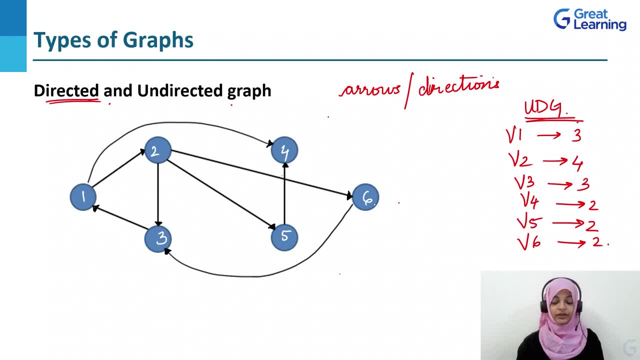 Now 2 times the number of edges, which is 7, will actually give us 14, which is exactly equal to the sum of the degrees as we've obtained in this particular graph. Now, 2 times the number of edges, which is 7, will actually give us 14, which is exactly equal to the sum of the degrees as we've obtained in this particular graph. 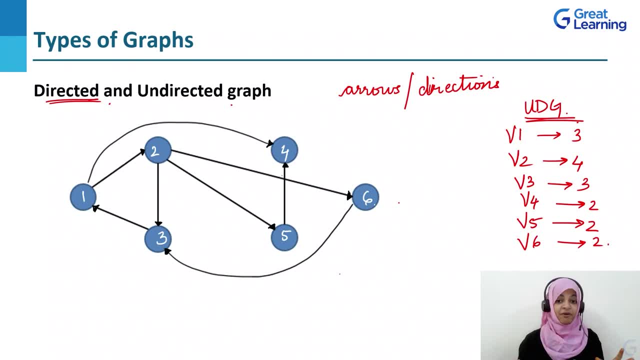 Now 2 times the number of edges, which is 7, will actually give us 14, which is exactly equal to the sum of the degrees as we've obtained in this particular graph. Now, 2 times the number of edges, which is 7, will actually give us 14, which is exactly equal to the sum of the degrees as we've obtained in this particular graph. 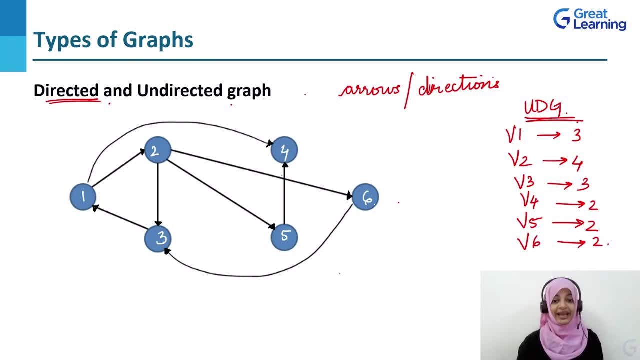 Now 2 times the number of edges, which is 7, will actually give us 14, which is exactly equal to the sum of the degrees as we've obtained in this particular graph. Now, 2 times the number of edges, which is 7, will actually give us 14, which is exactly equal to the sum of the degrees as we've obtained in this particular graph. 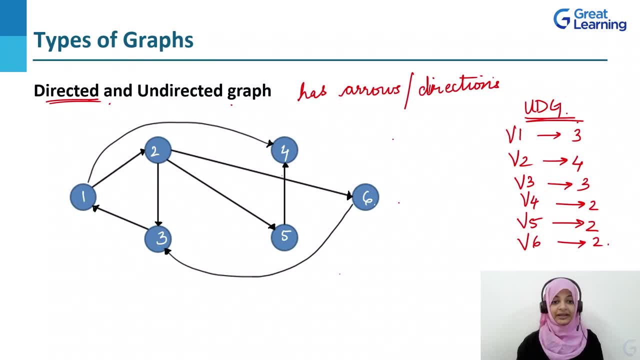 Now 2 times the number of edges, which is 7, will actually give us 14, which is exactly equal to the sum of the degrees as we've obtained in this particular graph. Now, 2 times the number of edges, which is 7, will actually give us 14, which is exactly equal to the sum of the degrees as we've obtained in this particular graph. 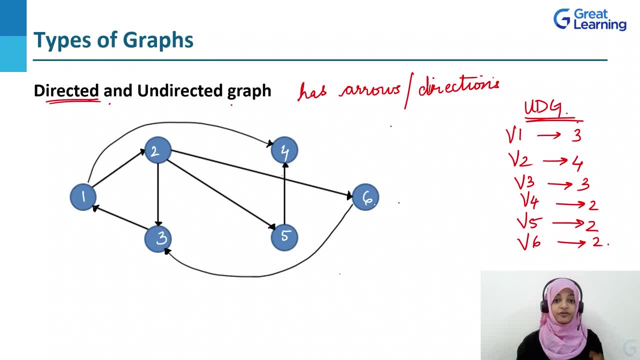 Now 2 times the number of edges, which is 7, will actually give us 14, which is exactly equal to the sum of the degrees as we've obtained in this particular graph. Now, 2 times the number of edges, which is 7, will actually give us 14, which is exactly equal to the sum of the degrees as we've obtained in this particular graph. 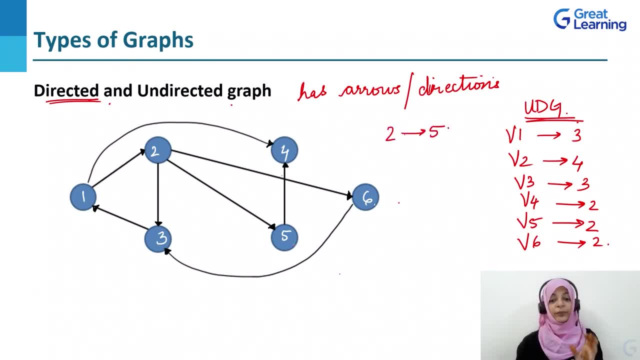 Now 2 times the number of edges, which is 7, will actually give us 14, which is exactly equal to the sum of the degrees as we've obtained in this particular graph. Now, 2 times the number of edges, which is 7, will actually give us 14, which is exactly equal to the sum of the degrees as we've obtained in this particular graph. 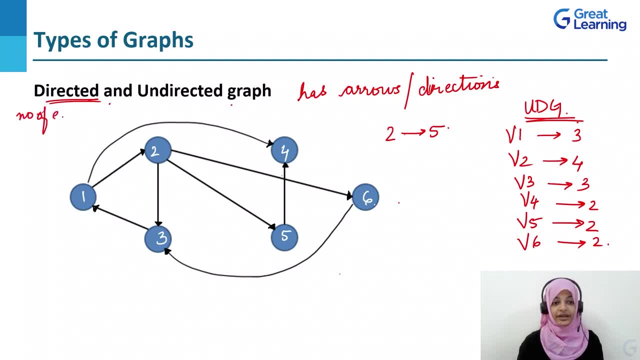 Now 2 times the number of edges, which is 7, will actually give us 14, which is exactly equal to the sum of the degrees as we've obtained in this particular graph. Now, 2 times the number of edges, which is 7, will actually give us 14, which is exactly equal to the sum of the degrees as we've obtained in this particular graph. 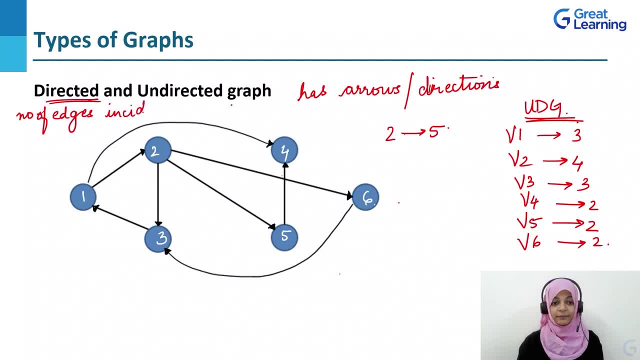 Now 2 times the number of edges, which is 7, will actually give us 14, which is exactly equal to the sum of the degrees as we've obtained in this particular graph. Now, 2 times the number of edges, which is 7, will actually give us 14, which is exactly equal to the sum of the degrees as we've obtained in this particular graph. 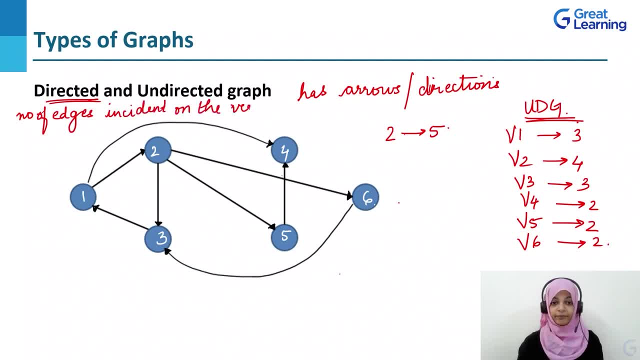 Now 2 times the number of edges, which is 7, will actually give us 14, which is exactly equal to the sum of the degrees as we've obtained in this particular graph. Now, 2 times the number of edges, which is 7, will actually give us 14, which is exactly equal to the sum of the degrees as we've obtained in this particular graph. 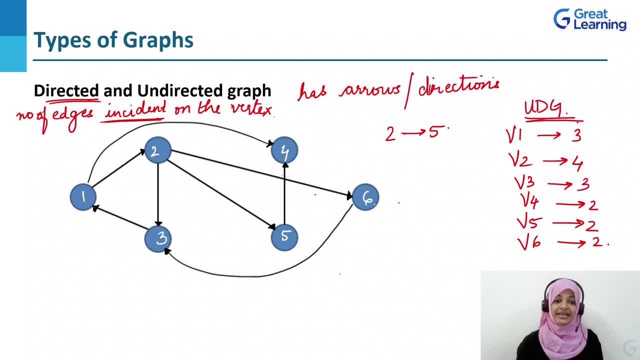 Now 2 times the number of edges, which is 7, will actually give us 14, which is exactly equal to the sum of the degrees as we've obtained in this particular graph. Now, 2 times the number of edges, which is 7, will actually give us 14, which is exactly equal to the sum of the degrees as we've obtained in this particular graph. 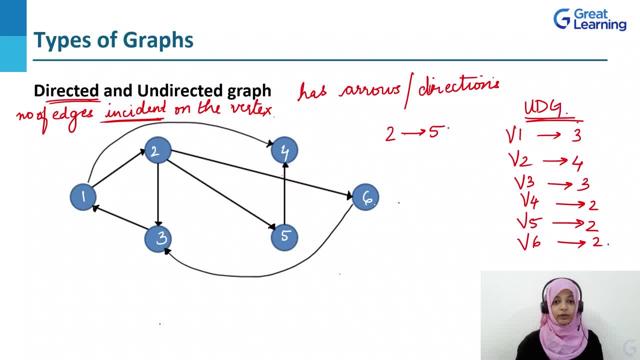 Now 2 times the number of edges, which is 7, will actually give us 14, which is exactly equal to the sum of the degrees as we've obtained in this particular graph. Now, 2 times the number of edges, which is 7, will actually give us 14, which is exactly equal to the sum of the degrees as we've obtained in this particular graph. 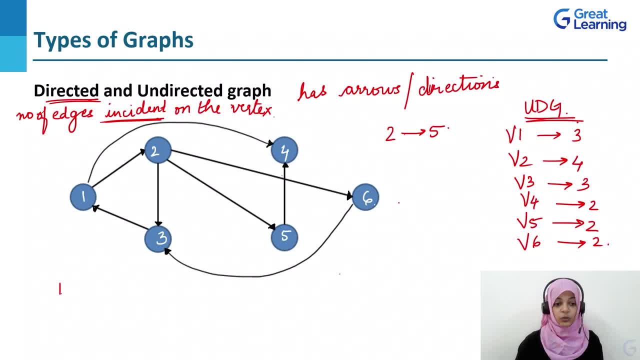 Now 2 times the number of edges, which is 7, will actually give us 14, which is exactly equal to the sum of the degrees as we've obtained in this particular graph. Now, 2 times the number of edges, which is 7, will actually give us 14, which is exactly equal to the sum of the degrees as we've obtained in this particular graph. 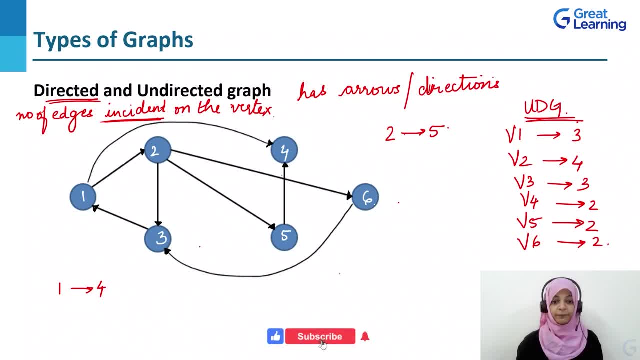 Now 2 times the number of edges, which is 7, will actually give us 14, which is exactly equal to the sum of the degrees as we've obtained in this particular graph. Now, 2 times the number of edges, which is 7, will actually give us 14, which is exactly equal to the sum of the degrees as we've obtained in this particular graph. 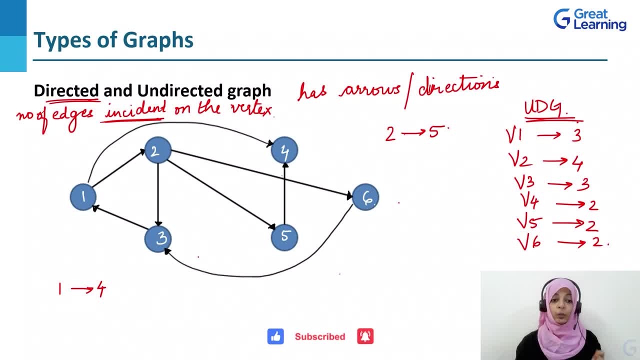 Now 2 times the number of edges, which is 7, will actually give us 14, which is exactly equal to the sum of the degrees as we've obtained in this particular graph. Now, 2 times the number of edges, which is 7, will actually give us 14, which is exactly equal to the sum of the degrees as we've obtained in this particular graph. 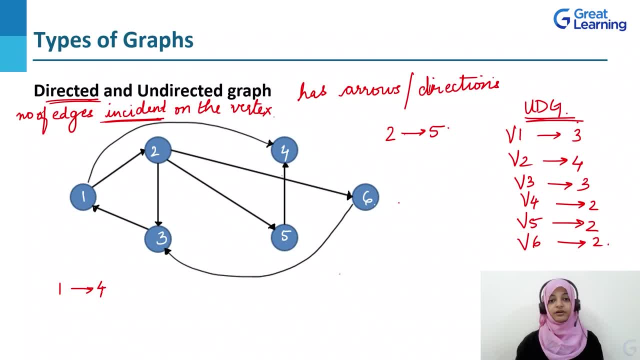 Now 2 times the number of edges, which is 7, will actually give us 14, which is exactly equal to the sum of the degrees as we've obtained in this particular graph. Now, 2 times the number of edges, which is 7, will actually give us 14, which is exactly equal to the sum of the degrees as we've obtained in this particular graph. 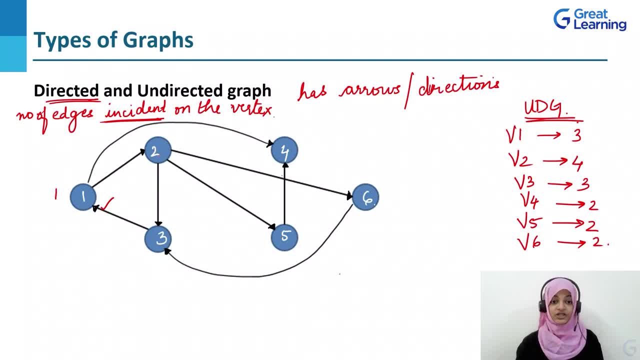 Now 2 times the number of edges, which is 7, will actually give us 14, which is exactly equal to the sum of the degrees as we've obtained in this particular graph. Now, 2 times the number of edges, which is 7, will actually give us 14, which is exactly equal to the sum of the degrees as we've obtained in this particular graph. 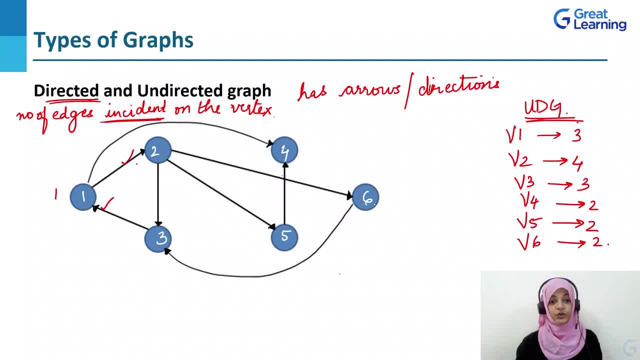 Now 2 times the number of edges, which is 7, will actually give us 14, which is exactly equal to the sum of the degrees as we've obtained in this particular graph. Now, 2 times the number of edges, which is 7, will actually give us 14, which is exactly equal to the sum of the degrees as we've obtained in this particular graph. 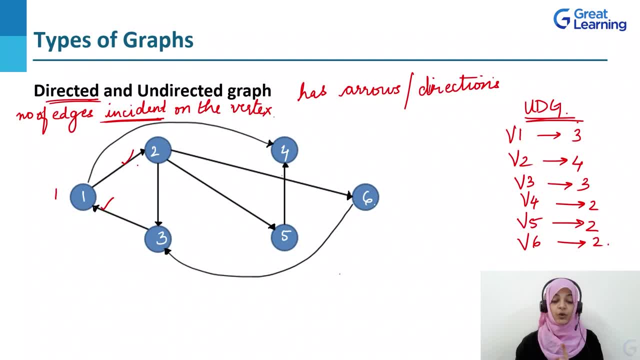 Now 2 times the number of edges, which is 7, will actually give us 14, which is exactly equal to the sum of the degrees as we've obtained in this particular graph. Now, 2 times the number of edges, which is 7, will actually give us 14, which is exactly equal to the sum of the degrees as we've obtained in this particular graph. 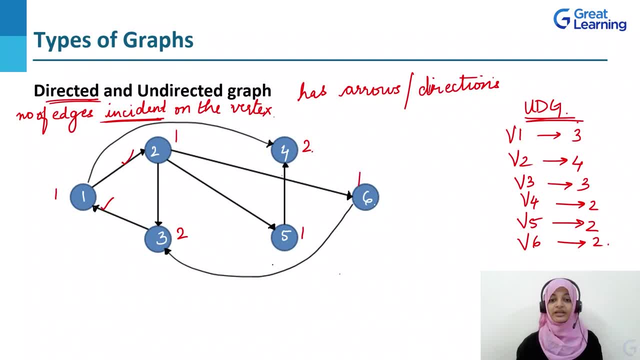 Now 2 times the number of edges, which is 7, will actually give us 14, which is exactly equal to the sum of the degrees as we've obtained in this particular graph. Now, 2 times the number of edges, which is 7, will actually give us 14, which is exactly equal to the sum of the degrees as we've obtained in this particular graph. 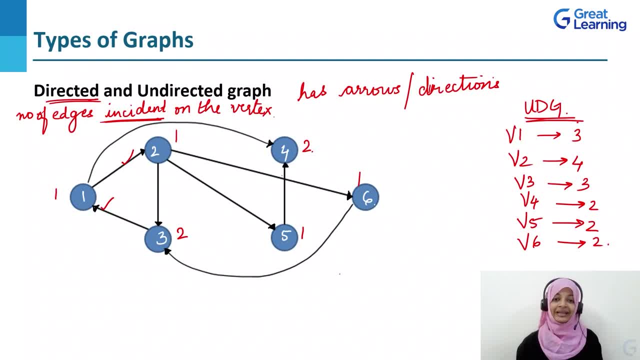 Now 2 times the number of edges, which is 7, will actually give us 14, which is exactly equal to the sum of the degrees as we've obtained in this particular graph. Now, 2 times the number of edges, which is 7, will actually give us 14, which is exactly equal to the sum of the degrees as we've obtained in this particular graph. 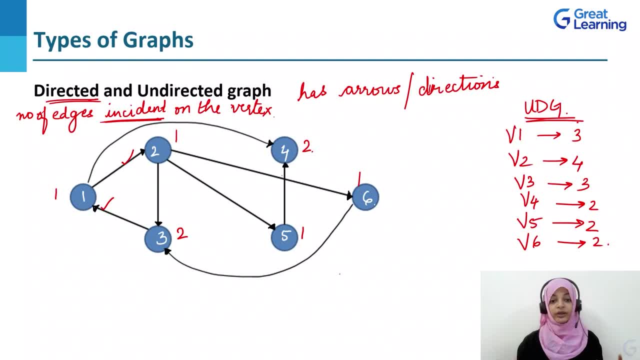 Now 2 times the number of edges, which is 7, will actually give us 14, which is exactly equal to the sum of the degrees as we've obtained in this particular graph. Now, 2 times the number of edges, which is 7, will actually give us 14, which is exactly equal to the sum of the degrees as we've obtained in this particular graph. 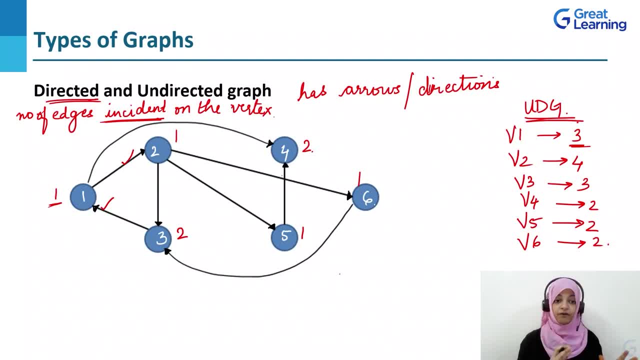 Now 2 times the number of edges, which is 7, will actually give us 14, which is exactly equal to the sum of the degrees as we've obtained in this particular graph. Now, 2 times the number of edges, which is 7, will actually give us 14, which is exactly equal to the sum of the degrees as we've obtained in this particular graph. 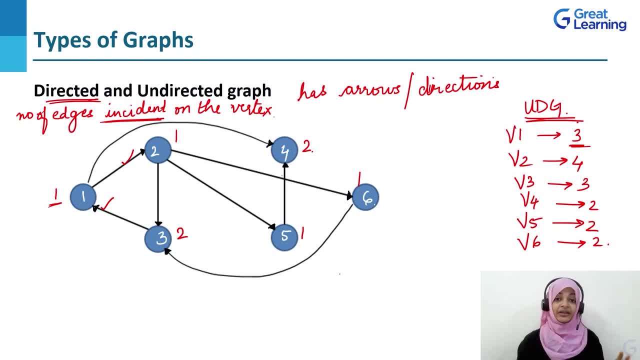 Now 2 times the number of edges, which is 7, will actually give us 14, which is exactly equal to the sum of the degrees as we've obtained in this particular graph. Now, 2 times the number of edges, which is 7, will actually give us 14, which is exactly equal to the sum of the degrees as we've obtained in this particular graph. 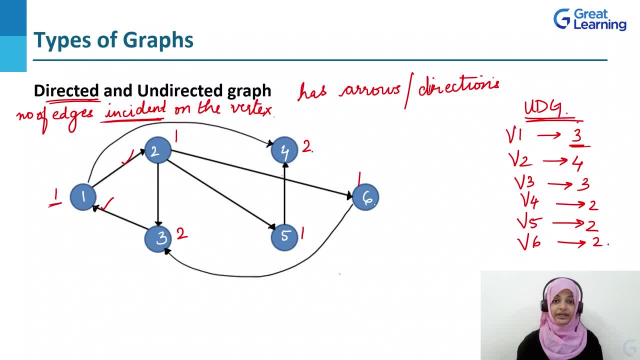 Now 2 times the number of edges, which is 7, will actually give us 14, which is exactly equal to the sum of the degrees as we've obtained in this particular graph. Now, 2 times the number of edges, which is 7, will actually give us 14, which is exactly equal to the sum of the degrees as we've obtained in this particular graph. 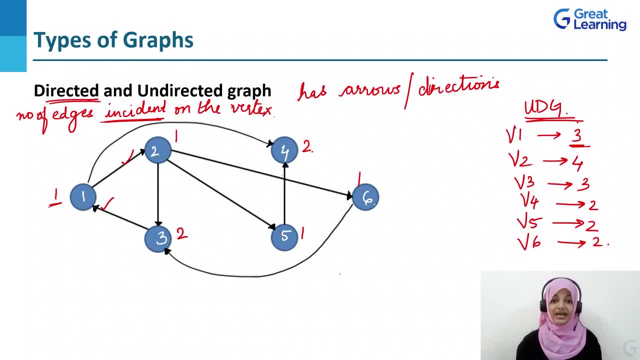 Now 2 times the number of edges, which is 7, will actually give us 14, which is exactly equal to the sum of the degrees as we've obtained in this particular graph. Now, 2 times the number of edges, which is 7, will actually give us 14, which is exactly equal to the sum of the degrees as we've obtained in this particular graph. 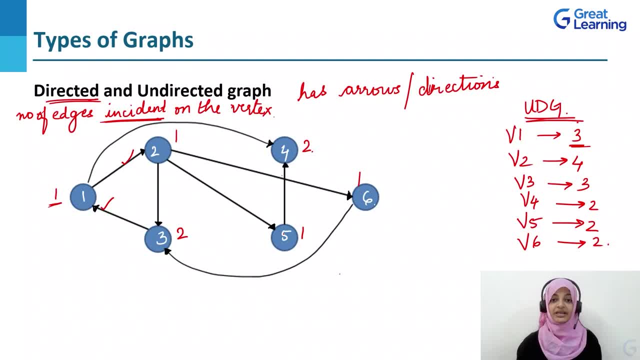 Now 2 times the number of edges, which is 7, will actually give us 14, which is exactly equal to the sum of the degrees as we've obtained in this particular graph. Now, 2 times the number of edges, which is 7, will actually give us 14, which is exactly equal to the sum of the degrees as we've obtained in this particular graph. 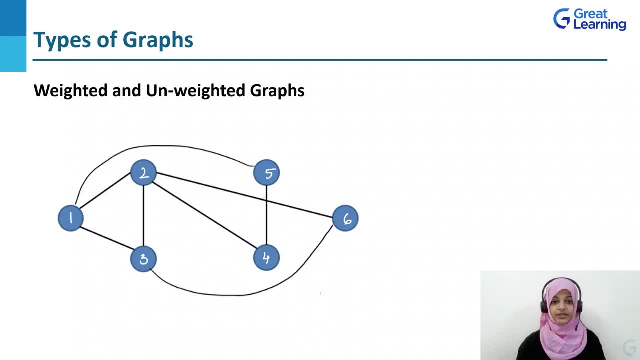 Now 2 times the number of edges, which is 7, will actually give us 14, which is exactly equal to the sum of the degrees as we've obtained in this particular graph. Now, 2 times the number of edges, which is 7, will actually give us 14, which is exactly equal to the sum of the degrees as we've obtained in this particular graph. 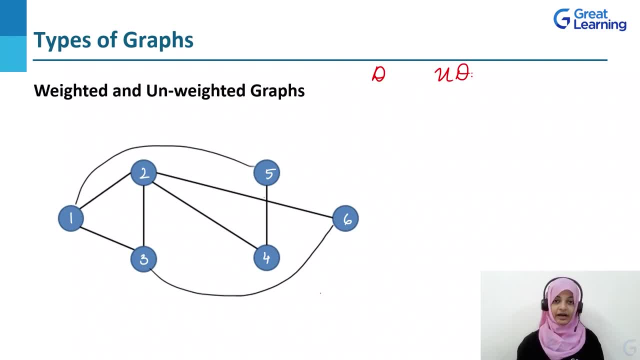 Now 2 times the number of edges, which is 7, will actually give us 14, which is exactly equal to the sum of the degrees as we've obtained in this particular graph. Now, 2 times the number of edges, which is 7, will actually give us 14, which is exactly equal to the sum of the degrees as we've obtained in this particular graph. 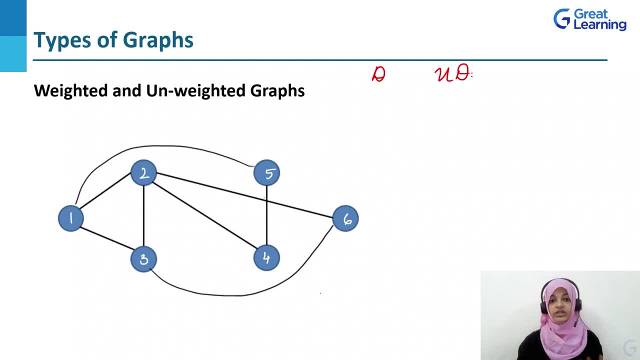 Now 2 times the number of edges, which is 7, will actually give us 14, which is exactly equal to the sum of the degrees as we've obtained in this particular graph. Now, 2 times the number of edges, which is 7, will actually give us 14, which is exactly equal to the sum of the degrees as we've obtained in this particular graph. 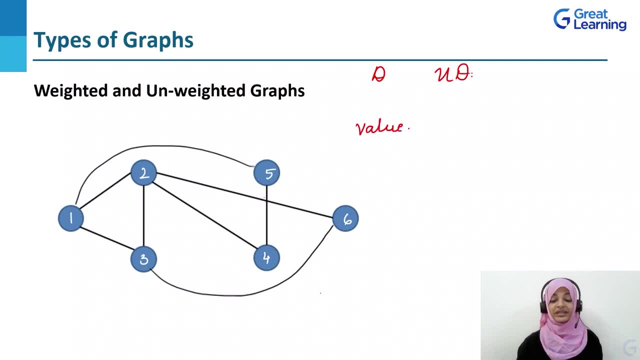 Now 2 times the number of edges, which is 7, will actually give us 14, which is exactly equal to the sum of the degrees as we've obtained in this particular graph. Now, 2 times the number of edges, which is 7, will actually give us 14, which is exactly equal to the sum of the degrees as we've obtained in this particular graph. 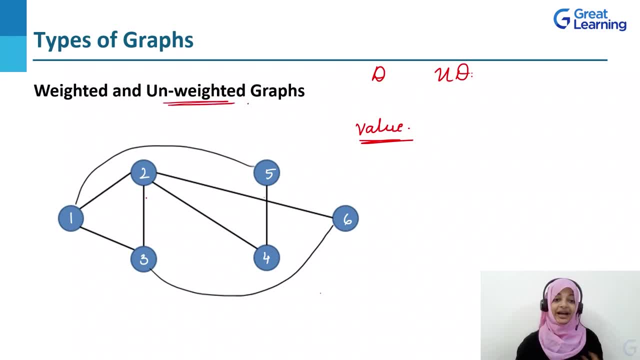 Now 2 times the number of edges, which is 7, will actually give us 14, which is exactly equal to the sum of the degrees as we've obtained in this particular graph. Now, 2 times the number of edges, which is 7, will actually give us 14, which is exactly equal to the sum of the degrees as we've obtained in this particular graph. 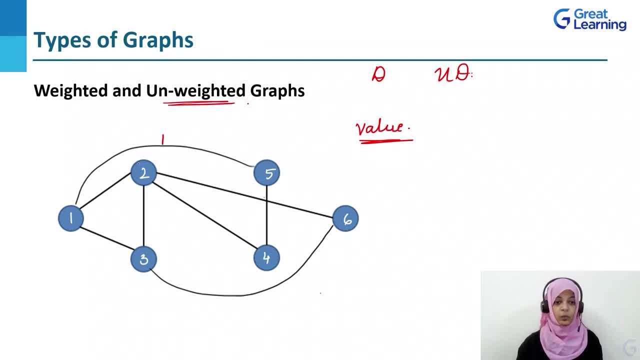 Now 2 times the number of edges, which is 7, will actually give us 14, which is exactly equal to the sum of the degrees as we've obtained in this particular graph. Now, 2 times the number of edges, which is 7, will actually give us 14, which is exactly equal to the sum of the degrees as we've obtained in this particular graph. 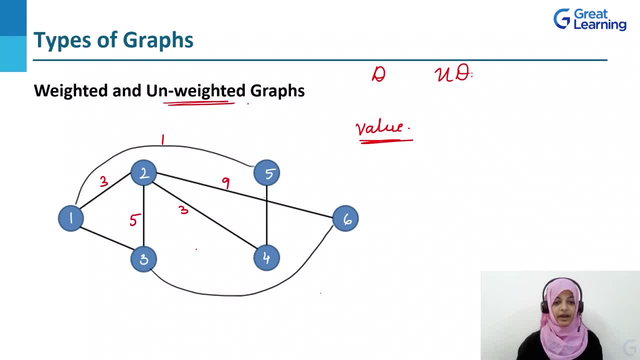 Now 2 times the number of edges, which is 7, will actually give us 14, which is exactly equal to the sum of the degrees as we've obtained in this particular graph. Now, 2 times the number of edges, which is 7, will actually give us 14, which is exactly equal to the sum of the degrees as we've obtained in this particular graph. 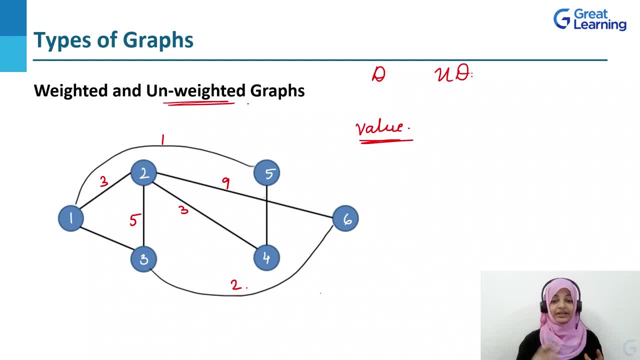 Now 2 times the number of edges, which is 7, will actually give us 14, which is exactly equal to the sum of the degrees as we've obtained in this particular graph. Now, 2 times the number of edges, which is 7, will actually give us 14, which is exactly equal to the sum of the degrees as we've obtained in this particular graph. 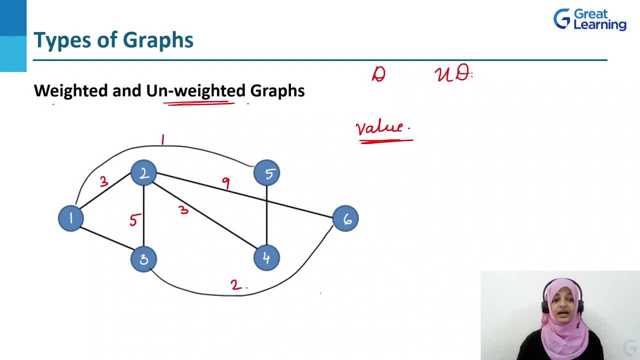 Now 2 times the number of edges, which is 7, will actually give us 14, which is exactly equal to the sum of the degrees as we've obtained in this particular graph. Now, 2 times the number of edges, which is 7, will actually give us 14, which is exactly equal to the sum of the degrees as we've obtained in this particular graph. 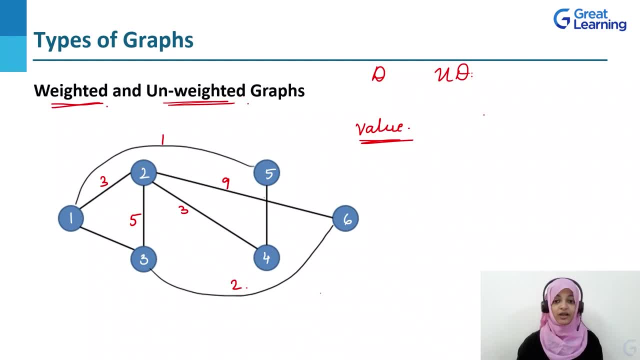 Now 2 times the number of edges, which is 7, will actually give us 14, which is exactly equal to the sum of the degrees as we've obtained in this particular graph. Now, 2 times the number of edges, which is 7, will actually give us 14, which is exactly equal to the sum of the degrees as we've obtained in this particular graph. 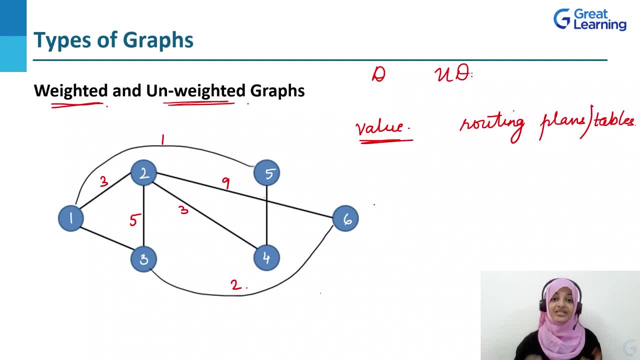 Now 2 times the number of edges, which is 7, will actually give us 14, which is exactly equal to the sum of the degrees as we've obtained in this particular graph. Now, 2 times the number of edges, which is 7, will actually give us 14, which is exactly equal to the sum of the degrees as we've obtained in this particular graph. 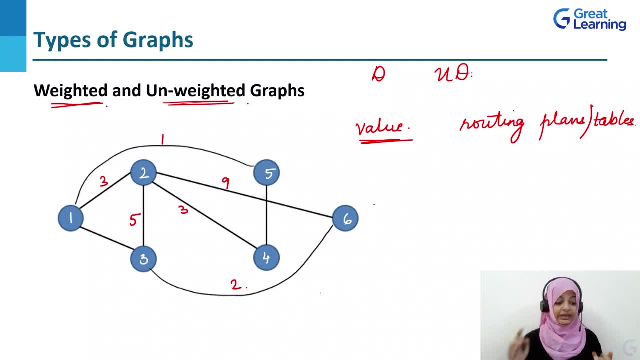 Now 2 times the number of edges, which is 7, will actually give us 14, which is exactly equal to the sum of the degrees as we've obtained in this particular graph. Now, 2 times the number of edges, which is 7, will actually give us 14, which is exactly equal to the sum of the degrees as we've obtained in this particular graph. 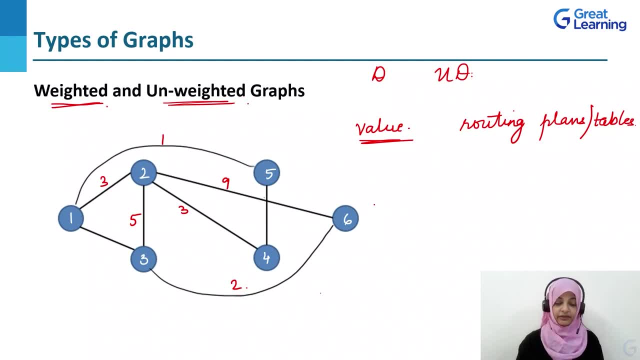 Now 2 times the number of edges, which is 7, will actually give us 14, which is exactly equal to the sum of the degrees as we've obtained in this particular graph. Now, 2 times the number of edges, which is 7, will actually give us 14, which is exactly equal to the sum of the degrees as we've obtained in this particular graph. 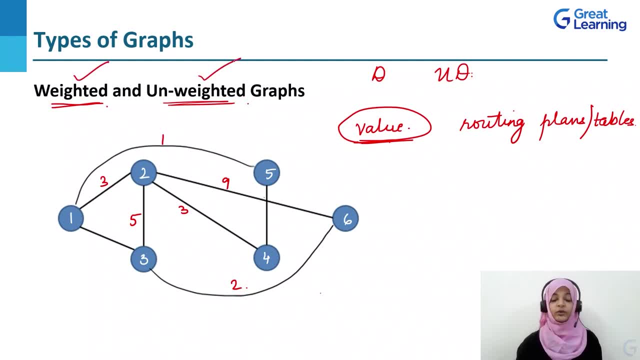 Now 2 times the number of edges, which is 7, will actually give us 14, which is exactly equal to the sum of the degrees as we've obtained in this particular graph. Now, 2 times the number of edges, which is 7, will actually give us 14, which is exactly equal to the sum of the degrees as we've obtained in this particular graph. 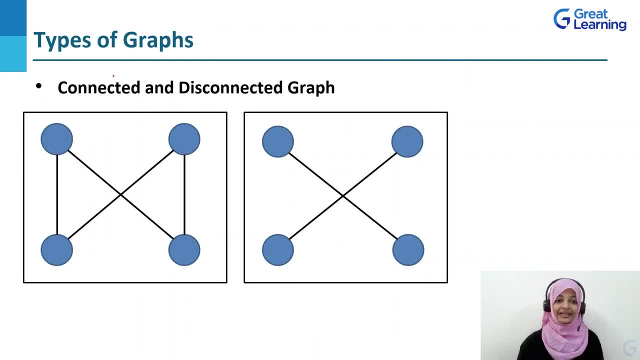 Now 2 times the number of edges, which is 7, will actually give us 14, which is exactly equal to the sum of the degrees as we've obtained in this particular graph. Now, 2 times the number of edges, which is 7, will actually give us 14, which is exactly equal to the sum of the degrees as we've obtained in this particular graph. 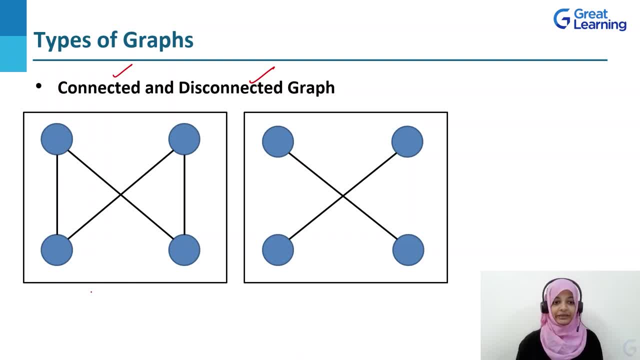 Now 2 times the number of edges, which is 7, will actually give us 14, which is exactly equal to the sum of the degrees as we've obtained in this particular graph. Now, 2 times the number of edges, which is 7, will actually give us 14, which is exactly equal to the sum of the degrees as we've obtained in this particular graph. 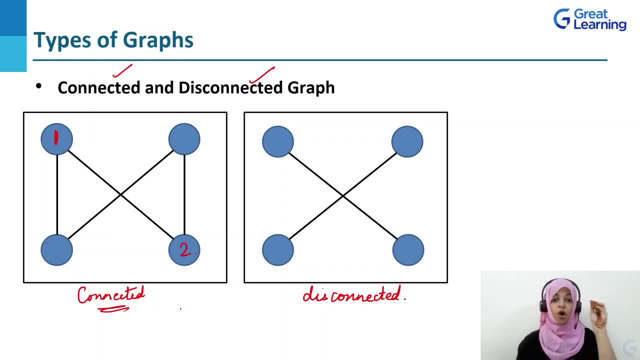 Now 2 times the number of edges, which is 7, will actually give us 14, which is exactly equal to the sum of the degrees as we've obtained in this particular graph. Now, 2 times the number of edges, which is 7, will actually give us 14, which is exactly equal to the sum of the degrees as we've obtained in this particular graph. 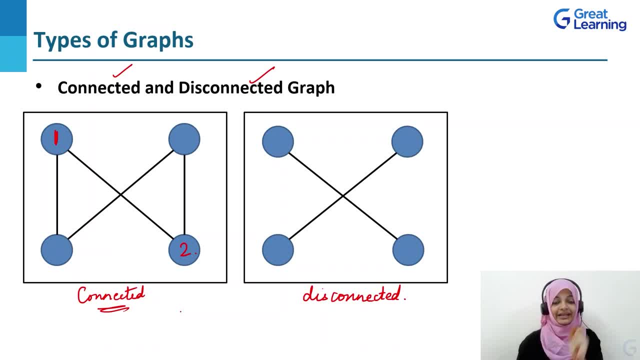 Now 2 times the number of edges, which is 7, will actually give us 14, which is exactly equal to the sum of the degrees as we've obtained in this particular graph. Now, 2 times the number of edges, which is 7, will actually give us 14, which is exactly equal to the sum of the degrees as we've obtained in this particular graph. 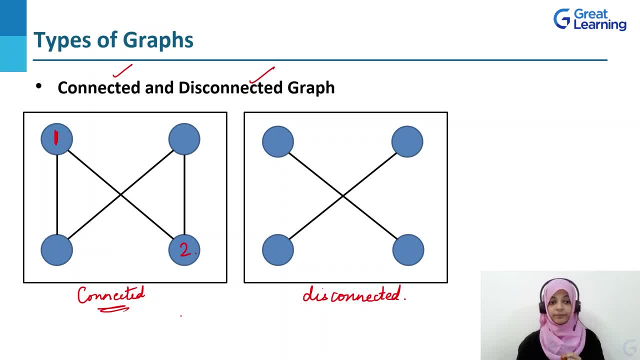 Now 2 times the number of edges, which is 7, will actually give us 14, which is exactly equal to the sum of the degrees as we've obtained in this particular graph. Now, 2 times the number of edges, which is 7, will actually give us 14, which is exactly equal to the sum of the degrees as we've obtained in this particular graph. 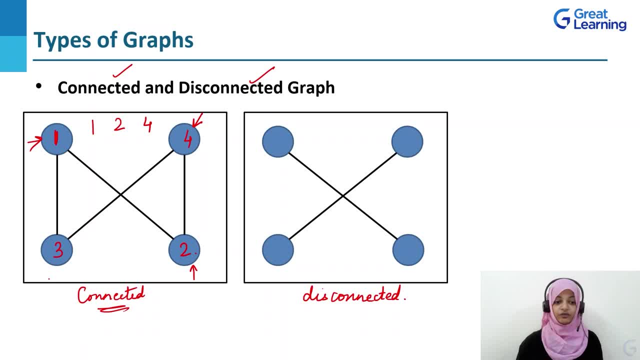 Now 2 times the number of edges, which is 7, will actually give us 14, which is exactly equal to the sum of the degrees as we've obtained in this particular graph. Now, 2 times the number of edges, which is 7, will actually give us 14, which is exactly equal to the sum of the degrees as we've obtained in this particular graph. 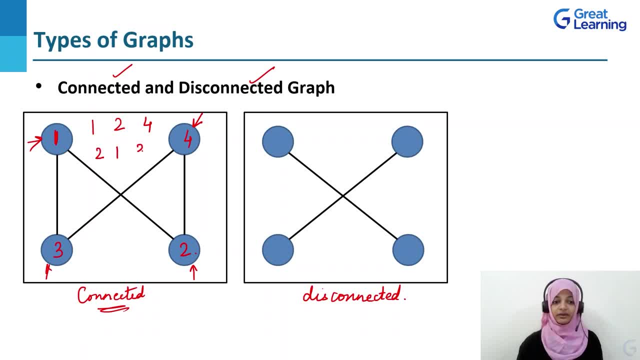 Now 2 times the number of edges, which is 7, will actually give us 14, which is exactly equal to the sum of the degrees as we've obtained in this particular graph. Now, 2 times the number of edges, which is 7, will actually give us 14, which is exactly equal to the sum of the degrees as we've obtained in this particular graph. 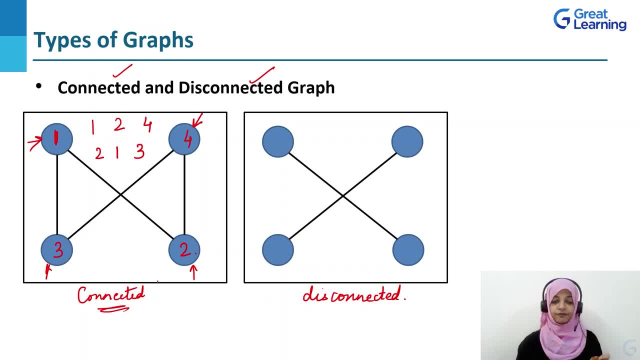 Now 2 times the number of edges, which is 7, will actually give us 14, which is exactly equal to the sum of the degrees as we've obtained in this particular graph. Now, 2 times the number of edges, which is 7, will actually give us 14, which is exactly equal to the sum of the degrees as we've obtained in this particular graph. 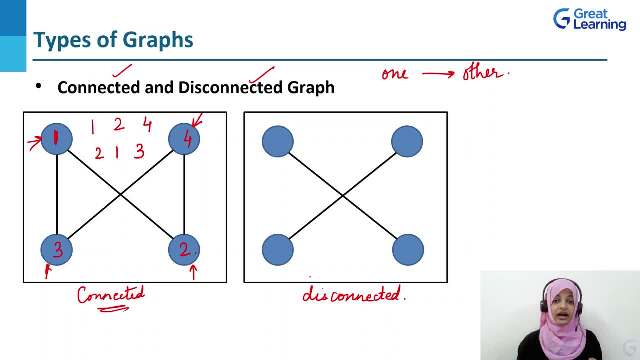 Now 2 times the number of edges, which is 7, will actually give us 14, which is exactly equal to the sum of the degrees as we've obtained in this particular graph. Now, 2 times the number of edges, which is 7, will actually give us 14, which is exactly equal to the sum of the degrees as we've obtained in this particular graph. 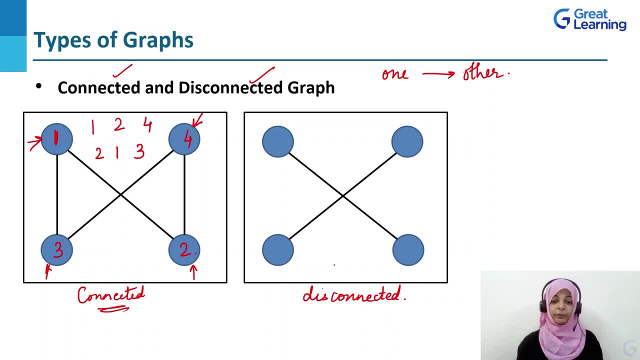 Now 2 times the number of edges, which is 7, will actually give us 14, which is exactly equal to the sum of the degrees as we've obtained in this particular graph. Now, 2 times the number of edges, which is 7, will actually give us 14, which is exactly equal to the sum of the degrees as we've obtained in this particular graph. 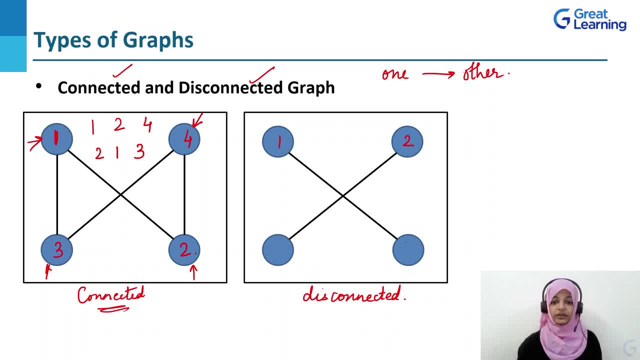 Now 2 times the number of edges, which is 7, will actually give us 14, which is exactly equal to the sum of the degrees as we've obtained in this particular graph. Now, 2 times the number of edges, which is 7, will actually give us 14, which is exactly equal to the sum of the degrees as we've obtained in this particular graph. 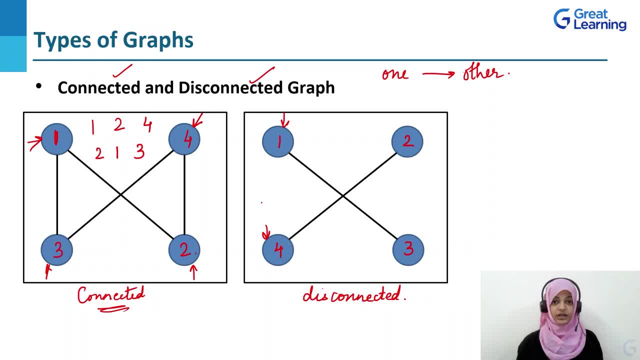 Now 2 times the number of edges, which is 7, will actually give us 14, which is exactly equal to the sum of the degrees as we've obtained in this particular graph. Now, 2 times the number of edges, which is 7, will actually give us 14, which is exactly equal to the sum of the degrees as we've obtained in this particular graph. 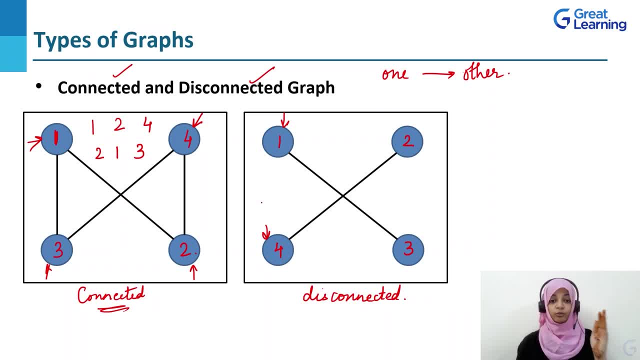 Now 2 times the number of edges, which is 7, will actually give us 14, which is exactly equal to the sum of the degrees as we've obtained in this particular graph. Now, 2 times the number of edges, which is 7, will actually give us 14, which is exactly equal to the sum of the degrees as we've obtained in this particular graph. 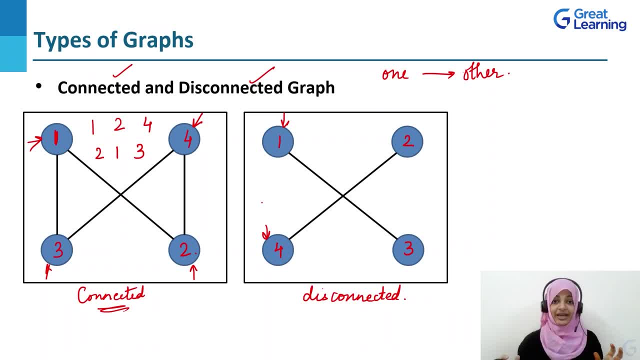 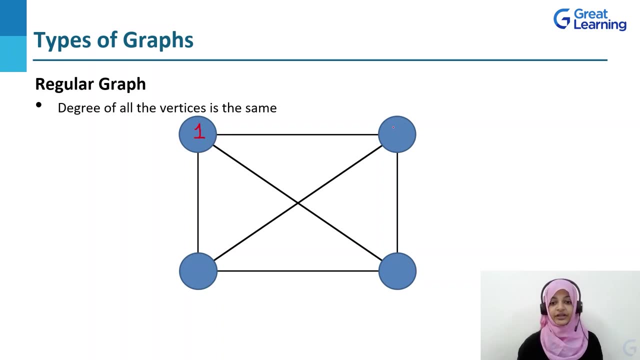 Now 2 times the number of edges, which is 7, will actually give us 14, which is exactly equal to the sum of the degrees as we've obtained in this particular graph. Now, 2 times the number of edges, which is 7, will actually give us 14, which is exactly equal to the sum of the degrees as we've obtained in this particular graph. 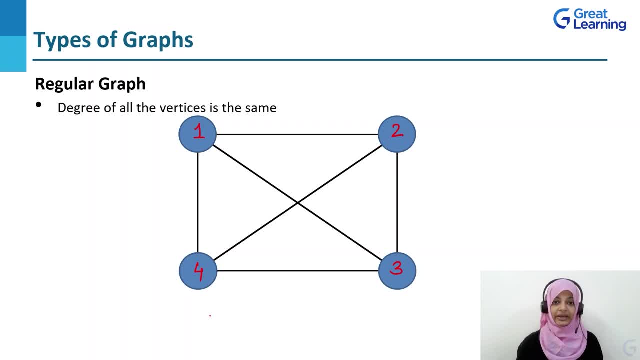 Now 2 times the number of edges, which is 7, will actually give us 14, which is exactly equal to the sum of the degrees as we've obtained in this particular graph. Now, 2 times the number of edges, which is 7, will actually give us 14, which is exactly equal to the sum of the degrees as we've obtained in this particular graph. 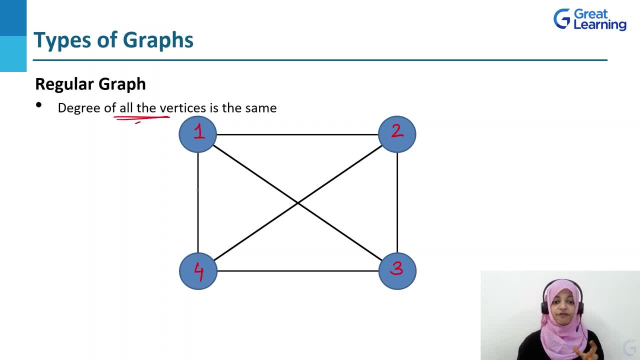 Now 2 times the number of edges, which is 7, will actually give us 14, which is exactly equal to the sum of the degrees as we've obtained in this particular graph. Now, 2 times the number of edges, which is 7, will actually give us 14, which is exactly equal to the sum of the degrees as we've obtained in this particular graph. 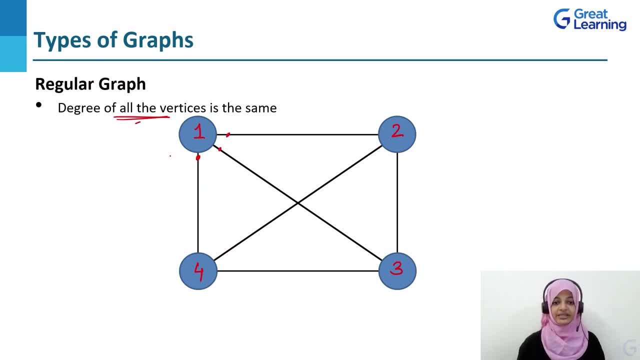 Now 2 times the number of edges, which is 7, will actually give us 14, which is exactly equal to the sum of the degrees as we've obtained in this particular graph. Now, 2 times the number of edges, which is 7, will actually give us 14, which is exactly equal to the sum of the degrees as we've obtained in this particular graph. 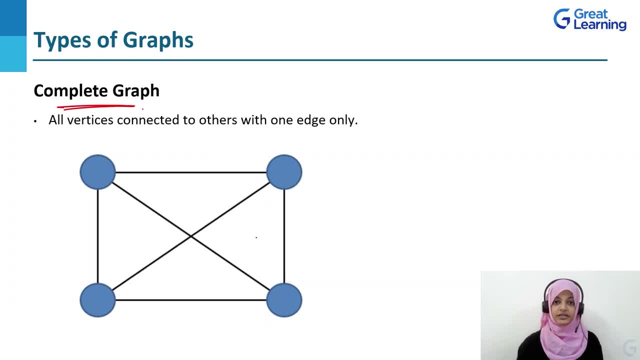 Now 2 times the number of edges, which is 7, will actually give us 14, which is exactly equal to the sum of the degrees as we've obtained in this particular graph. Now, 2 times the number of edges, which is 7, will actually give us 14, which is exactly equal to the sum of the degrees as we've obtained in this particular graph. 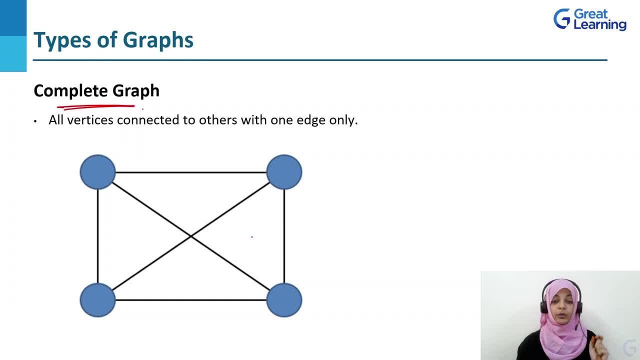 Now 2 times the number of edges, which is 7, will actually give us 14, which is exactly equal to the sum of the degrees as we've obtained in this particular graph. Now, 2 times the number of edges, which is 7, will actually give us 14, which is exactly equal to the sum of the degrees as we've obtained in this particular graph. 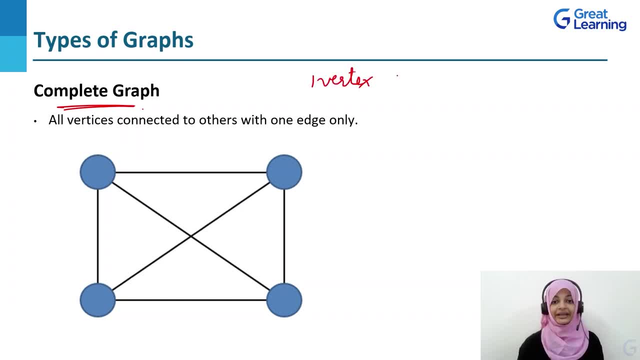 Now 2 times the number of edges, which is 7, will actually give us 14, which is exactly equal to the sum of the degrees as we've obtained in this particular graph. Now, 2 times the number of edges, which is 7, will actually give us 14, which is exactly equal to the sum of the degrees as we've obtained in this particular graph. 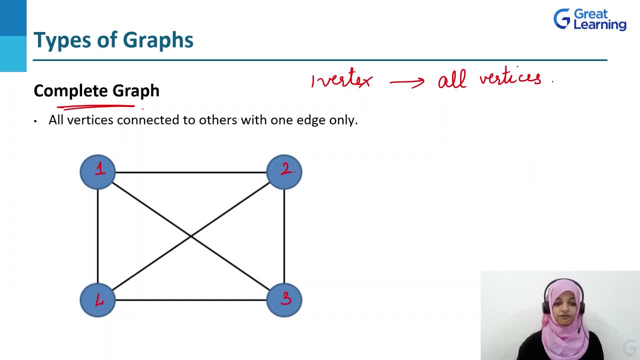 Now 2 times the number of edges, which is 7, will actually give us 14, which is exactly equal to the sum of the degrees as we've obtained in this particular graph. Now, 2 times the number of edges, which is 7, will actually give us 14, which is exactly equal to the sum of the degrees as we've obtained in this particular graph. 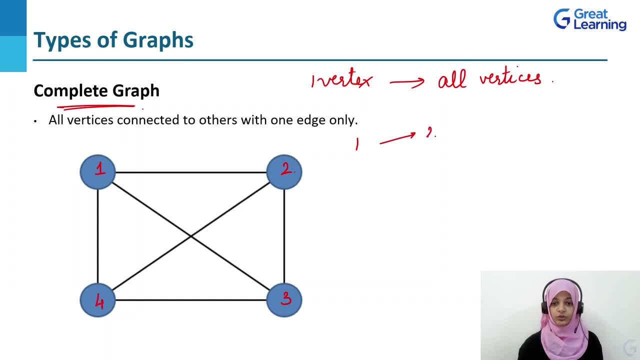 Now 2 times the number of edges, which is 7, will actually give us 14, which is exactly equal to the sum of the degrees as we've obtained in this particular graph. Now, 2 times the number of edges, which is 7, will actually give us 14, which is exactly equal to the sum of the degrees as we've obtained in this particular graph. 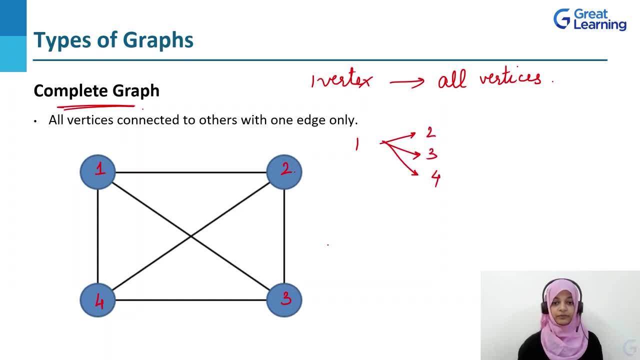 Now 2 times the number of edges, which is 7, will actually give us 14, which is exactly equal to the sum of the degrees as we've obtained in this particular graph edges to vertex 1, vertex 2 and vertex 3.. This means that each and every vertex that is a part 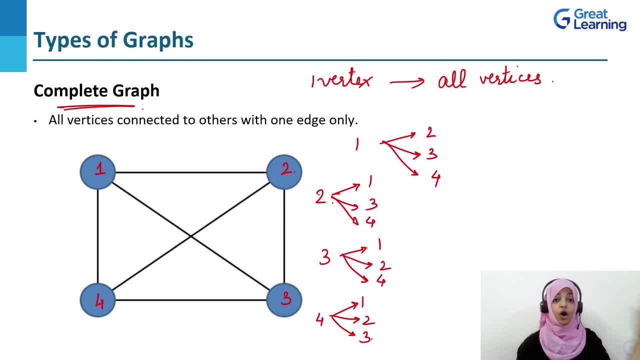 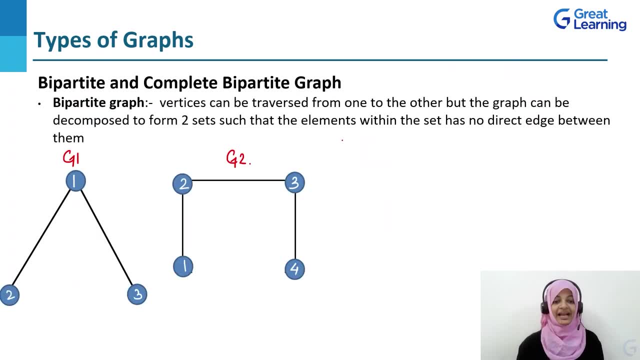 of the graph is directly connected to all of the other vertices that are a part of the exact same graph. Such graphs are known as complete graphs. Next, let's look at the last concept that we have in our types of graphs. This is the bipartite and the complete bipartite graph. Now, in order to 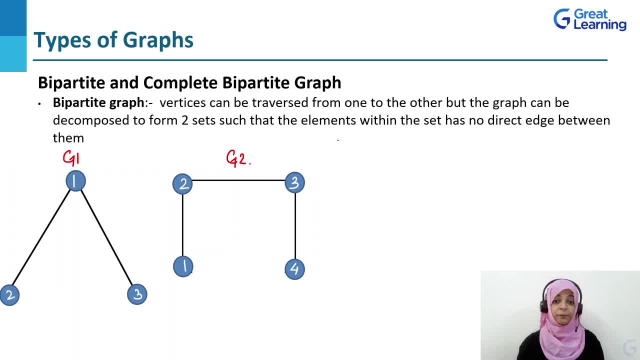 understand what complete bipartite is, we first need to understand what a bipartite graph is. Now, a bipartite graph is one wherein the vertices can be traversed from one vertex to the other, But we can split up this particular graph into two sets of vertices such that there is no set. 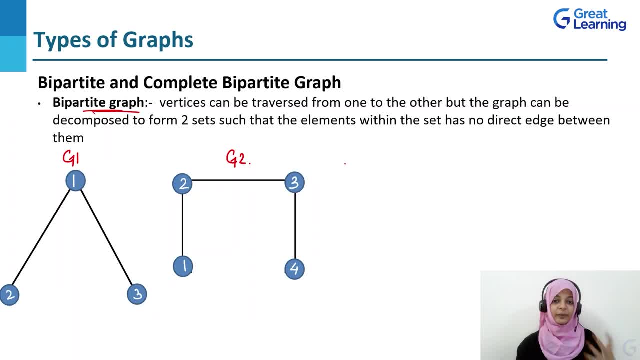 which has a direct connectivity between them. Let me explain this further with the example of this G1 graph. We are able to traverse from vertex 2 to vertex 3.. Also, we are able to traverse from vertex 2 to vertex 1 and vertex 1 to vertex 3.. This means that this particular graph is a connected graph. 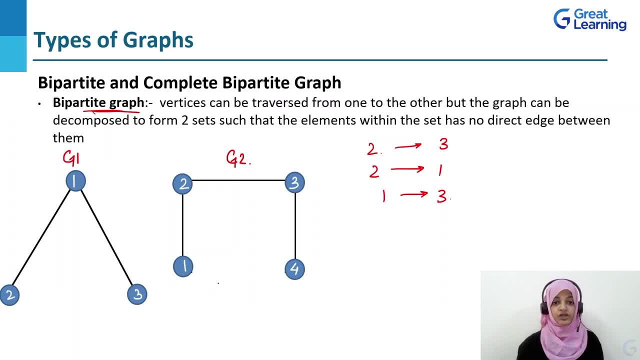 right. There is no disconnectivity between this graph. So our first condition is complete: that the vertices can be traversed from one to the other. Next look at the second part of the definition of the bipartite graph. We are able to traverse from vertex 2 to vertex 3.. So our 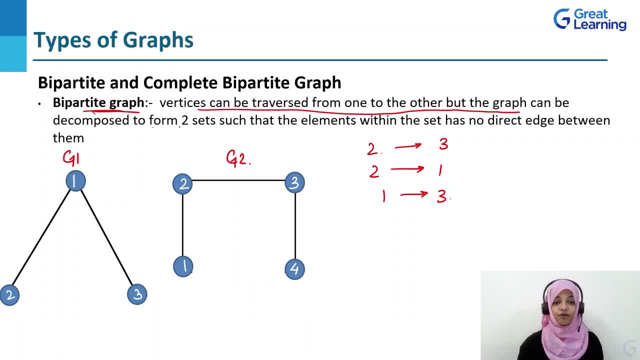 first condition is complete: that the vertices can be traversed from one to the other. Next, look at the definition of the bipartite graph. In the next part we actually need to form two sets with the vertices that are a part of the graph. So for our graph G1, let us create two sets. Say, for example: 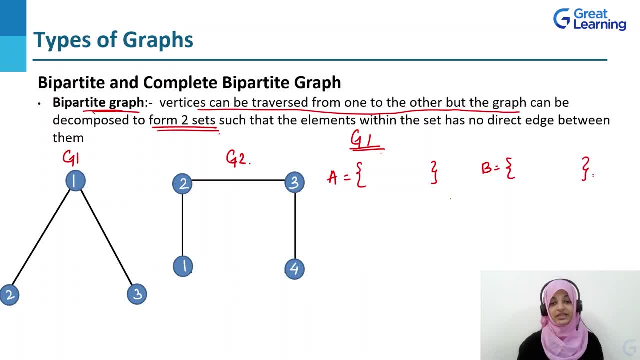 set A and set B, And the method in which these two sets have to be set up is very simple. They've said that both of these sets are supposed to contain vertices, But the vertices should be split up in such a way that they are not separated from each other. So let's say that we have a set of 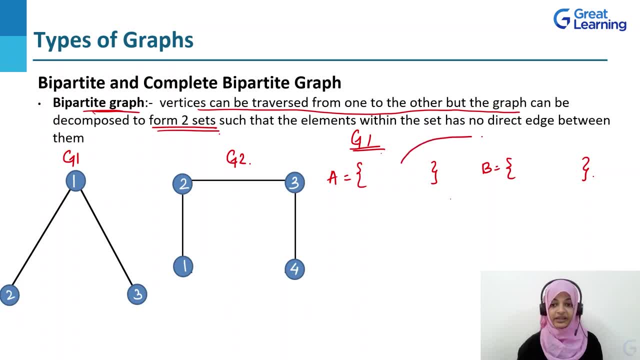 in such a way that they are not separated from each other. So let's say that we have a set of. there is connectivity between the vertices across set, but no connectivity between the elements of the set. So here they are talking about direct connectivity. If there exists a direct 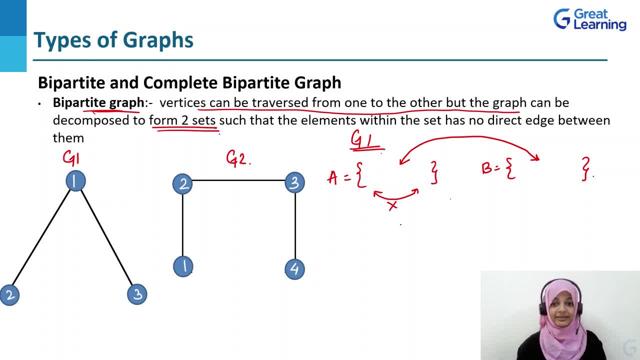 edge between the two elements then existing, they should exist in two different sets And if they are existing in the exact same set, there should be no direct edge between them. so if we look at graph g1, then we can put 2 and 3 in one particular set. 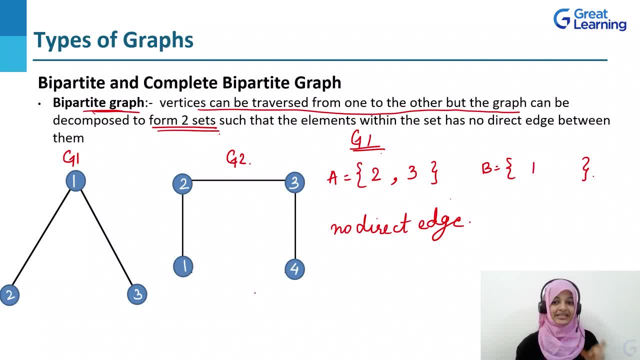 and vertex 1 in a complete different set. let us see if this actually satisfies our bipartite condition. so if we look at this particular example, there is a direct edge between vertex 2 and vertex 1, so it is across the two sets. again we've got connectivity between. 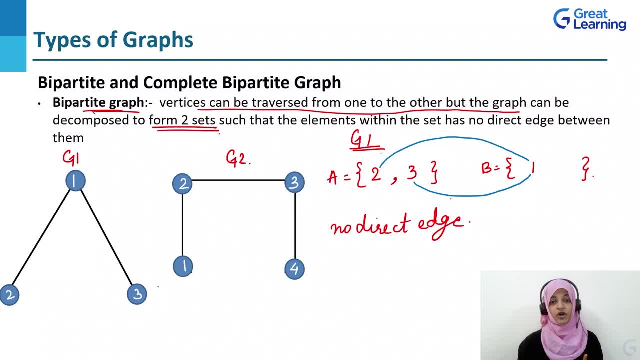 vertex 3 and vertex 1. again, it is across the two sets. but is there any connectivity between vertex 2 and vertex 3? no, in our graph there is no connectivity between vertex 2 and vertex 3. by connectivity here i'm talking about a direct edge between the two vertices. 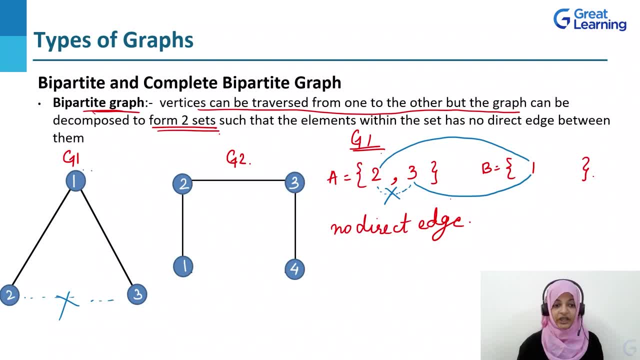 since this is not the case, that means that this particular graph can be decomposed in such a manner that two sets are formed, such that the elements within the set have no direct edge between them, but there are edges across the 2 sets, right? let us understand this. 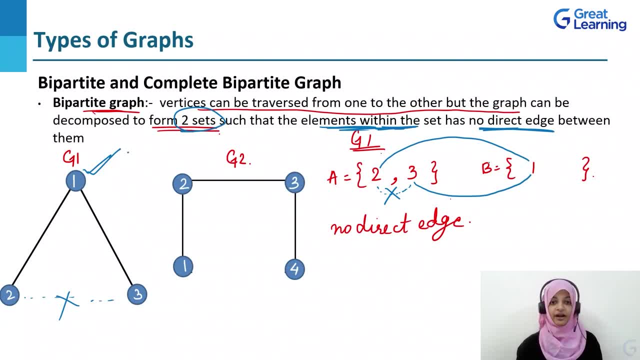 further with the other example given here, namely graph2 or g2. now look at graph g2. Graph G2 actually has four vertices in it. Now let us decompose these vertices in such a manner that we have two separate sets. We can put up vertex 1 and vertex 3 into one set. 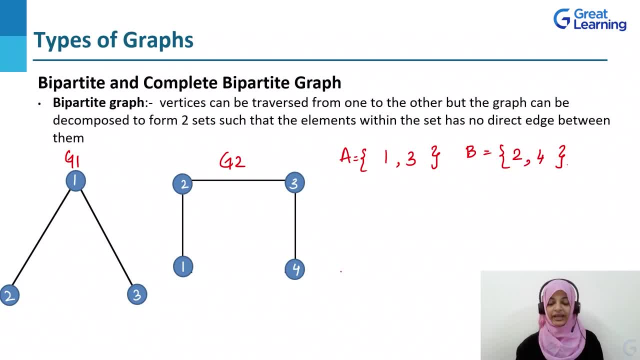 And we can put up vertex 2 and vertex 4 in another set. Observe this very closely. We have a direct edge between vertex 1 and vertex 2, which is cross-set in this case. Again, we have a direct edge between vertex 2 and vertex 3, which is again cross-set. 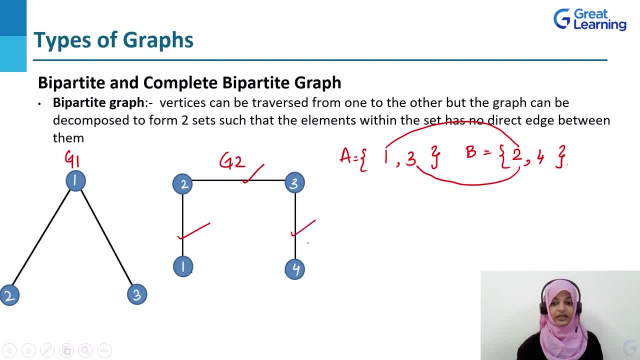 Lastly, we have a direct edge between vertex 3 and vertex 4.. This is again cross-set. As you can see, we have no direct edges between vertex 1 and vertex 3, which are a part of the equation, And similarly we have no connectivity direct edge, that is, between vertex 2 and vertex 4,. 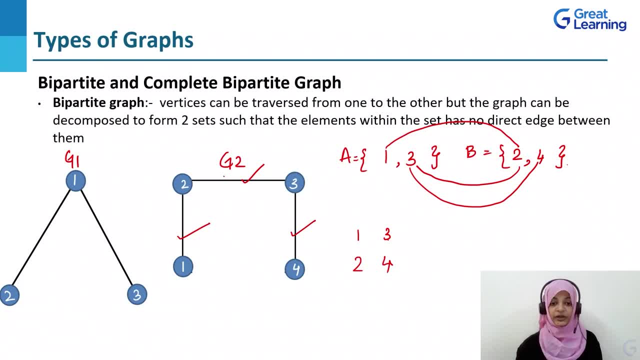 which is again a part of the same set. This means that this particular graph is a bipartite graph, because we are able to traverse from vertex 1 to any of the other vertices, but there are no direct edges within the decomposed set. vertices right. 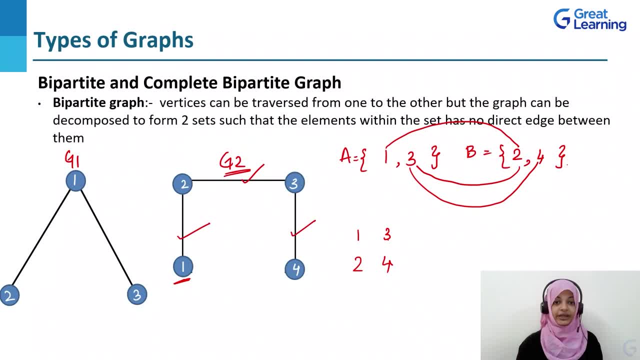 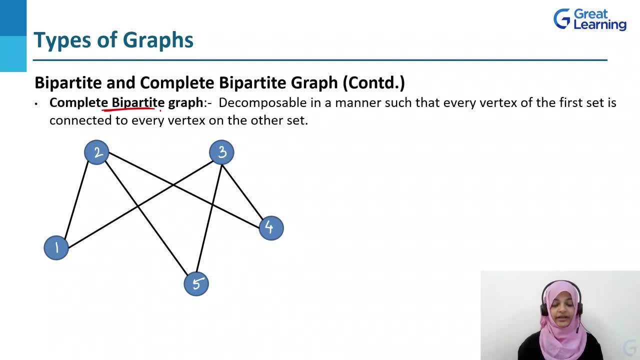 So this is how bipartite graphs are activated. Lastly, let us look into the complete bipartite graph. Now, what is a complete bipartite graph? It is a graph that is actually a combination of the concepts of bipartite and complete. 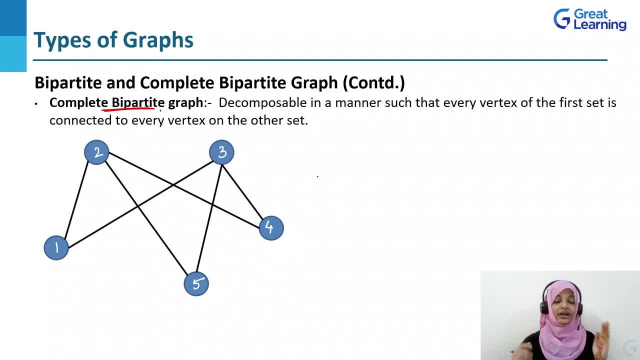 graphs. So in complete graphs, we've said a complete graph is one which is actually set up in such a manner that we are able to have direct edges from one vertex to all the other vertices that are a part of the graph. And in bipartite graphs, we know we need to have vertices set up in such a manner that. 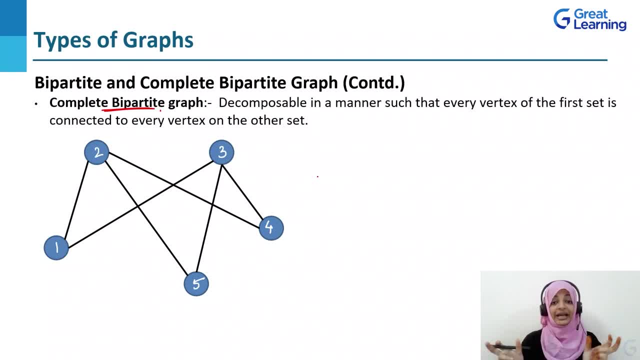 we are decomposing the graph into two sets, such that inter-set edges exist, but intra-set edges do not exist, And here we have a combination of both of those concepts. So if we look at this particular graph, we can decompose this graph into two sets. 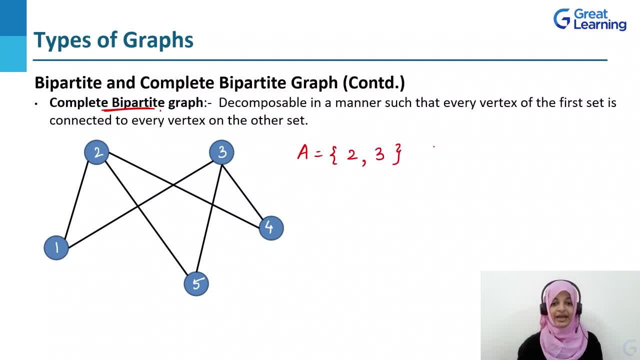 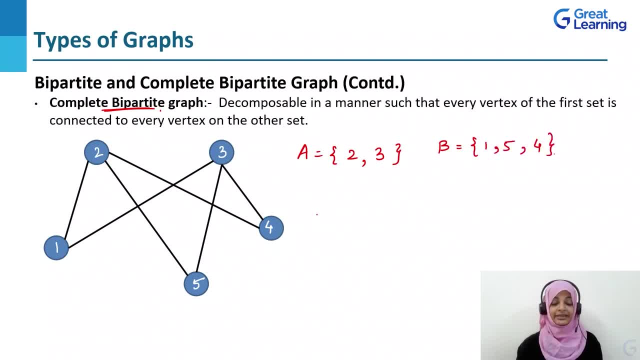 They are vertex 1,, 5, and 4.. Now observe these two sets. We have clearly decomposed this particular graph into a bipartite form. That is because there are inter-set edges, but there are NO edges between the elements. 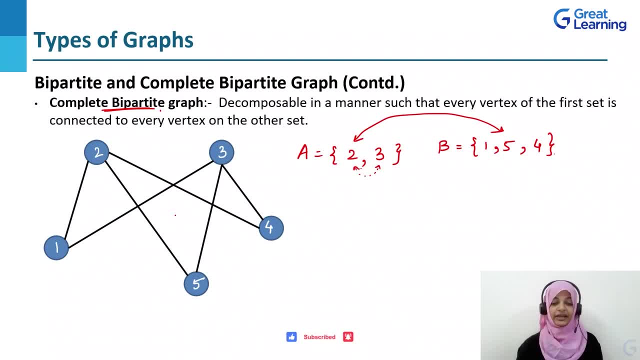 of any single set. Please observe this carniffer- starve the graph. So again, this is a Bipartite Graph. Now let us look at the complete portion of this particular type of graph. So here what we can see is if we take up any one element from any one set, 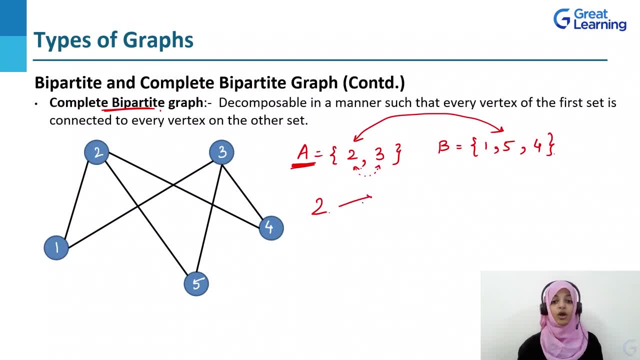 this particular element is connected with all of the elements of the second set. So if we look here, we have an edge between 2 and 1, an edge between 2 and 5 and an edge between 2 and 4.. Similarly, if we take the other element of the set, 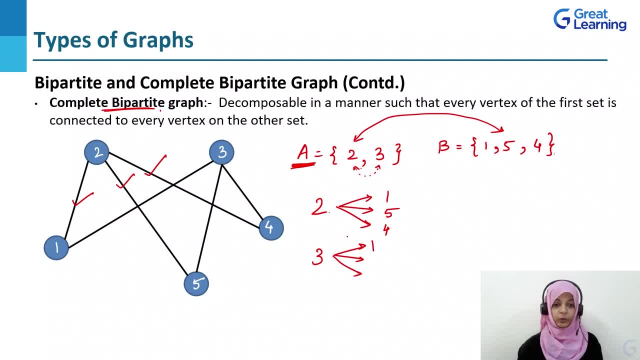 we again have edges going from 3 to 1,, 3 to 5 and 3 to 4.. Similarly, if we take the other set here, namely 1,, 5 and 4, we have edges going from 1 to 2 and 3, edges going from 5 to 2 and 3. 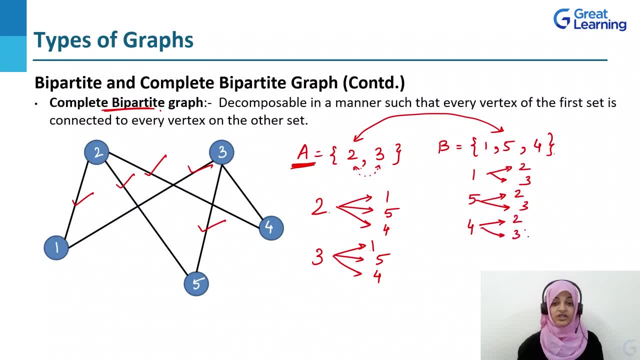 and edges going from 4 to 2 and 3.. So here each of the elements of one set are connected with all of the elements of the second set. So these are the elements of the other set. So this is what a complete bipartite graph is. 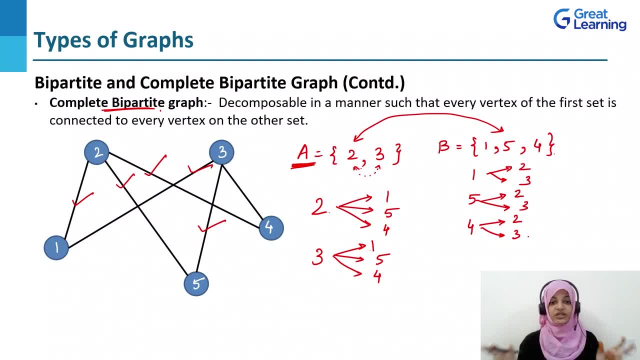 One in which the vertices can be decomposed in such a manner that there are only inter-set edges existing and no intra-set edges existing and, apart from that, each and every vertex of one set is connected with all of the vertices of the other set. 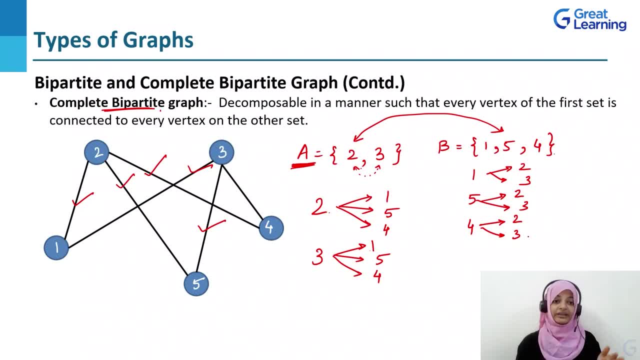 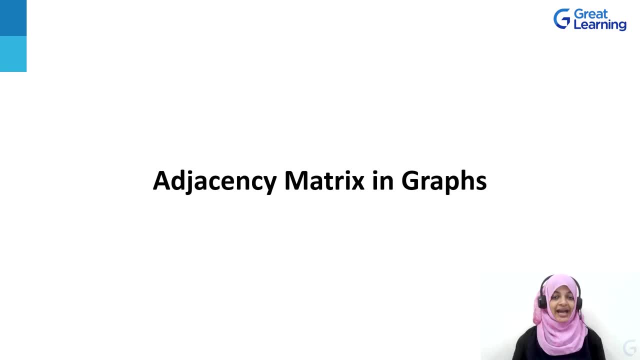 So these are all of the various graphs that we have taken up from this set. Now let us look at the next set we commonly see in graph theory. lastly, let us quickly look into adjacency matrix and how it is actually used in graphs. so adjacency matrix is actually a chart which looks like: 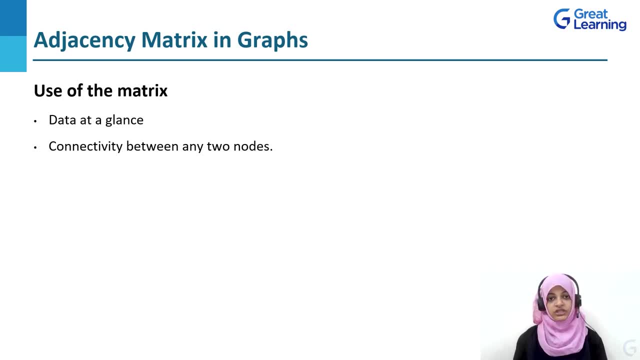 a complete matrix. this means that it has a particular set of rows and a particular set of columns. the basic use of adjacency matrix is that it gives us an analysis of all of the data about the graph. in a glance, we understand what is the connectivity between any two nodes. 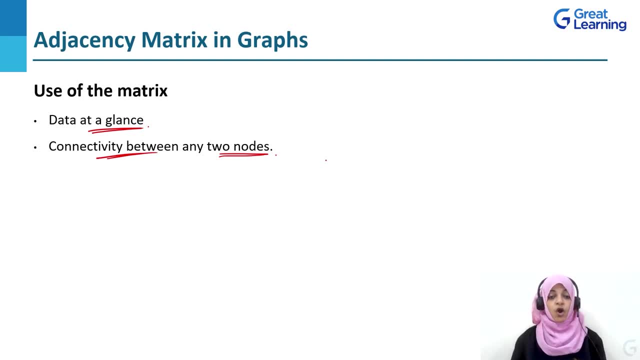 or the connectivity between the node and itself. all of these can be identified at one glance of the adjacency matrix. so the adjacency matrix is actually utilized for these kind of properties in any use case where you need to find the shortest path. this means that in most of those 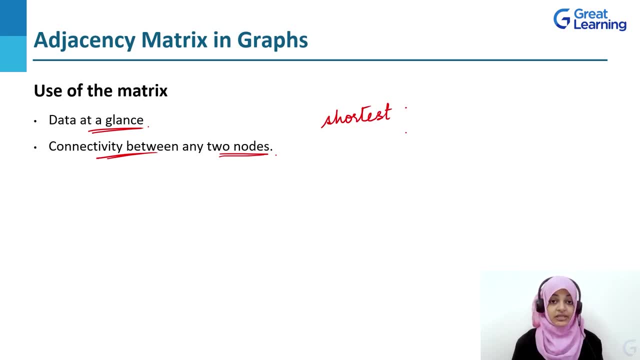 algorithms which actually help us find the shortest path, such as dx, m, z, etc. algorithm. for example, we would use an adjacency matrix. other applications where we use adjacency matrix is network analysis, finding out whether a graph is isomorphic and not, etc. right, so let 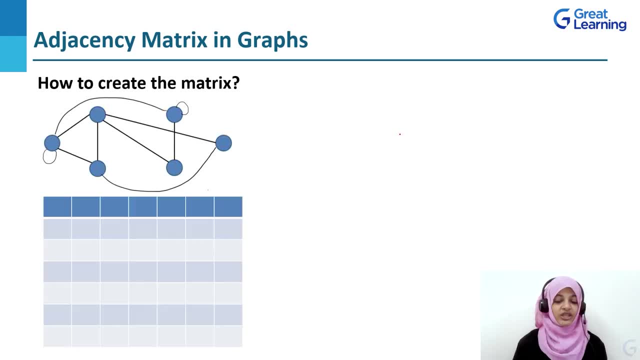 us quickly look at what the adjacency matrix actually is. so the adjacency matrix is actually a combination of the various edges and how those edges are related from one vertex to the other. the adjacency matrix always has a v into v size. this means that it always has a number. 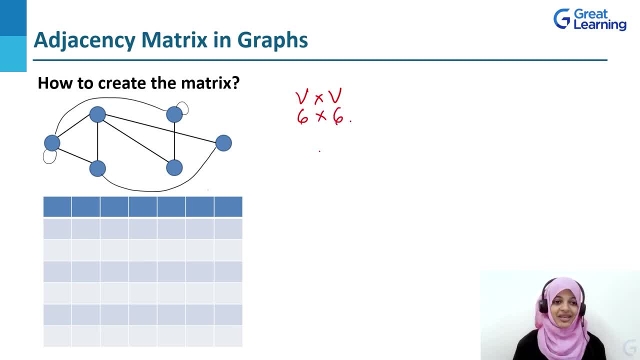 of vertices into a number of vertices size. as you can see, here we've got six vertices right, so all of these vertices are actually supposed to be set up in this table in such a manner that the first column and the first row all have all of the vertices listed on them. 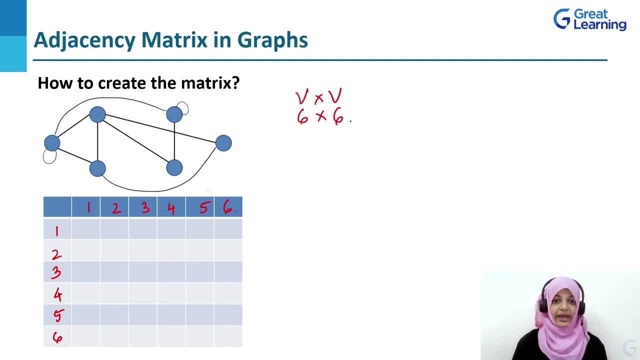 next, what do we do? We identify where edges are moving from and from where they are moving. So the initiation vertex and the destination vertex have to be identified. So let our graph be numbered in this particular way. Let the vertices be from 1 to 6.. We need to identify whether there are edges. 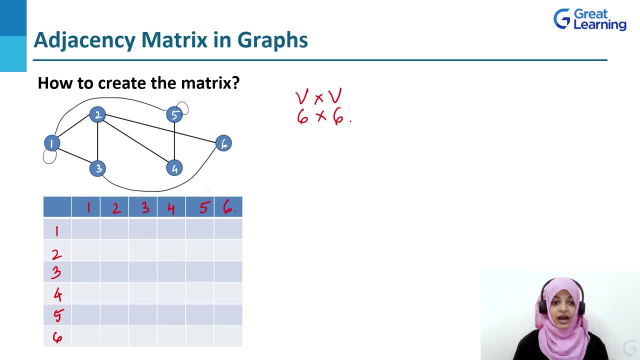 passing from one vertex to the other. If there are, then we write a value of 1 in that particular cell. If there are no edges going from one vertex to the other, we'll write a 0.. So let us see how this particular graph can be translated into an adjacency matrix. First we look at this particular 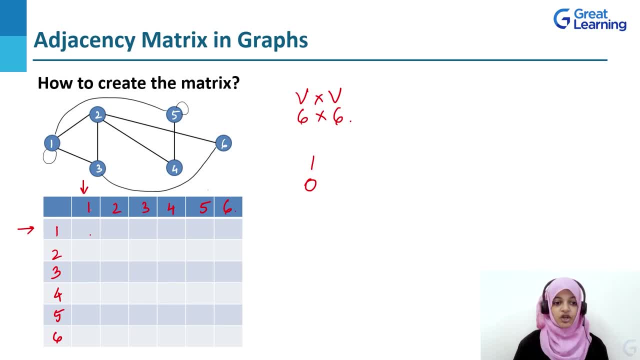 cell. This cell is in the first row and the first column. This means that it is actually asking us whether there is an edge from 1 to 1.. So let's say that there is an edge from 1 to 1.. So let's. 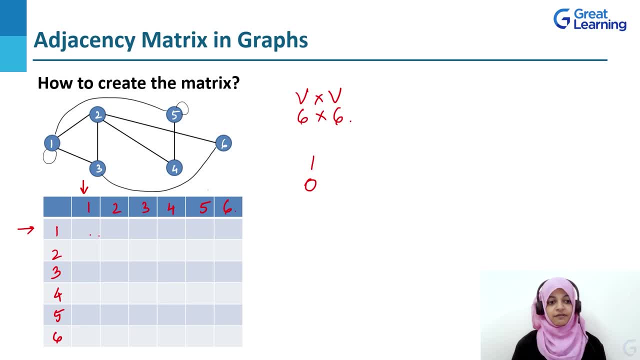 say that there is an edge from 1 to 1.. An edge from a particular vertex to itself is only possible in the case of a loop. Since we do have a loop here, we would write 1, indicating that such an edge actually exists. Next we look at 1, 2.. This means that it is asking us if there is an edge. 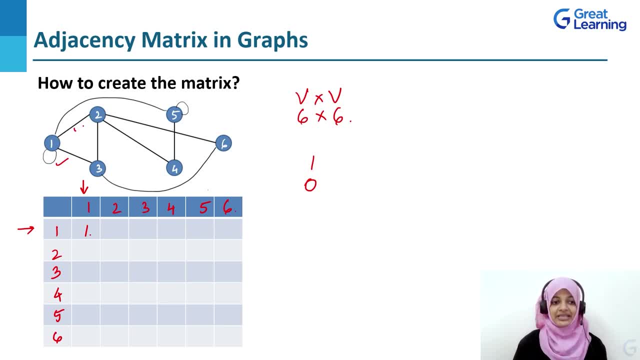 that goes from vertex 1 to vertex 2.. As we can see, such an edge actually exists. Thus, we'll write a 1 here. Next we've got 1, 3. This means that it is asking us whether there is an edge. 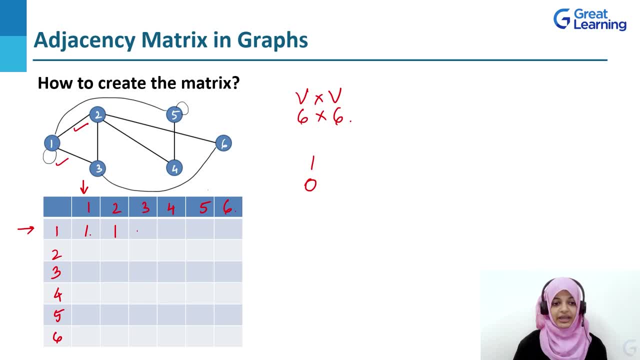 going from 1 to 3, and such an edge exists. Next we've got 1, 4.. There is no edge directly going from vertex 1 to vertex 4.. So this particular edge does not exist. Next we've got an edge going from: 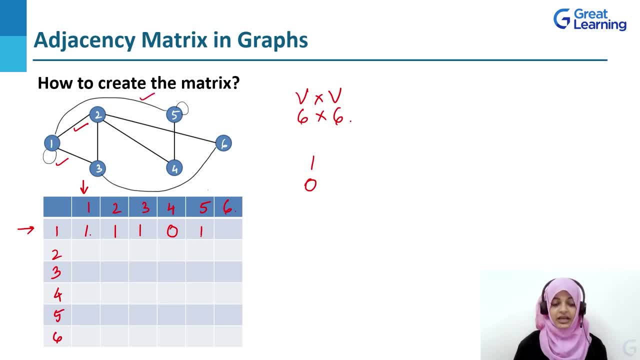 vertex 1 to vertex 5, and such an edge exists. Lastly, we've got no edge going from vertex 1 to vertex 6, and that is why no such edge exists. So in this case we'll write 1, 2.. This means that 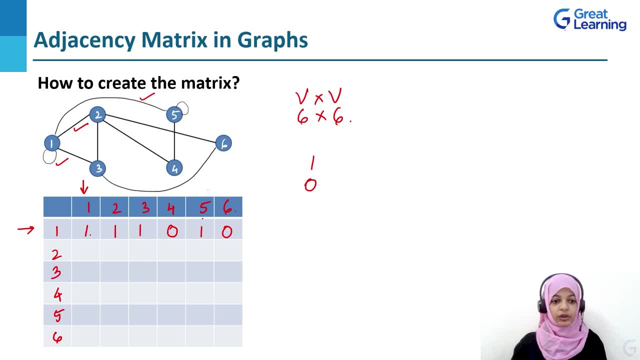 this particular manner we can find out all the other rows also. Let us do the second vertex row. Is there an edge between the second vertex and the first? Yes, as per our diagram, we can see that there is an edge between the second and the first vertex. So we get a 1 here. Next we check. 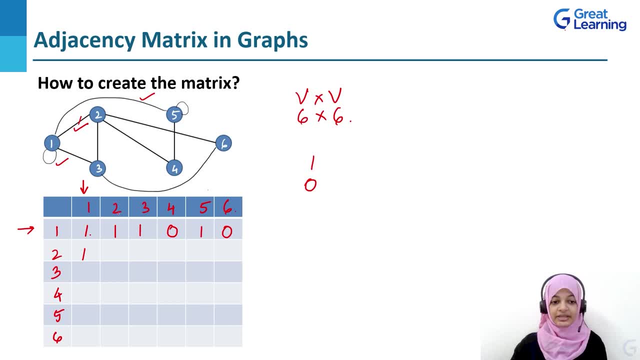 whether there are any edges between the second and the second vertex itself. As we can see, there is no loop of this particular kind, So here we would get a 0.. Similarly, between 2 and 3, we've got another edge here, So here again we'll get a 1.. Next, 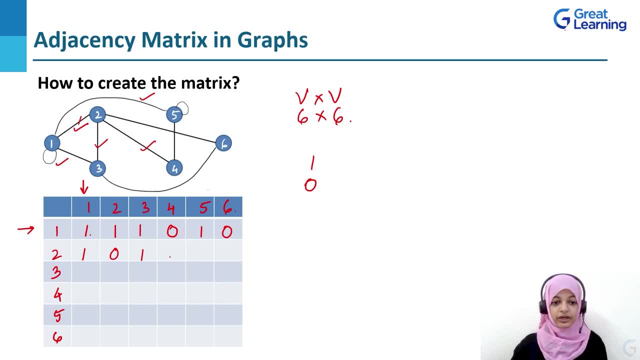 between 2 and 4, we've got an edge, So here we've got 1. again, Between 2 and 5, there are no direct edges. As a result, here we'll put up 0.. And between 2 and 6, we do have a direct edge, and 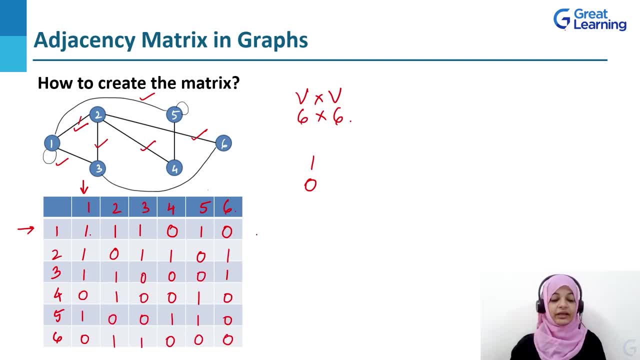 that is why we'll get a 1 here. So if we look at our complete table or adjacency matrix, then this is what it looks like. Now, as you can see, here there are actually rows and columns having the exact same values. So if you look at the row containing all of the data, 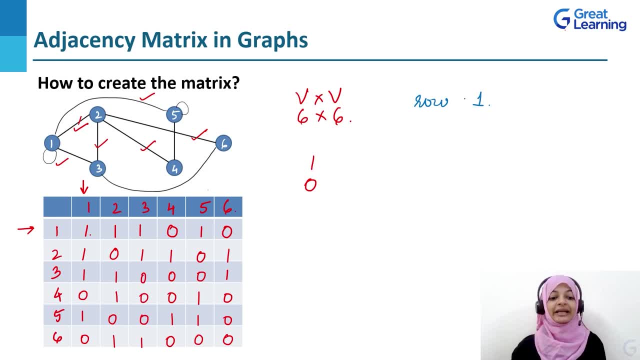 for vertex 1, you will see that this is exactly equal to the column containing the data for vertex 1.. That is because it is the exact same vertex that we're talking about. So the adjacency matrix is actually a square table in which we set up all of our required vertices and we map out. 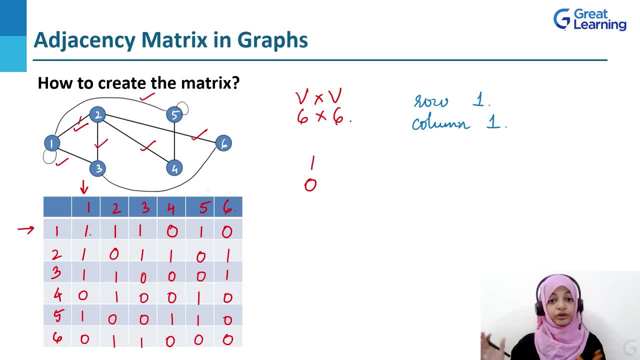 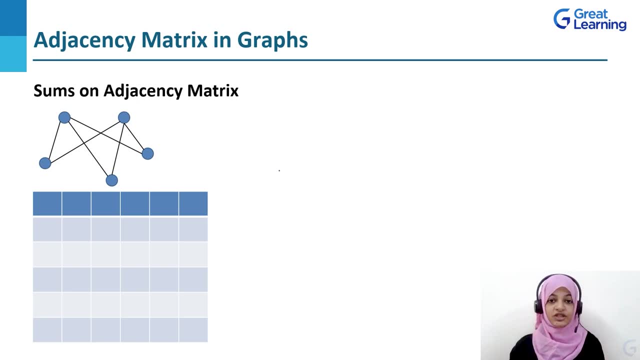 the various edges that have existed or do not exist between the given vertices. Next, let us solve two sums on adjacency matrix to understand exactly how this particular matrix works. Please keep in mind that actually the adjacency matrix can be formed for different types of graphs And in these different types of graphs we've got directed and undirected. 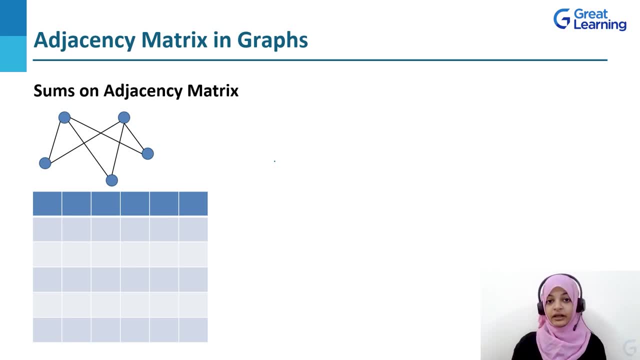 graphs. So, based upon whether the graph is a directed graph or undirected graph, there is a slight difference between the adjacency matrix that we actually form. Let us understand that with an example. Consider this particular example given here. So here we'll be taking this example. 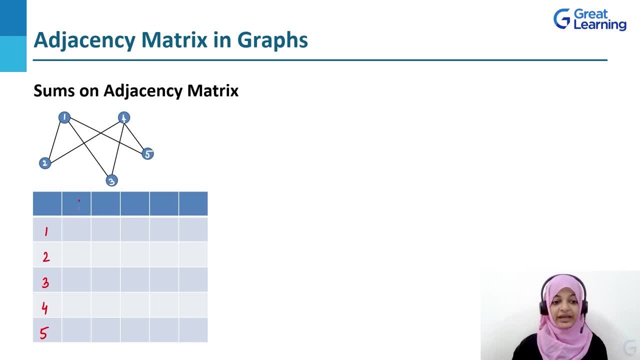 with vertices 1,, 2,, 3,, 4 and 5.. And similarly, we will take vertices 1,, 2,, 3, 4 and 5 above also. Now, what do we have to do here? Similar to the example we've seen previously, even here. 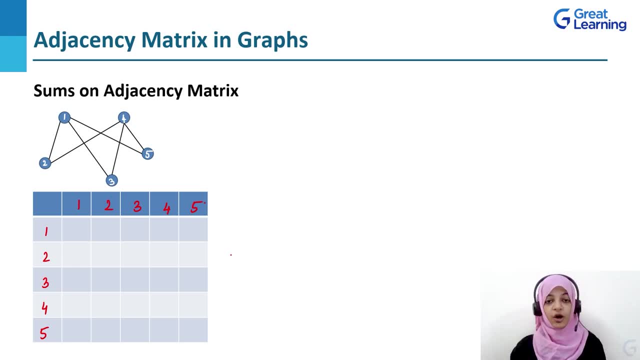 we need to find out whether an edge exists or does not between two given vertices. So what are we going to do first? First, we're going to check for vertex 1.. Vertex 1 does not have any edge width. This vertex does not have any edge width. So what are we going to do here? 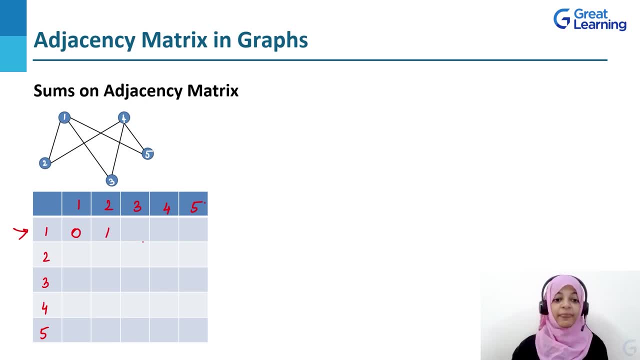 Let us find out what is the distance between vertices 1 and vertex 2.. And similarly we will take vertices 1,, 2,, 3,, 4 and 5 above. also itself, Vertex 1 has an edge with 2, vertex 1 has an edge with 3, vertex 1 has no edges. 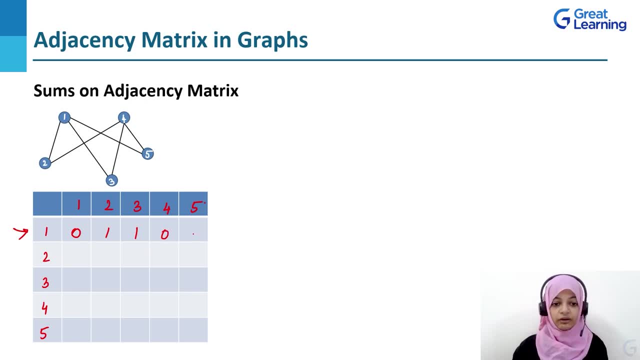 with 4 and vertex 1 has an edge with 5.. Similarly, vertex 2 has an edge with 1, vertex 2 has no edges with itself. vertex 2 has no edges with vertex 3, vertex 2 has one edge with. 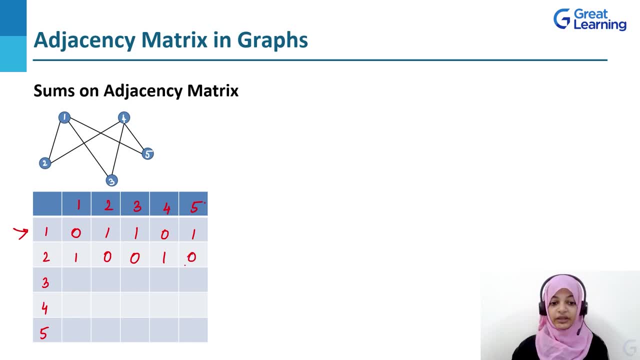 vertex 4, and vertex 2 has no edges with vertex 5.. Next let's look at vertex 3.. Vertex 3 has one edge with vertex 1, zero edges with vertex 2, zero edges with itself, one edge with vertex 4 and zero edges with vertex 5.. Similarly, vertex 4 has zero edges with vertex. 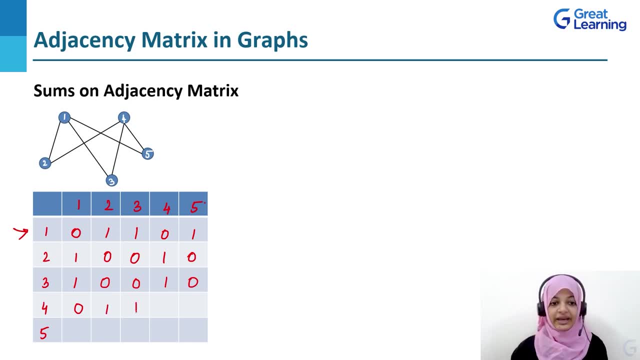 1, one edge with vertex 2, one edge with vertex 3, zero edges with itself and one edge with vertex 5.. Lastly, vertex 5 has one edge with vertex 1, zero edges with vertex 2, zero edges with vertex 3, one edge with vertex 4 and zero edges with itself. So our adjacency, 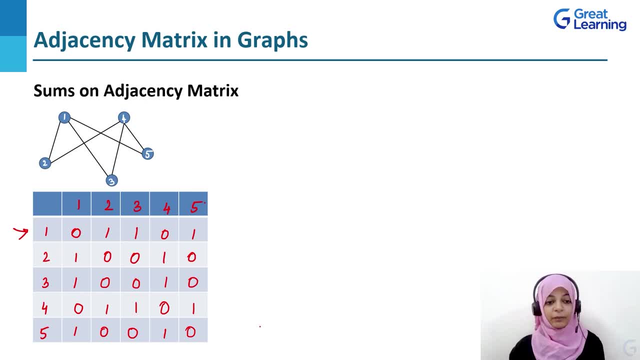 matrix was very clearly made here and also very quickly made here. As you can see, we didn't really differentiate between going from vertex 1 to 2 or going from vertex 2 to 1.. Since these parameters are different, we didn't really differentiate between going from. 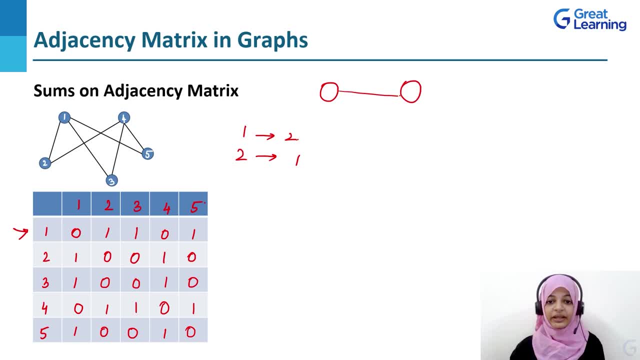 vertex 1 to vertex 3.. In case, for example, if vertices this particular edge in both the places, activity in both places, for example editping, is belonged to vertex1 to vertex3, we didn't really differentiate between going from vertex 2 to vertex 3 until we were 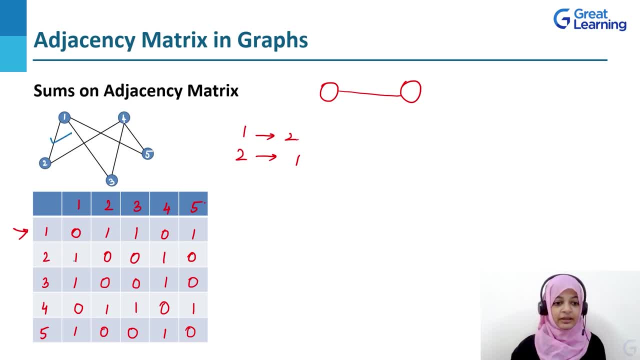 at theending point. So we didn't really differentiate between when going from other vertices. object: geometry�: всех in both the places, so that we could see both the different edges. In our example thisυτhe one particular edgeiint in both the places. 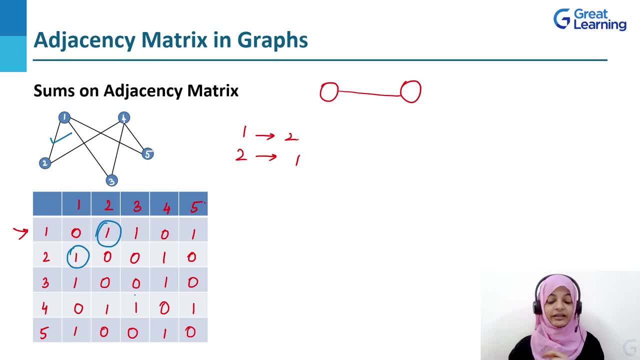 So this is actually one of the major differences between undirected and directed graphs. In the undirected graphs, this one singular edge will be mentioned in two places, because in one case we are considering the edge between vertex 1 and 2.. In the other case, manifests. 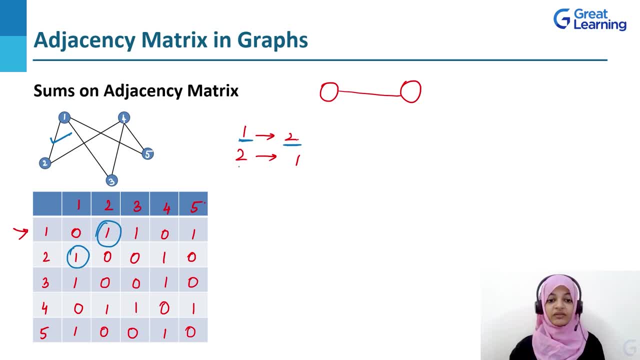 by the 2 idiotic vertices in the left side, where the single vertex circle is Highway 1.. In case we are actually considering the edge between vertex 2 and 1. Since they are undirected in nature, if the edge exists, then it will be counted right. Let us see what happens in a 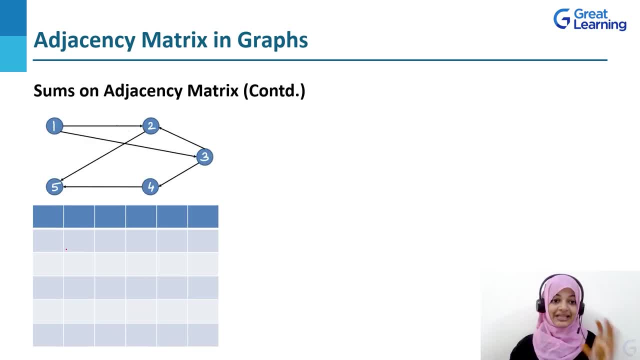 similar case in directed graphs. Consider this particular graph as given Now. as per this particular graph, we will take the required vertices as 1, 2, 3, 4, 5 and 1, 2,, 3, 4, 5.. 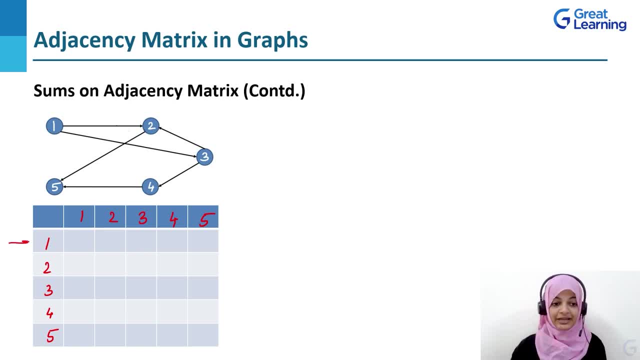 While looking at this graph, we can see that if, considering vertex 1, we have got one edge that moves from vertex 1 to vertex 2, right? Can you see the difference in the way that I am actually talking about it? When we were looking at undirected graphs? 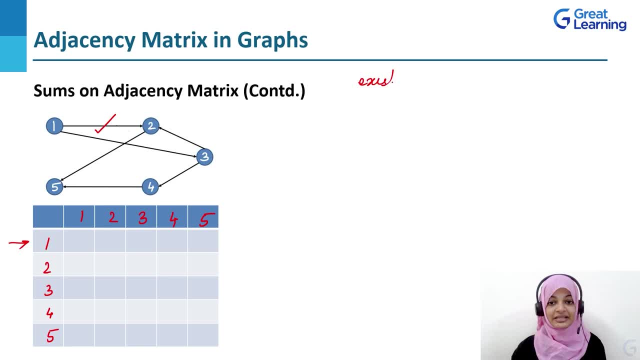 we were just looking at the edge between vertex 1 and vertex 2, right? So we are actually just looking at whether there exists an edge between 1 and 2.. But now what we are saying is, we need to understand, or we need to determine whether there exists an edge, moving from. 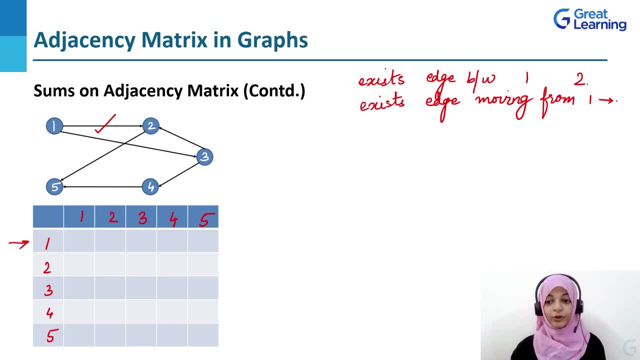 1 to 2.. So here the direction is very important. So, as you can see, here there is an edge between 1 and 2.. So here the direction is very important. So, as you can see, here there is an edge which is moving from 1 to 2, that is vertex 1 to 2.. So we will put up a 1. 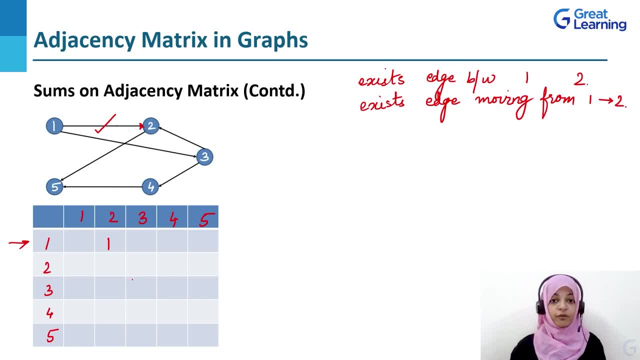 here, Whereas there is no edge that is moving from vertex 1 to itself, So a 0 is put up here. Similarly, if we look at vertex 1, there is an edge moving from vertex 1 to 3.. This means that 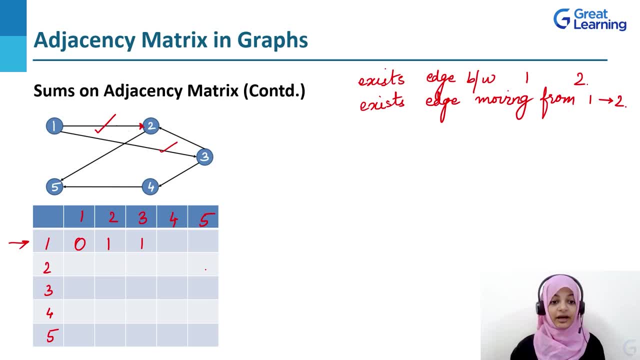 we will have a 1 here. On the other hand, can you see that there are no edges moving from vertex 1 to 4.. So there will be a 0.. Similarly, since there are no edges moving from vertex 1 to 4,. 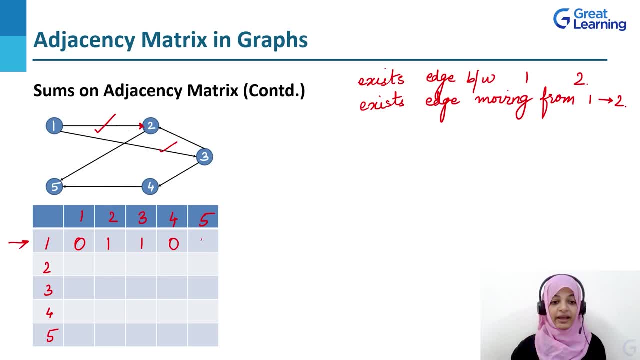 since there are no edges moving from vertex 1 to 5, there will be a 0 here. Next, let's look at the second vertex. If we were talking about undirected graphs, then we would again have a 1 here between the vertex 2 and 1.. But here the way in which we identify edges is: 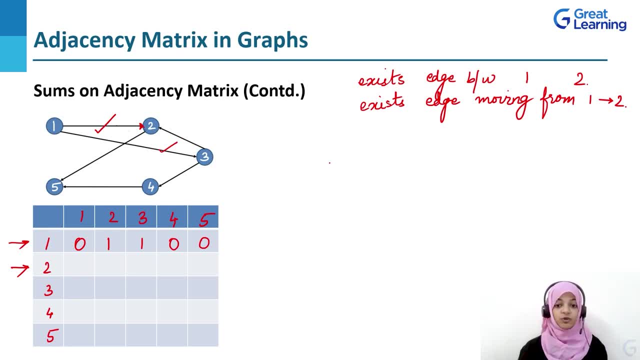 different. We need to check whether an edge moves from the second vertex to the first, Because these are directed graphs, right, As you can see, in this particular graph, we have an edge that is moving from vertex 1 to 2. But we do not have a case wherein the edge is. 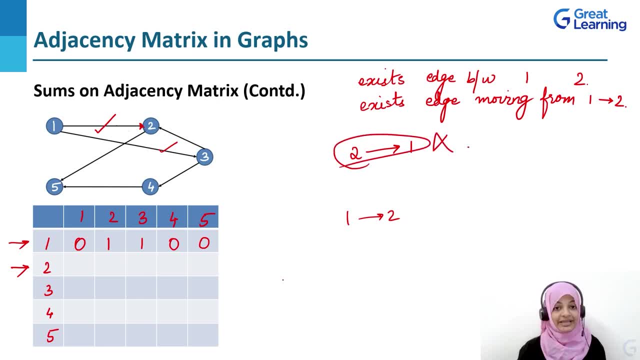 moving from vertex 2 to 1.. So since this does not exist in our graph, we are going to write a 0 here. Similarly, there are no edges moving from vertex 2 to itself. There are no edges moving from vertex 2 to vertex 3.. 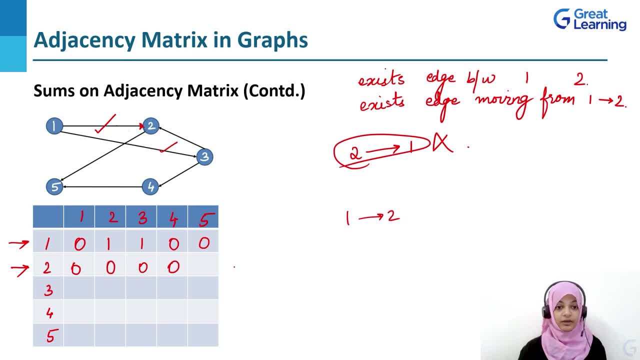 So we are going to write a 0 here. Lastly, there is one edge that moves from vertex 2 to vertex 5.. Thus we get a 1 here. So now let us look at vertex 3.. So, as we can see, here there are no. 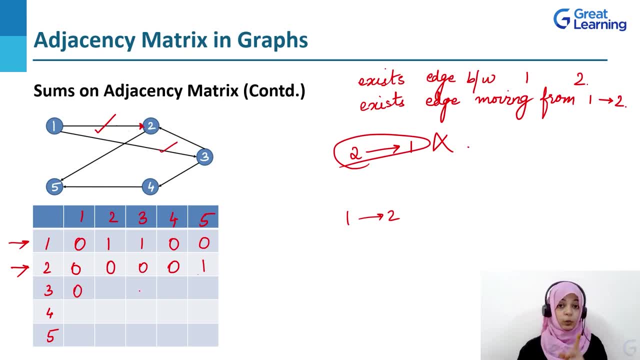 edges moving from vertex 3 to vertex 1.. There is one edge moving from vertex 3 to vertex 2.. There are no edges moving from vertex 3 to itself, One edge moving from vertex 3 to vertex 4.. And zero edges moving from vertex 3 to vertex 5.. Similarly for vertex 4, we have got zero edges. 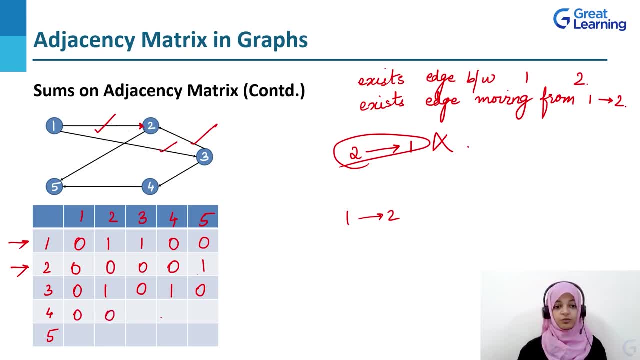 moving from vertex 4 to vertex 1.. Zero edges moving from vertex 4 to vertex 2.. Zero edges moving from vertex 4 to vertex 3.. Zero edges moving from vertex 4 to itself And one edge moving from vertex 4 to vertex 5.. Lastly, looking at vertex 5, we can say that there are zero edges. 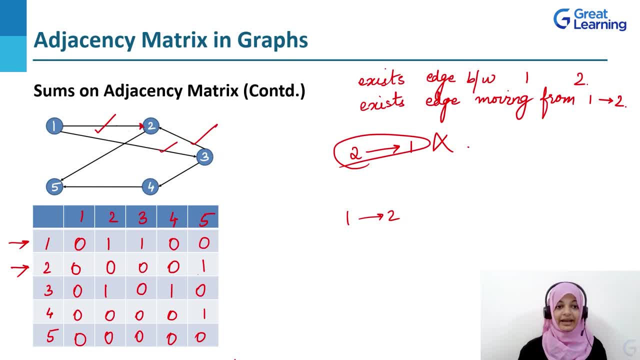 moving from vertex 3 to vertex 5.. So, as we can see here, there are no edges moving from vertex 4 to any other vertex. So this is how we actually have a difference between our directed graphs and undirected graphs when we are looking at adjacency matrices. So let us quickly just 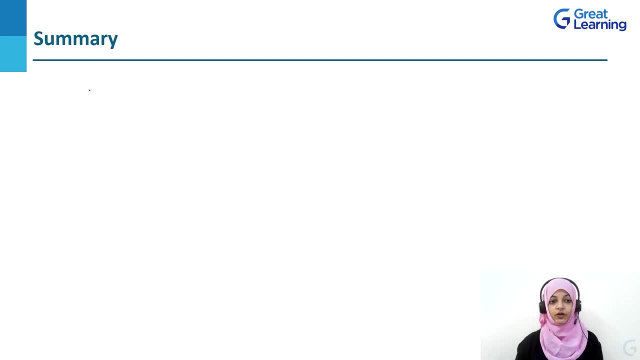 summarize everything that we have seen in this particular course. First, we have seen what graph theory actually is And we have understood why we are using these graphs. So graphs are actually representations of any kind of interaction that goes on between either homogeneous nodes or 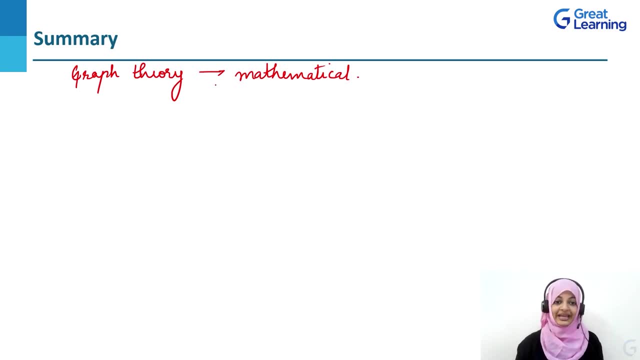 homogeneous points and heterogeneous points or nodes. Next, we also looked at the real life as well as computer science based applications of graph theory. Next, we understood the various components of graph theory, Namely what are edges, What are vertices, What are paths. We also 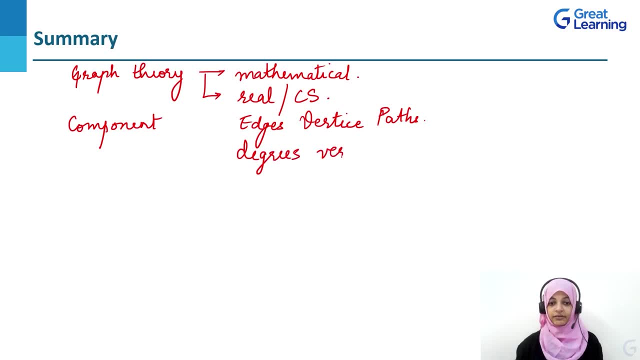 understood what the degrees of both a vertex as well as a graph was. We also understood what our handshaking lemma was and the two interpretations of the handshaking lemma. Next, we saw various types of graphs, namely null graph, simple graph, multigraph, right. All of these different types. 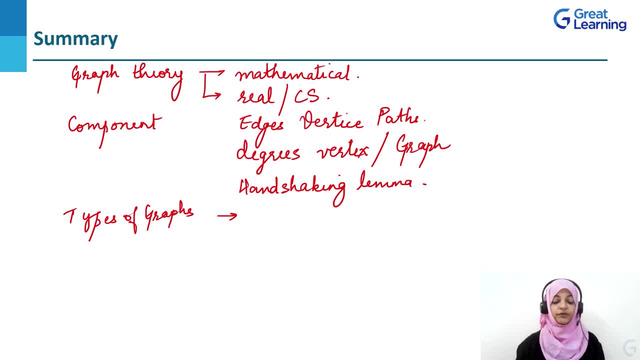 of graphs apart from null, simple and multigraph. So we have understood what the degrees of both are, But instead of the graphs, we have understood all the Olympics. Now let us go back a little bit. as to the features, What is the difference between virtual visco- currencies and the? 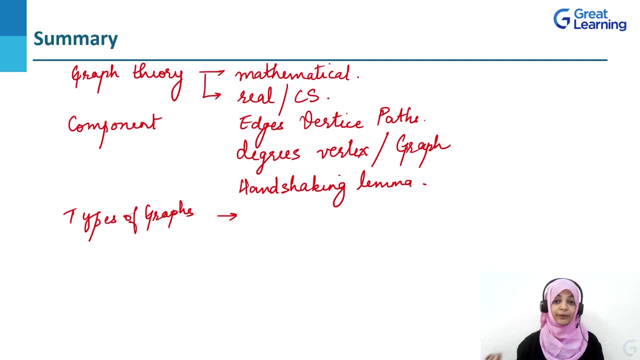 ANDI应ceпов, As between them you can examine the information factors. Agree to our place? Yes, no question, That is correct In the context, quindi, we see that we also saw weighted and unweighted graphs, The characteristics of all the vertical and the un athlete graphs, And we also observed the difference between complete 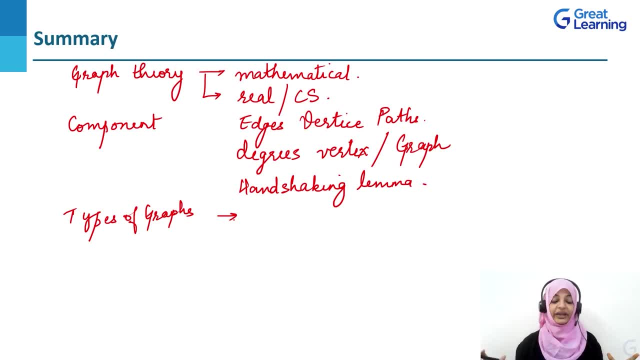 regular, bipartite and complete-partite graphs. In 2016,, we also saw the types of graphs, namely seen can either be directed- undirected in nature, weighted- unweighted in nature, and so on and so forth. realistically, many of the graphs are actually a combination of all of these different 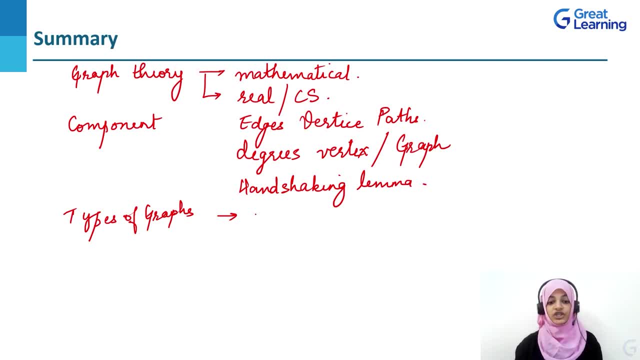 types of graphs. so ideally, we can have a graph which is unweighted but directed, and at the same time, this particular graph could also be a complete graph. so what we've seen is the various types of graphs, and what we've understood now is that it is not necessary that these graphs would. 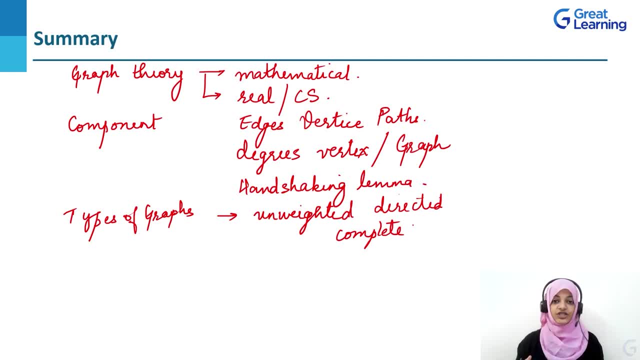 be separate from each other. we could have one graph which is a combination of multiple graphs because it has the characteristics of multiple types of graphs. next we saw the adjacency matrix. what was the adjacency matrix? it was like a map of which edge is being connected to which other edge in a graph. 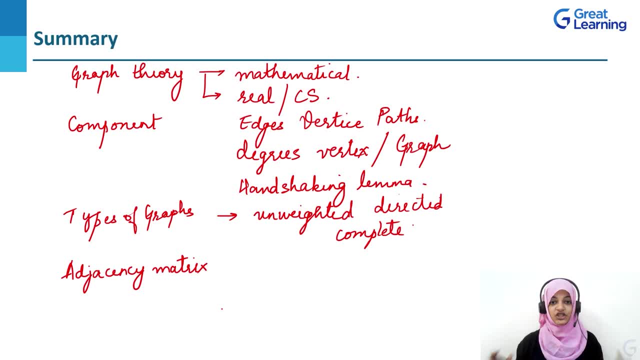 we saw that this particular graph is being connected to which other edge in a graph. this particular map changes its shape and direction as soon as you either put it up for a directed graph or an undirected graph. so one of the basic characteristics, as we observed, was that in an undirected graph, we saw that the row for a vertex would be equal to the column values of that particular vertex. this is because, since this particular edge is not directed, we count it both ways. 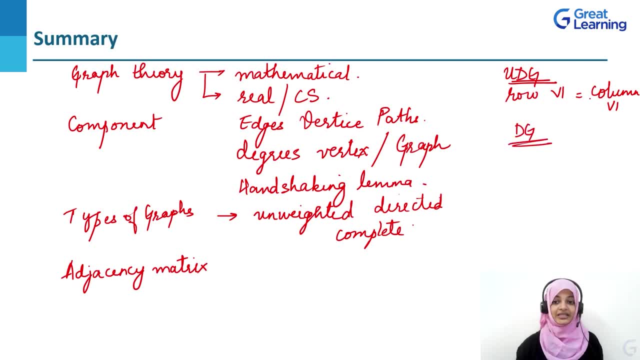 this particular edge is not directed. we count it both ways. on the other hand, in a directed graph, this condition would not hold true, so the row for a vertex would not be equal to the column for a vertex in the graph. on the other hand, in a directed graph, this condition would not hold true, so the row for a vertex would not be equal to the column for a vertex in the graph. 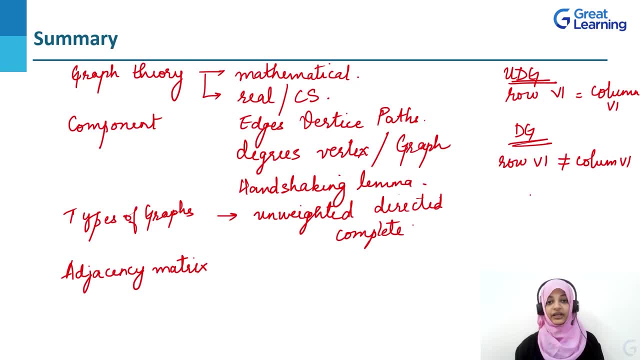 majorly because in directed graphs we are very particular in stating or in understanding that the edge is going from a source vertex to a, refers to wh, имеest to v and it is not necessary that if it goes from vertex 1 to b then there would exist an edge going for another vertex. then it is better to vanillae for this point, because if it is going toなる con vertex b instead of goal review verse secant register vertex would have been machine and queen function. function. function. 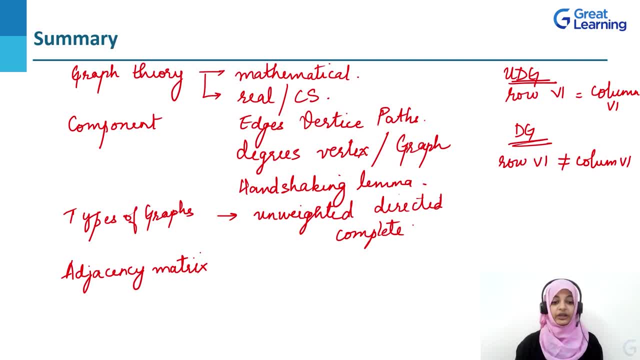 edge going from vertex b to 1. so this is what we need to take care of next. we also saw that adjacency matrices are used in various places where we require shortest distance first, or power grid calculations, etc. right, so we saw two examples of adjacency matrix, also one for our 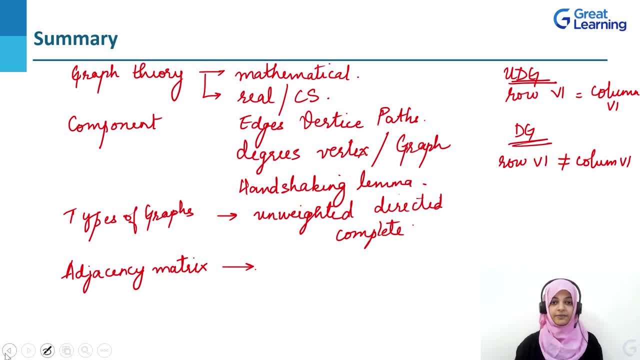 directed graphs and the other for our undirected graphs. so that is it for this particular course, and i hope all of you have understood the concepts given here. thank you so much for attending this course. if you haven't subscribed to our channel yet, i want to request you to hit. 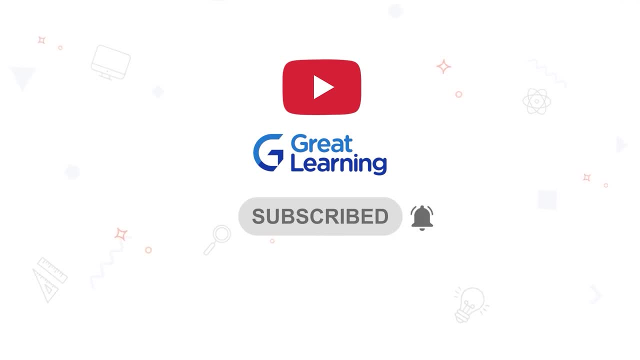 the subscribe button and turn on the notification bell so that you don't miss out on any new update or video releases from great learning. if you enjoy this video, show us some love and like this video. knowledge increases by sharing, so make sure you share this video with your friends and colleagues. 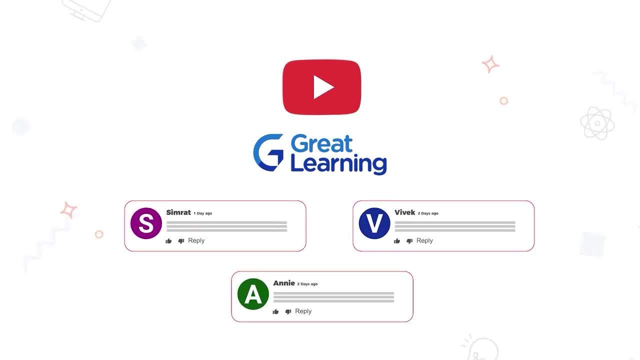 make sure to comment on the video for any query or suggestions and i will see you in the next video. bye, and respond to your comments.